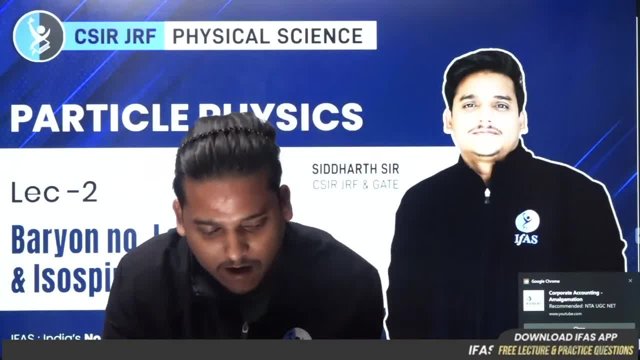 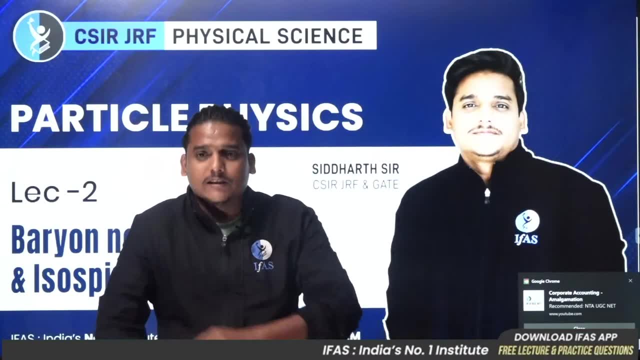 quickly tell me in the comment section what is my voice for. Is it coming to you Quickly? I will also check from my side. Voice is clear, Very good, Perfect, Okay, So quickly join friends. Lecture is going to start. 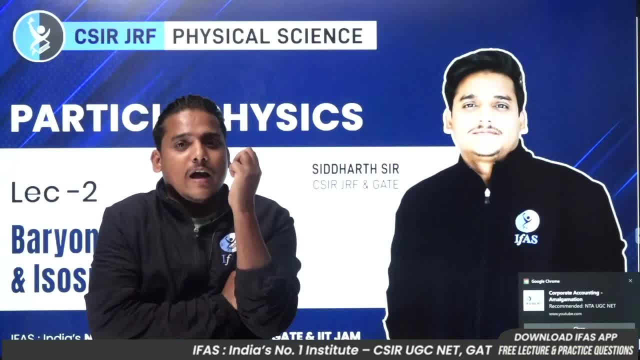 Your according time has been kept. We have joined again. at 8 o'clock Today we are going to do lecture number 2 of particle physics. Okay, So connect maximum students here quickly. Until then, I will talk to the students. 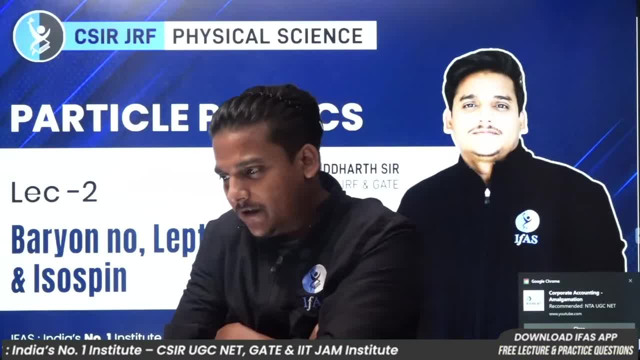 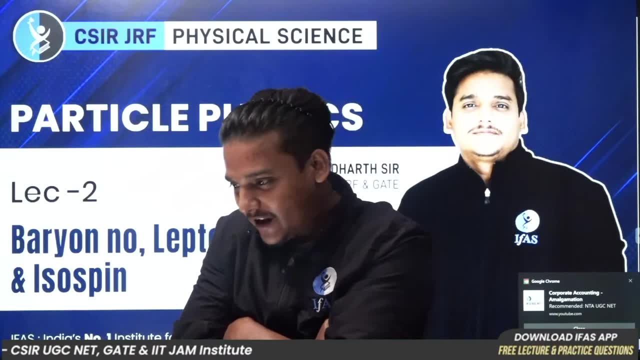 Good evening Abhirup, Good evening Rabia, Good evening Priyanshi. Defense study is saying welcome. Welcome for saying: Tell me too. Good evening Shonika. Hello, Voice is clear. Thank you so much, Abhirup. 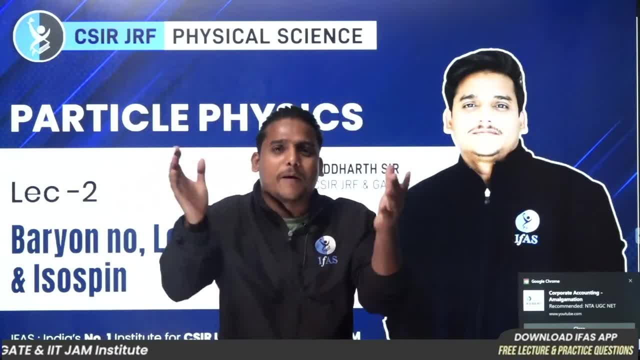 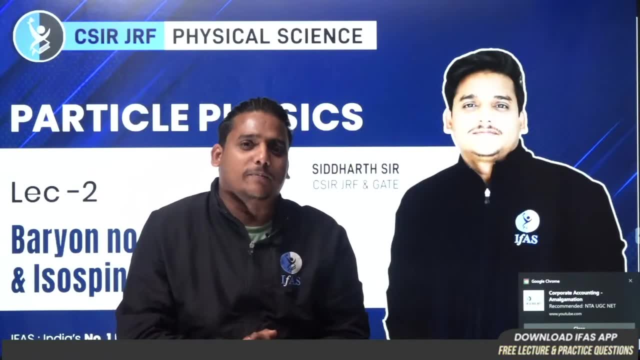 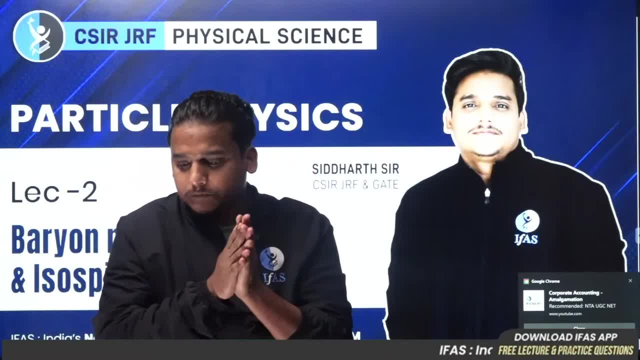 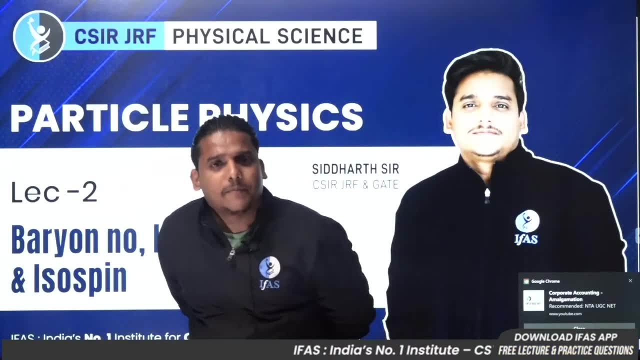 And today I am going to do lecture number 2 of particle physics. So I hope you all must have seen yesterday's lecture. You must have enjoyed it and made notes right. So quickly call your friends here, Share the link of the session and like the session. 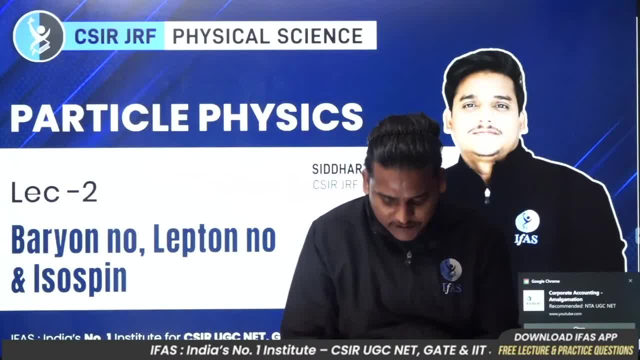 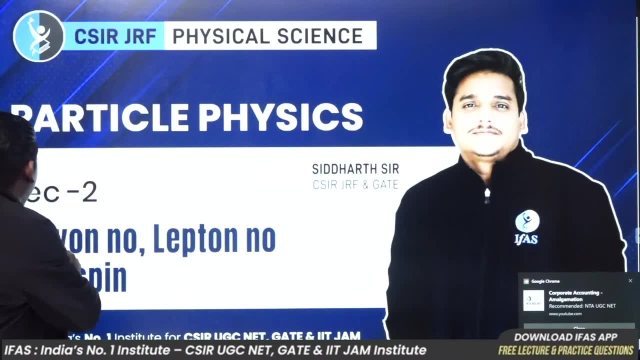 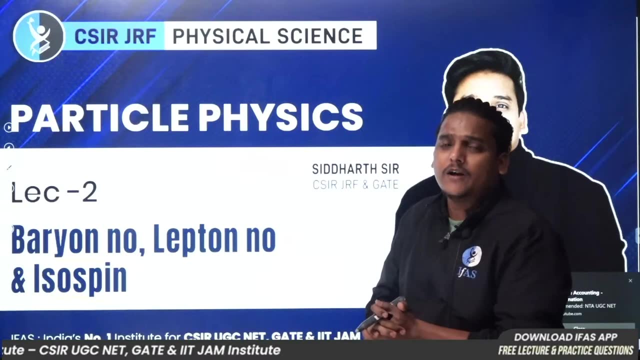 We are going to start, We are going to do batting continuously. The lecture that is going to be today- you can see it on the thumbnail- Today's lecture is going to be on quantum numbers, right, In which, especially the quantum number of iso spin and its third component, we will discuss on it. 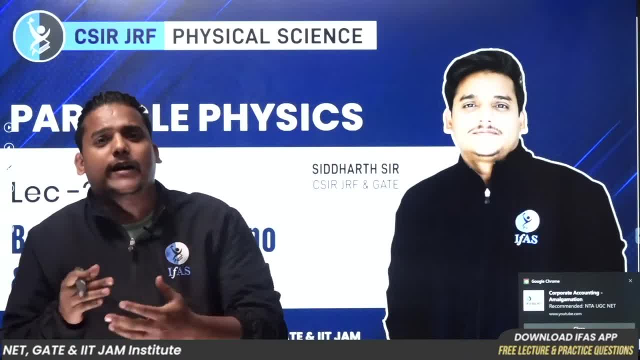 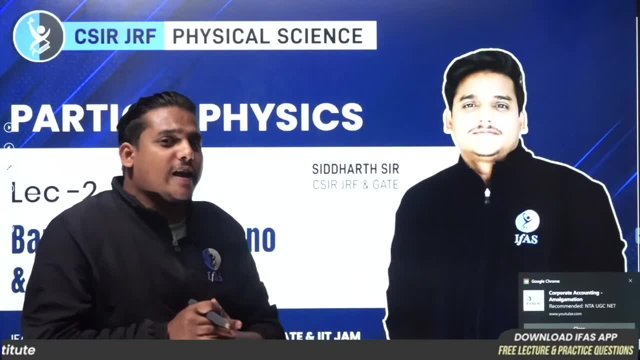 That different parties are going to be there, That different parties are going to be there. How do we take out for these particles- And there is an important lecture You will be need- what is the type of reaction in the reactions? in which interaction is the reaction happening? 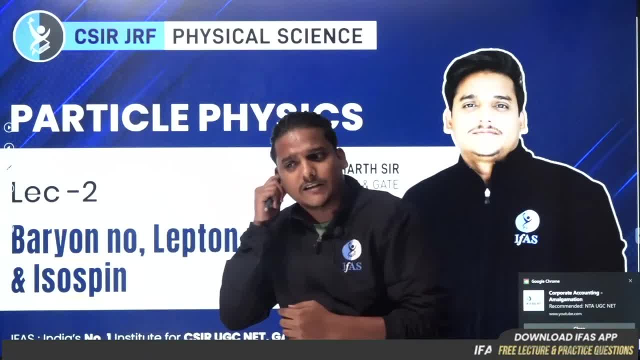 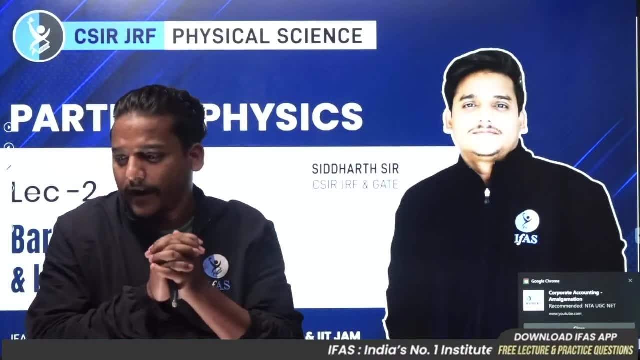 If you want to know this, then you are going to need iso spin. Do you agree with this thing? So quickly? be ready in the comments section Once. tell me that you are ready. Good evening everyone. Good evening, Good evening Bhrushali Gharat. 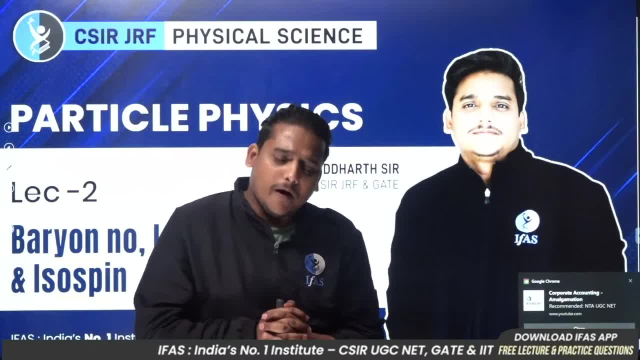 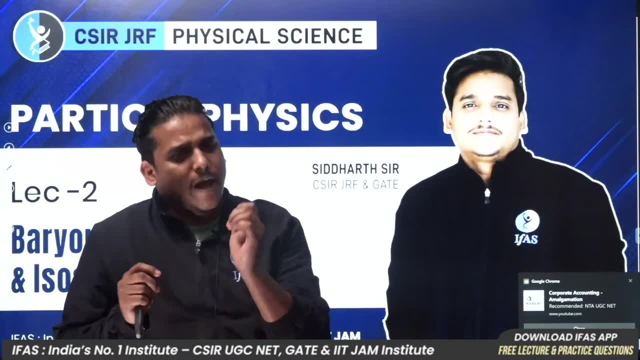 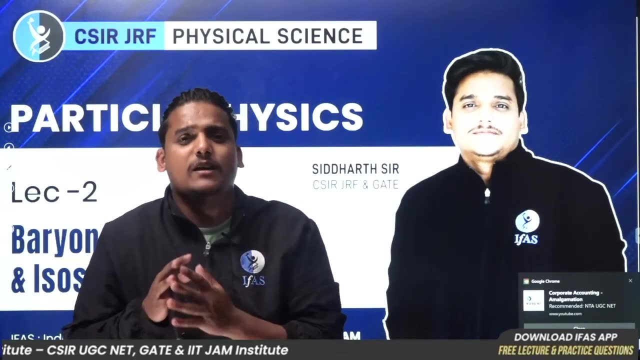 Like the session. All the kids here quickly Like the session and share the session. Your main work is that you have joined here to study. My work is to teach. I will teach well. What you have to do is to do your lecture on whatsapp. whatsapp status insta. 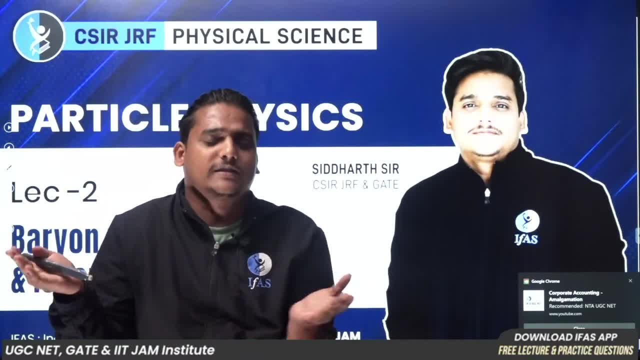 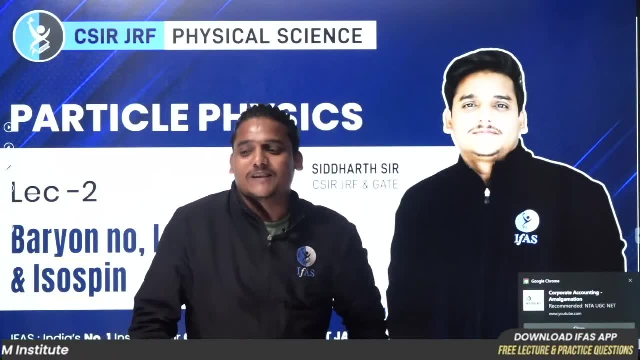 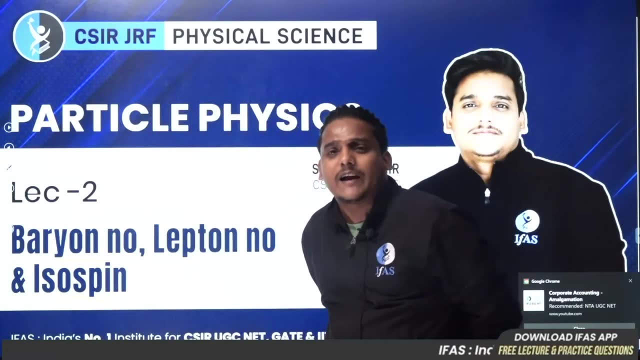 Wherever there are people of your knowledge, who study physics, Who are targeting CSI and net. reach this lecture quickly, Sir. nice hairstyle, thank you so much. potential ji, Thank you so much. let's go. So shall we start the lecture? So students who didn't watch yesterday's lecture go and watch today's lecture after finishing it. 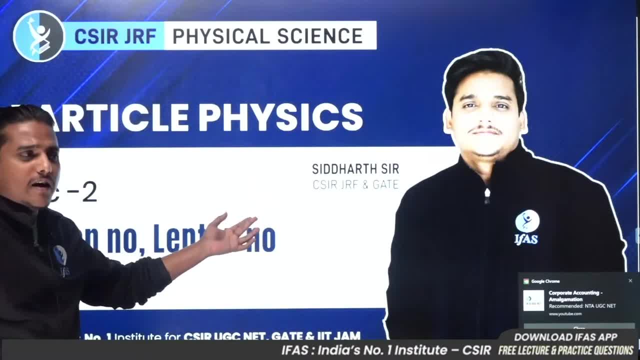 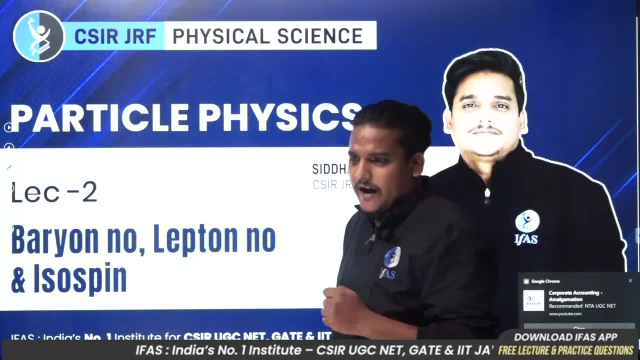 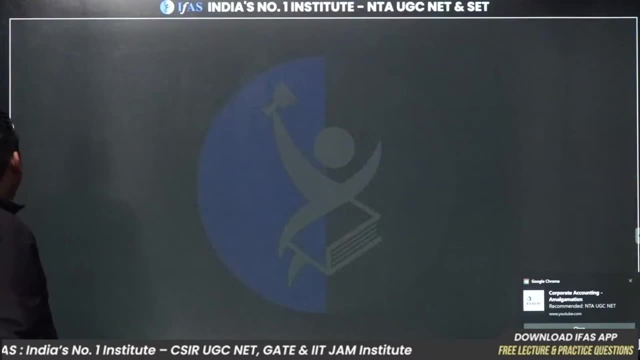 In yesterday's lecture I told you about particles- which are which particles? Which is singlet, which is triplet, And in yesterday's lecture we also discussed about interactions. In yesterday's lecture we also discussed about interactions. Now we will talk about today's lecture and start. 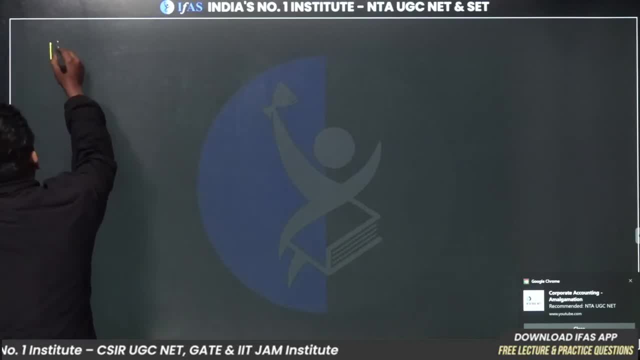 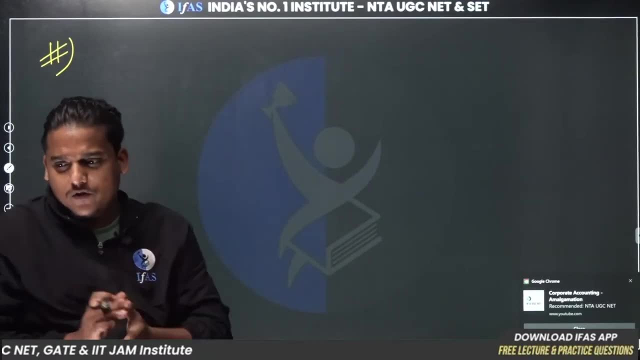 I hope all the students are ready and we have started to do tower toll batting. Keep making notes. Whatever I will teach here is enough for you to do questions on particle physics. I will not let you get worried at all, Sir. Potential ji is our Lalit sir, I know it. Ayesha, I know it. 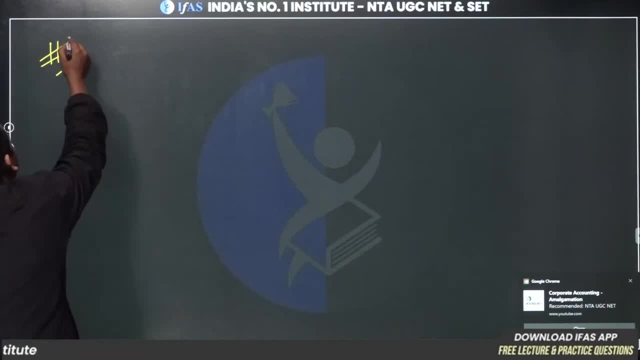 Sir has a lot of potential inside him. that's why sir's name is Potential ji, Isn't it? So let's talk about quantum numbers first. I hope you are ready with the copy and paste quantum numbers Now, students, we have defined particle in particle physics yesterday. that's good sir. 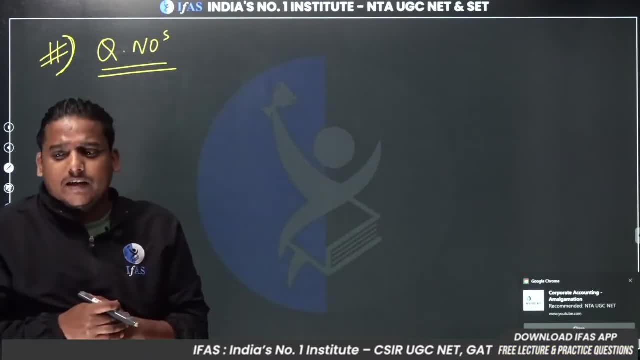 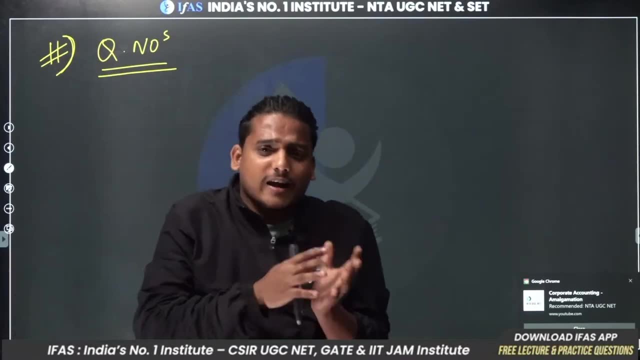 Now you are basically asked: what type of questions are there here that reaction allows? Now you are basically asked: what type of questions are there here that reaction allows? Is this reaction allowed or not? Is it forbidden? These type of questions come to you. If this reaction is allowed, then which interaction is allowed? 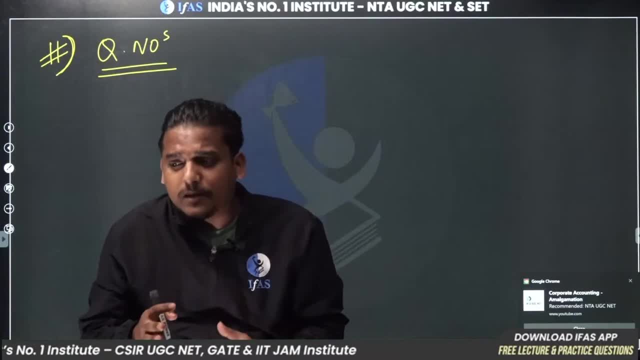 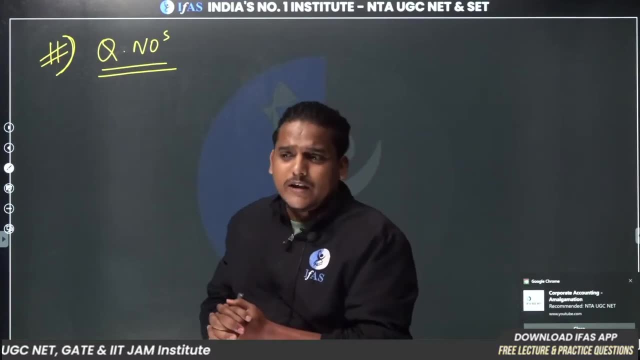 These type of questions come to you. So first of all, we will define some quantum numbers here And understand why this quantum number has been defined. This quantum number has been defined because With the help of this, we can tell The one we will define, isospin now. 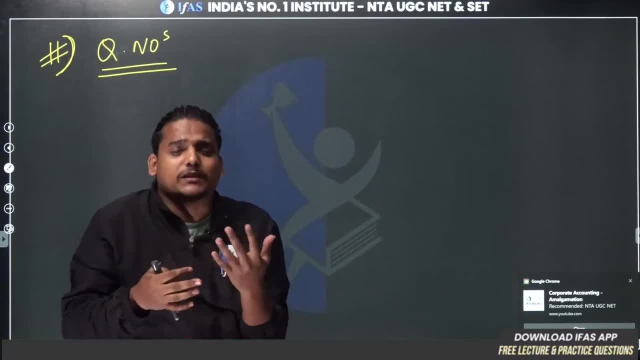 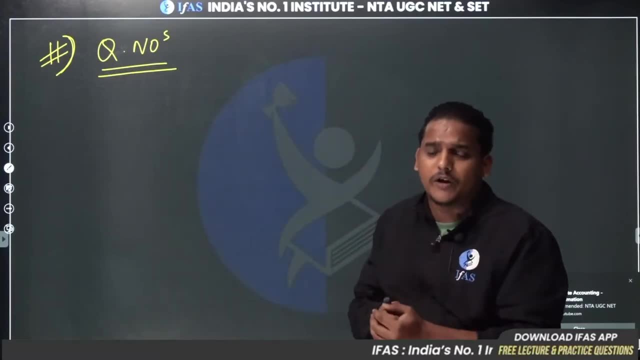 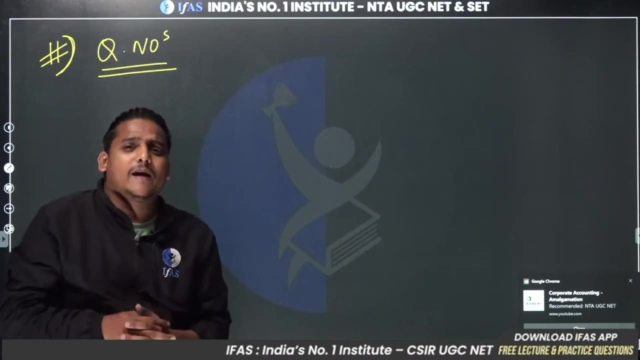 Or Leptonic number or Varonic number. With the help of this, we can tell that reaction is allowed or not, whether the reactions are taking place or not, whether the reaction is allowed or forbidden, Or we can also tell whether the particles in the reaction are existing or not. 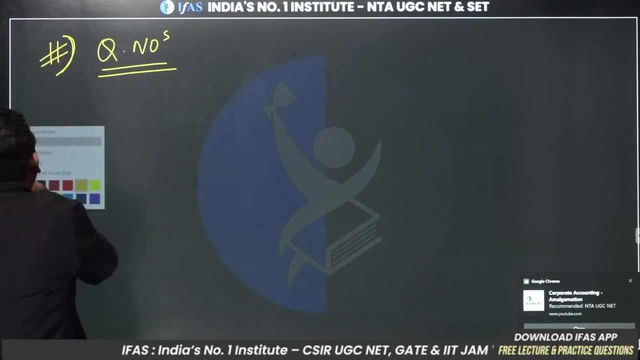 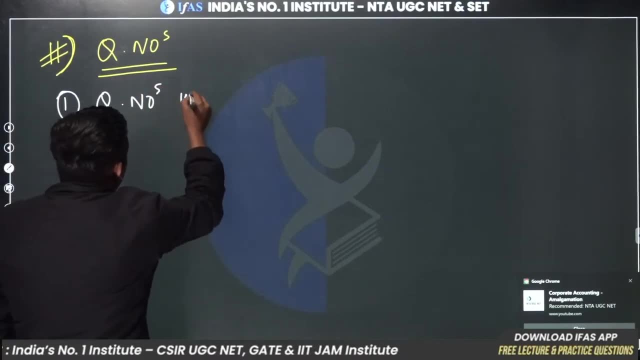 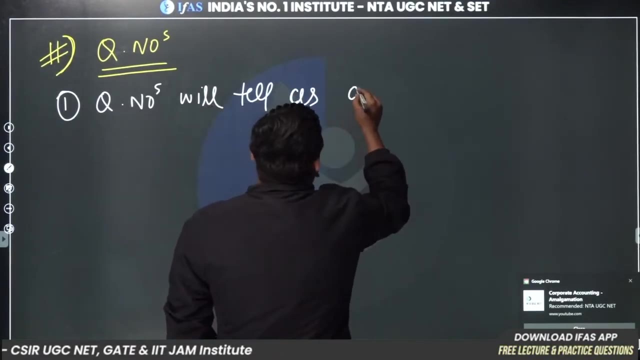 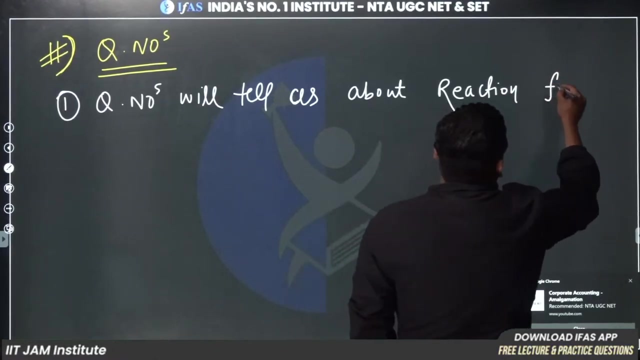 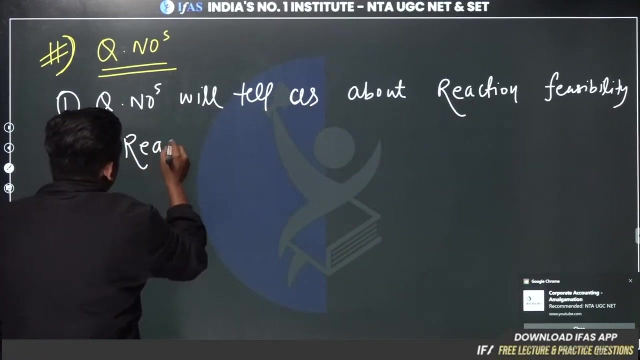 So what information does a quantum number give us? First of all, write it down here At a point. quantum numbers will tell about us. quantum number will tell us about reaction feasibility- Reaction will take place or not. as a little, 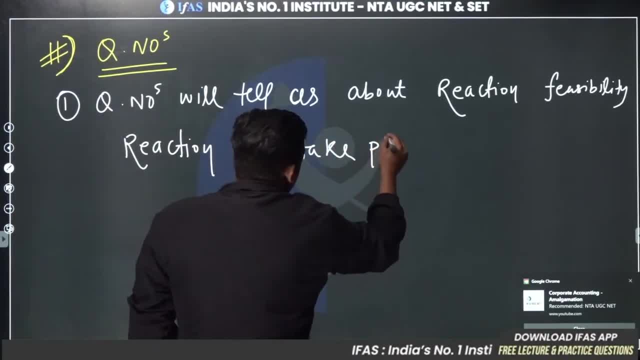 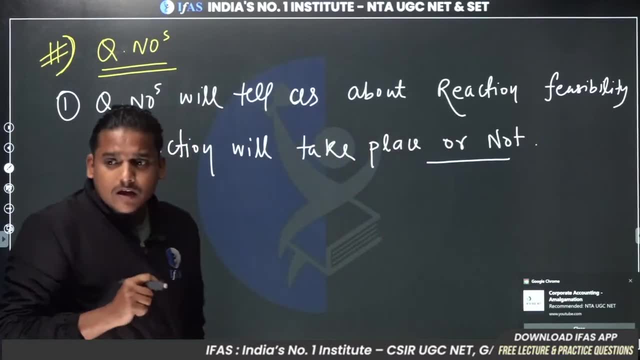 Reaction will take place or not, as a little Reaction will take place or not as a little. Rest of the factors are also there. We will discuss them slowly in each lecture. See, I have divided things in all six lectures, so we will discuss all the things in each lecture. 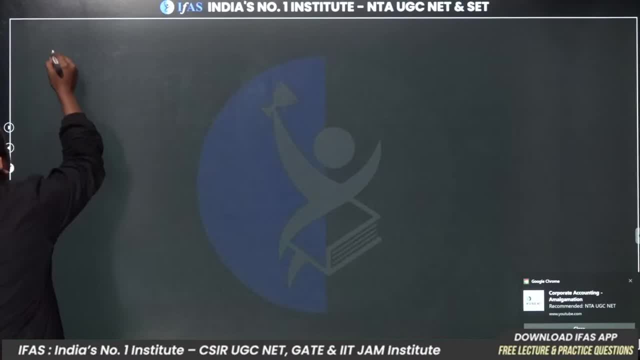 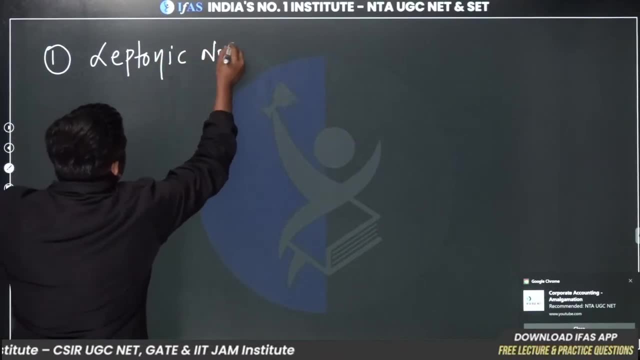 Now I hope everyone has written it First. the first quantum number we will discuss is the leptonic number. right, Tell me if anyone wants the slide at the back. Yesterday we discussed about lepton, that we had lepton particles. 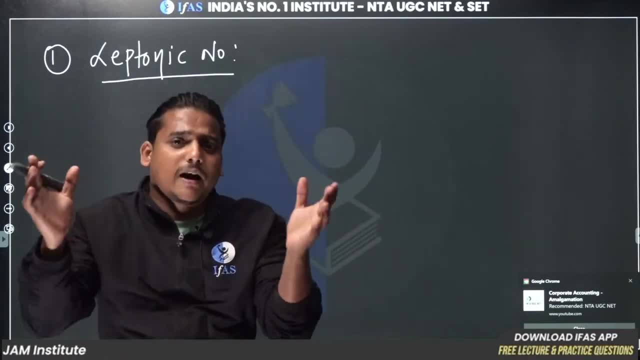 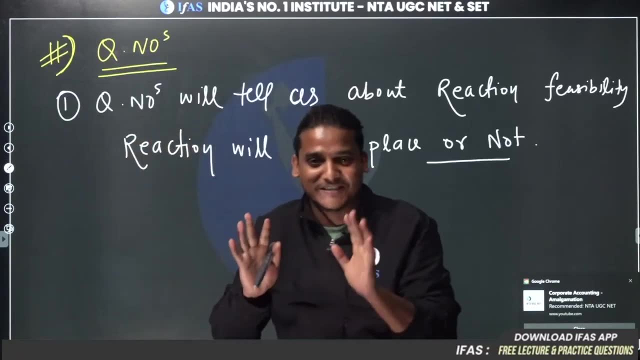 If we look at the total, if we get all the particles, then we had a family of 12 particles in lepton, right, Is it clear? Okay, I could not write, sorry, Sorry, forgive us. So yesterday we talked about the total family of lepton particles, which is 12.. 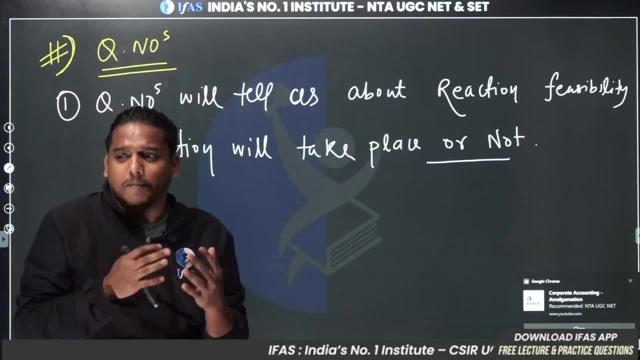 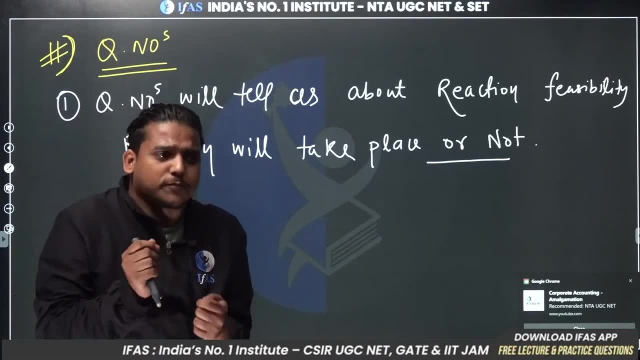 So we are defining a leptonic number here which will tell us- will help us in the future- whether the reaction will take place or not, Reaction will take place or not, And it will also tell us whether some particles are existing or not. right, 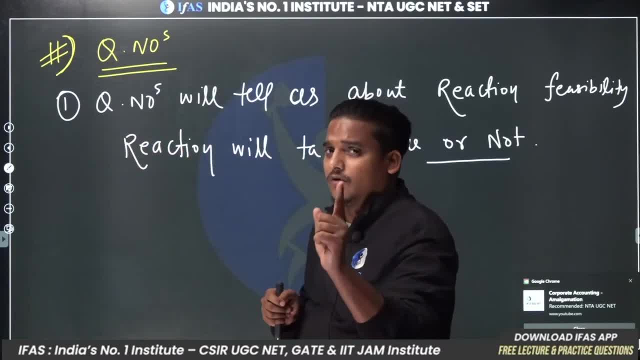 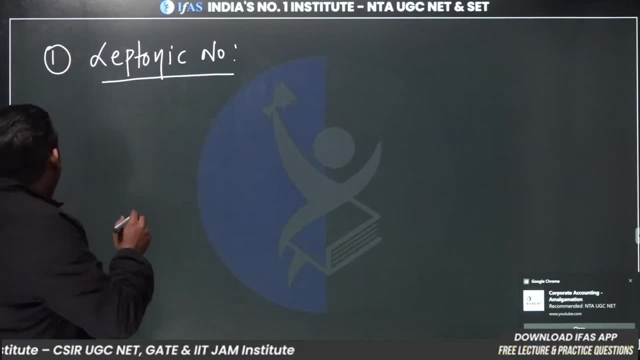 Good evening, Jorah. good evening. Keep sharing the sessions, son. Do not do immorality. do religion quickly. Follow your religion. Now I hope you have written it. So which particles did I tell you yesterday? 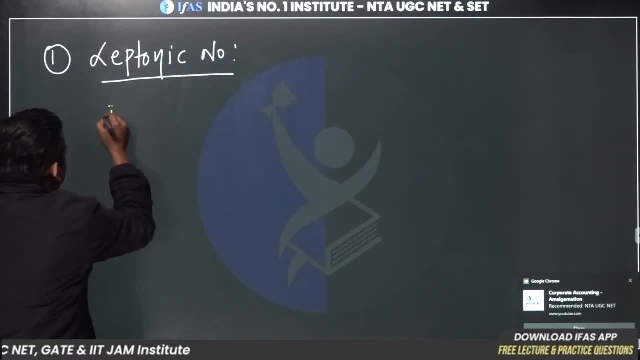 Which particles were there in lepton? We said that the first one is an electron, The second one we said is muon And the third one we said is tau. Okay, We had told all these particles, And then we saw anti-particles. 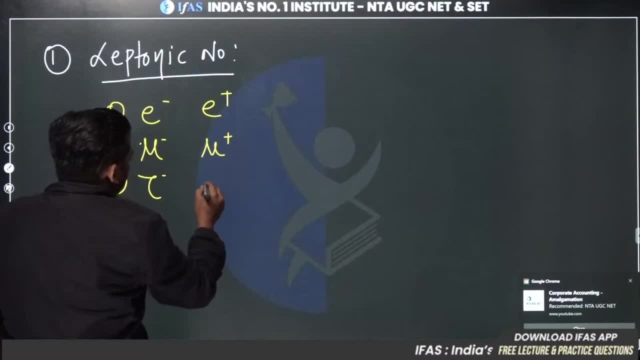 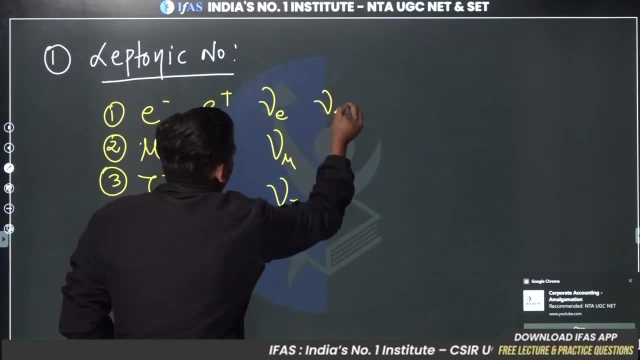 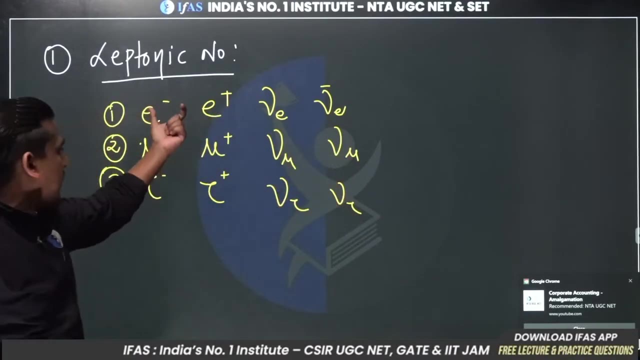 We saw a total of 12 families. We saw its anti-particles, And then we saw its corresponding neutrinos Right, And then its anti-neutrinos. We saw a total of 12 particles yesterday right. So for all these, a quantum number was defined which we called leptonic number. 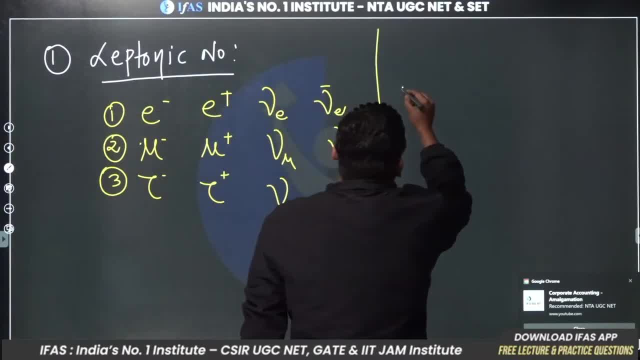 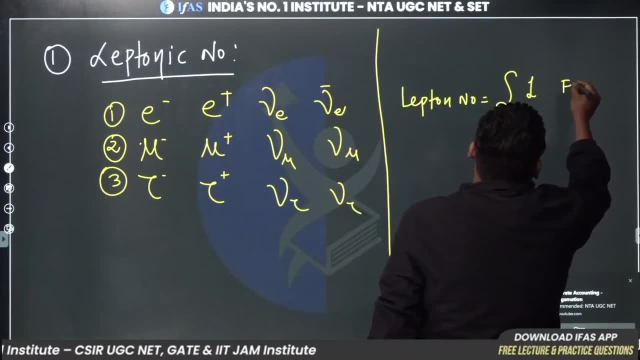 So write it on the side. What is that leptonic number? Write this leptonic number here. Lepton number is equal to 1 for leptons And this will be minus 1 for anti-leptons, Right And otherwise whatever is equal to them. if there is no lepton, then you will choose it as 0.. 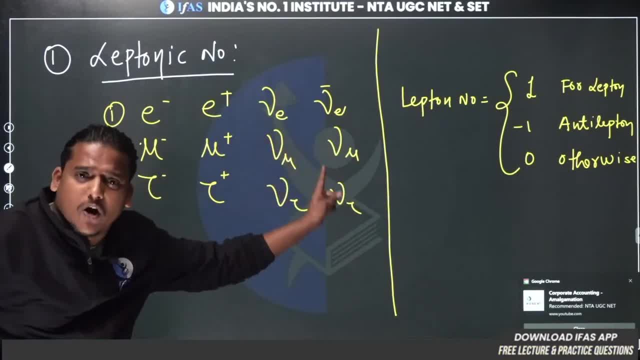 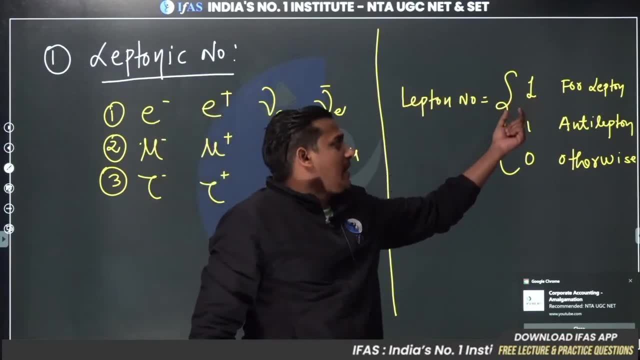 Keep in mind that this lepton number is only defined for leptons. If there is no lepton in any reaction, then there will be no lepton number: 0.. 1 for leptons minus 1 for anti-leptons, otherwise 0.. 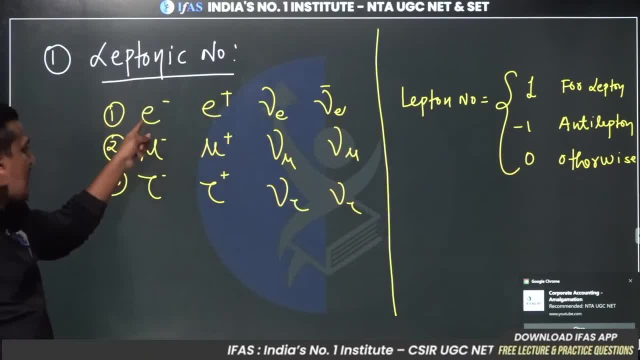 And one thing you also have to keep in mind: that everyone has their own alkyl Right. Everyone has their own different leptonic number. For this you will have LE, for this you will have LMU and for this you will have LTA. 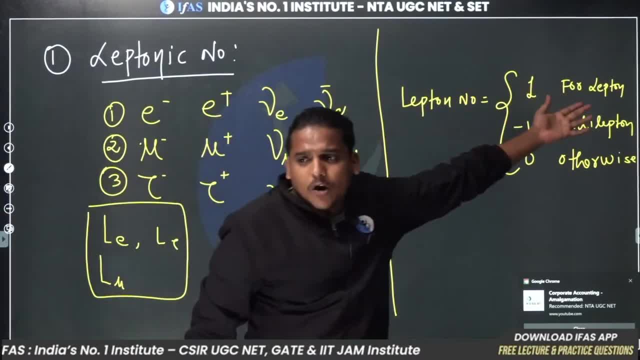 So for everyone, your different leptonic numbers are defined. If it is a lepton particle, then it will be positive for it. If it is an anti-particle, then it will be minus 1 for it. Is it clear, children? 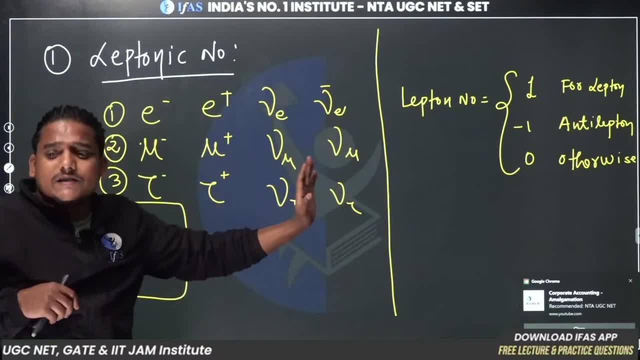 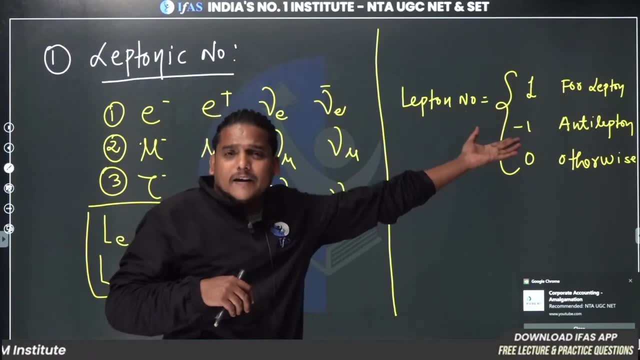 Is it so clear, our dear students? See, you just have to note the basic things. Keep sharing the link of the session. Lepton number is equal to 1 for particle. Lepton particle is minus 1 for anti-particle. 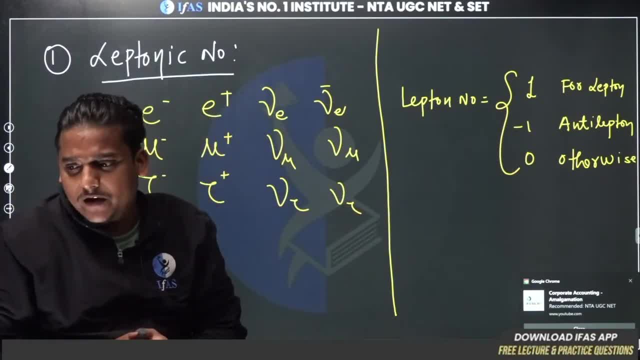 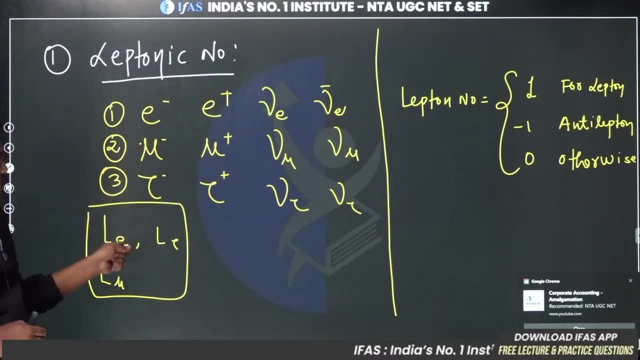 If there is no lepton, then we will take 0.. I hope it is clear. If it is clear, then quickly write this thing and keep in mind For one more lepton. you will see the individual lepton number in the reaction. 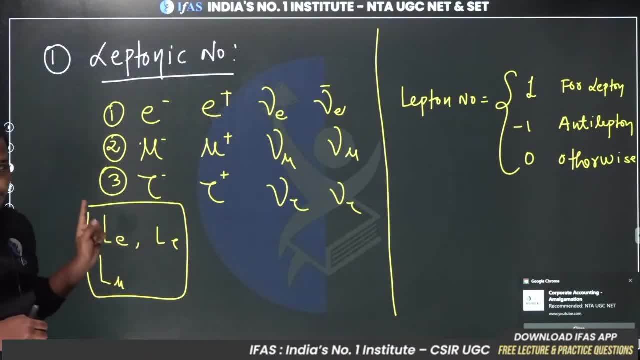 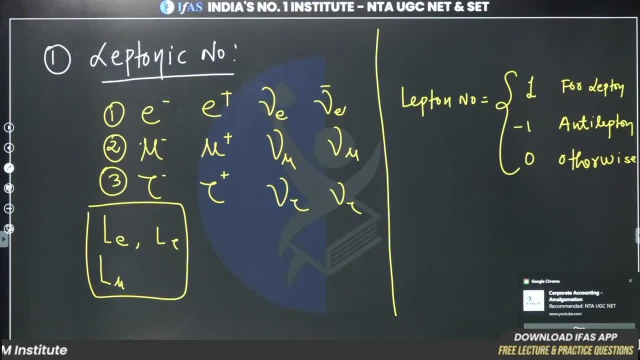 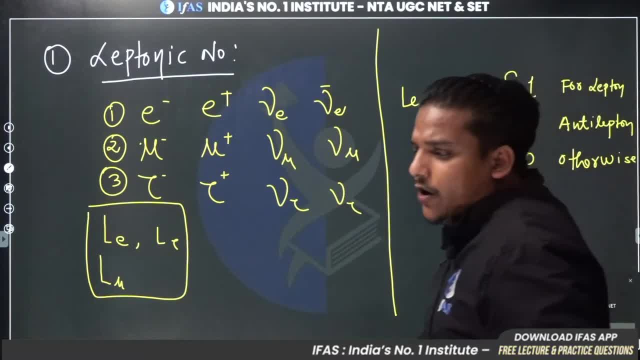 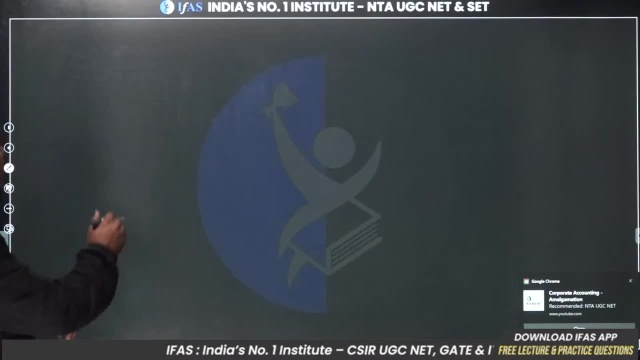 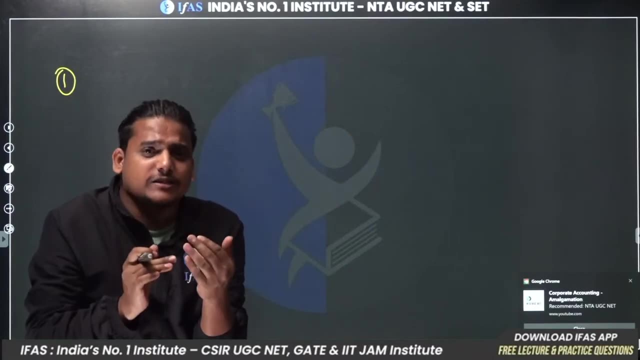 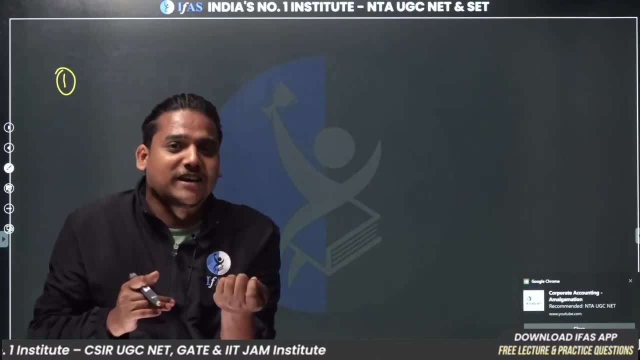 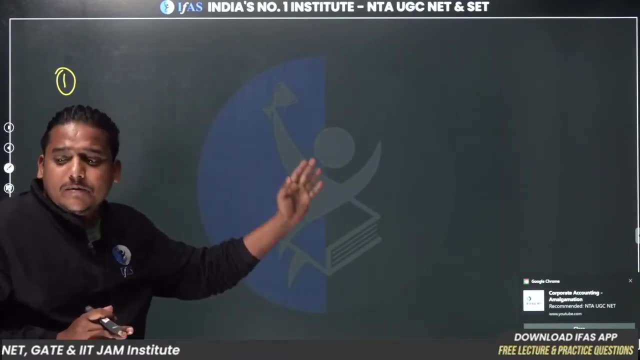 It is not that in any reaction the electronic leptonic number is conserved. but it is not meonic. you will say that the reaction is allowed. No, if you want to conserve the leptonic number then you will have to conserve and check every individual leptonic number. 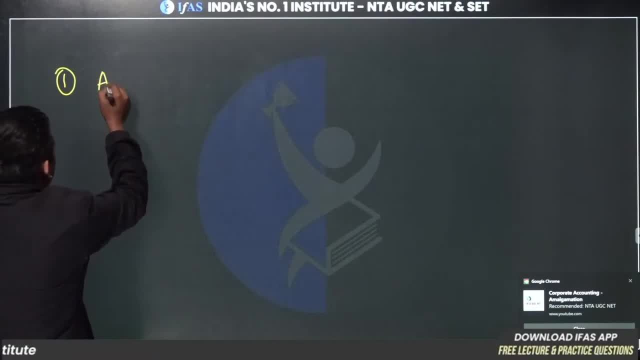 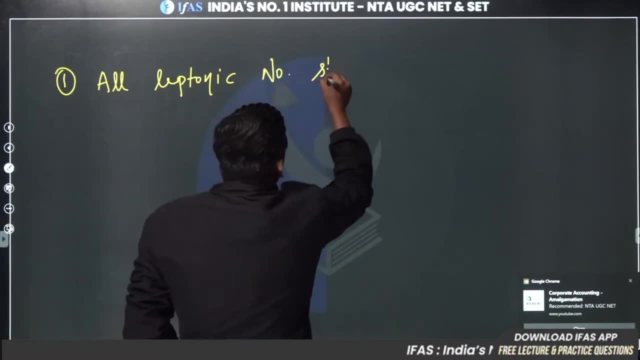 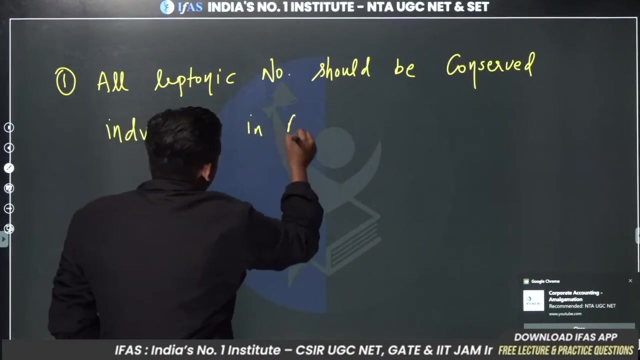 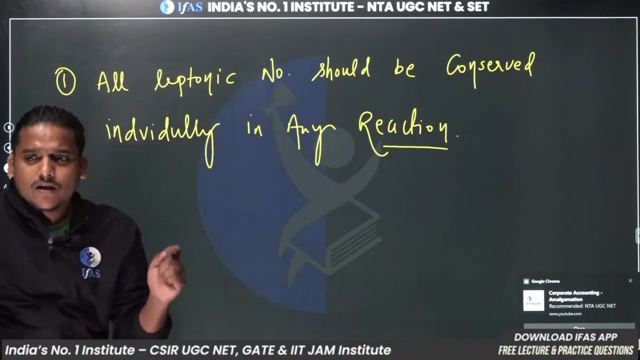 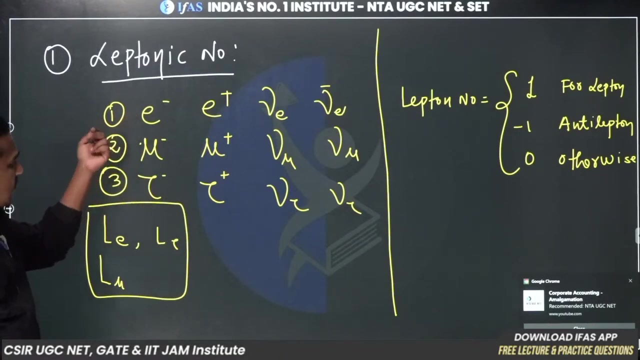 Good evening, Suchita. write here: all leptonic number should be conserved individually in any reaction. Only then that reaction will be allowed. Okay, Okay, If you have any reaction, then in that reaction every individual leptonic number should be conserved, because you have basically three leptonic particles: electron, muon, tau. 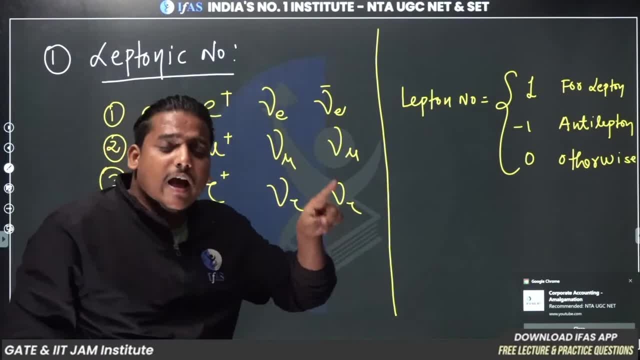 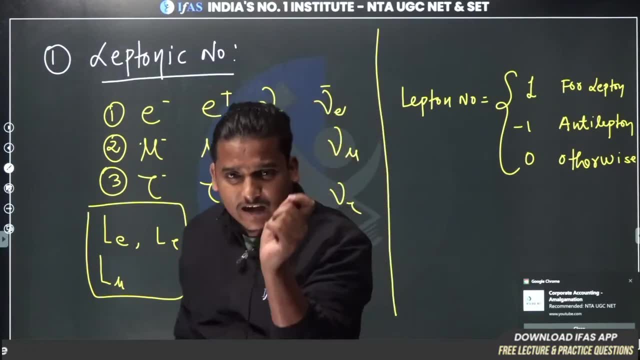 So these three should be conserved individually. If in any reaction electron is also present, muon is also present, then you have to check the electronic leptonic number as well. Is it conserved? LHS and RHS are on both sides, And then you have to check the meonic leptonic number as well. is it conserved or not conserved? 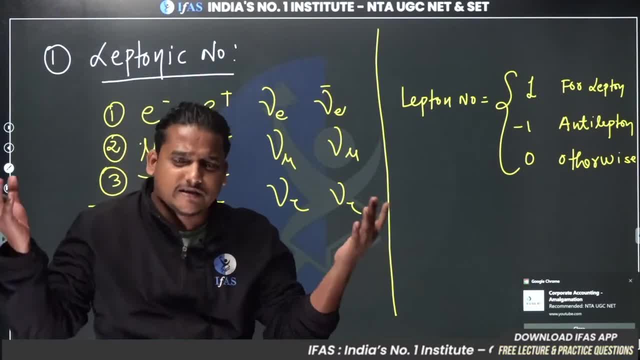 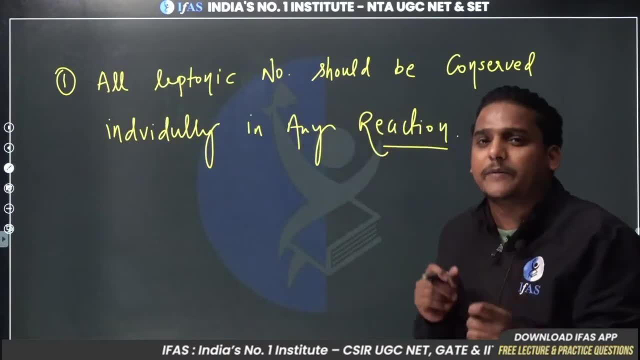 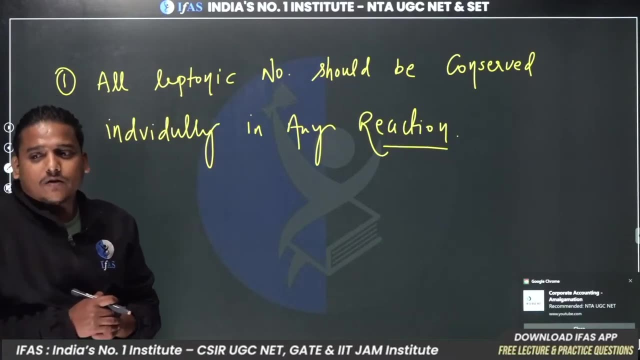 If none of them are conserved, that means reaction is not allowed Easy. So this statement is very important. write it quickly: All leptonic number should be conserved individually in any reaction. Any reaction should have leptonic number conserved individually. Keep liking the session and keep sharing the session. 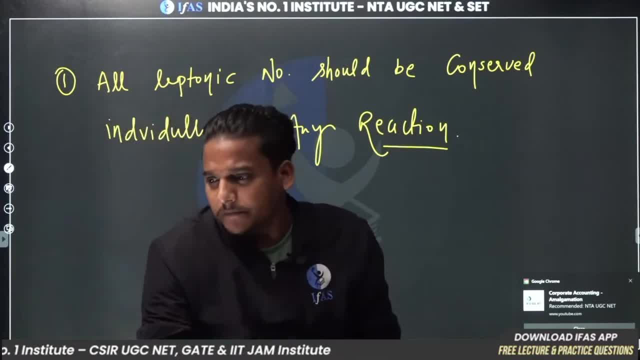 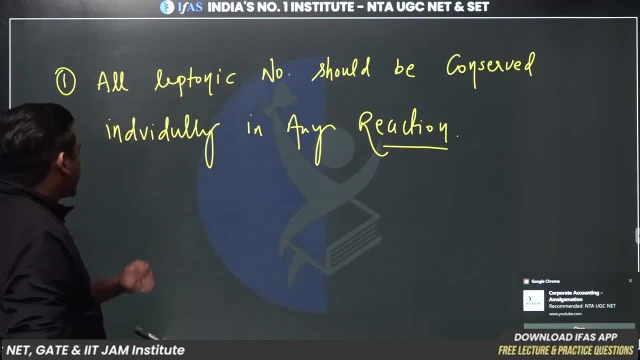 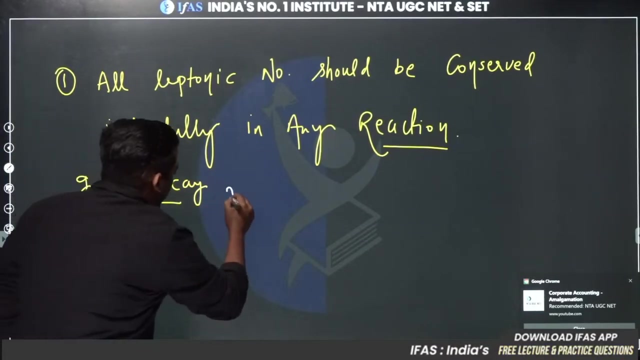 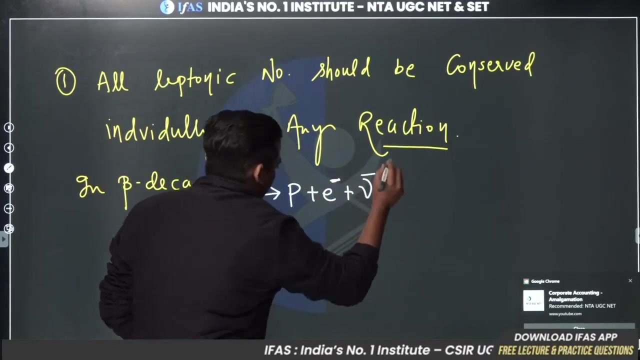 I hope you have written it clearly. Is it clear? Okay, Let's understand it as an example. How, sir, Like I told you about beta decay yesterday, Right, I told you about beta decay yesterday. yesterday, I told you about a beta decay. what do we see in beta decay? we see in beta decay that my neutron is being converted into a proton and along with that electron, and here antineutron is coming out. sorry, here, yes, antineutron is coming out. you know this, but how will we be able to find out which particle is coming out with the help of this concept? suppose I have. 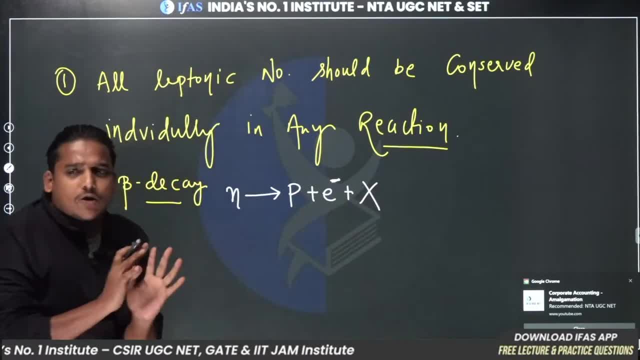 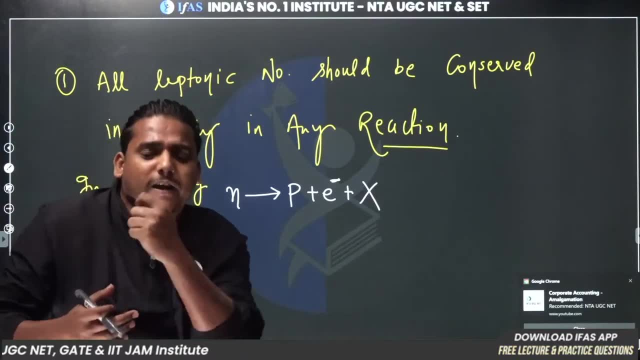 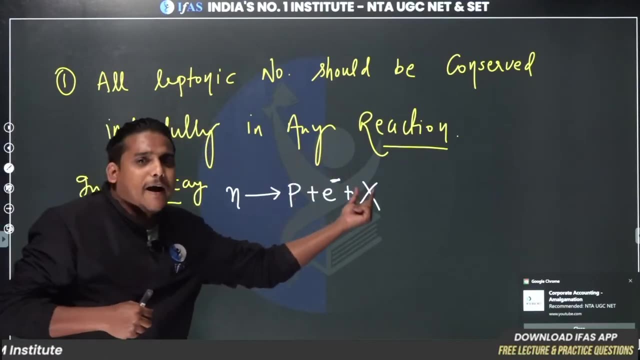 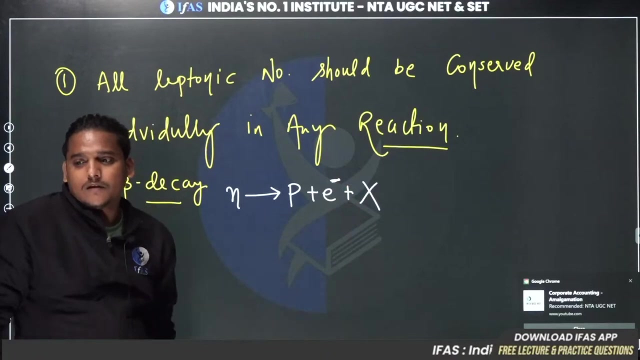 put some x here. suppose, for example, you know that antineutron is coming out here. you know, but let's apply this concept. how will we be able to find out with the help of this concept, if both are concerned, then only conservation is exactly. how will we be able to find out from this concept that actually this particle is x? put the concept of leptonic number. you will be able to find out by default that this x is antineutron. put the concept. 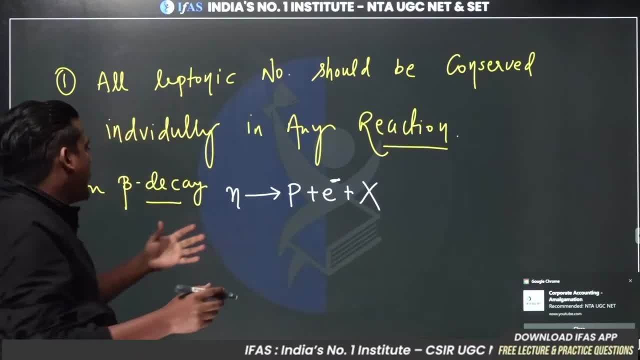 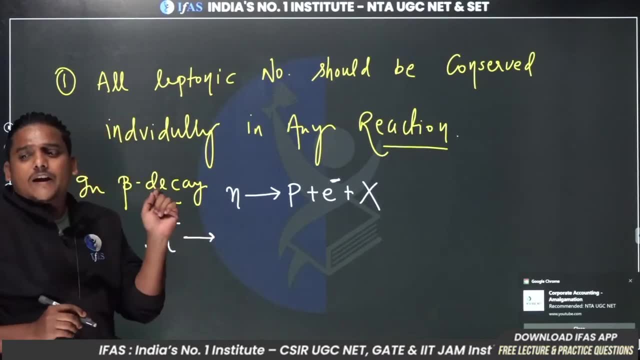 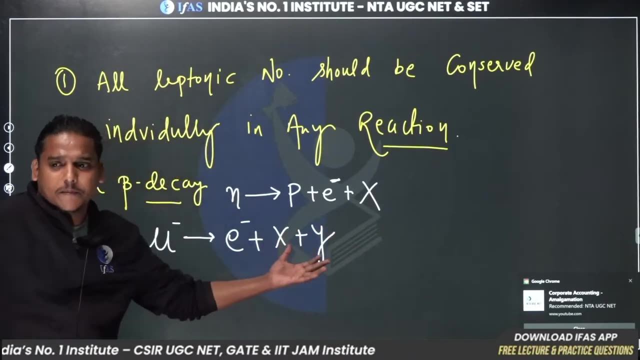 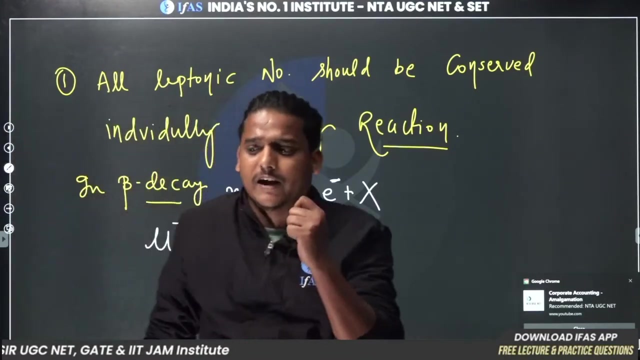 or leave it here. I will give one more reaction. put it in this, as I said, one reaction mu minus gives us. if I give you a reaction, mu minus gives us electron plus x plus y. for example, I gave this reaction. right now you tell me what is x and y here. how will you find out? see, from the concept of lepton number you will be able to easily find out what is x and y. there is a reaction mu minus, which is electron plus x plus y. 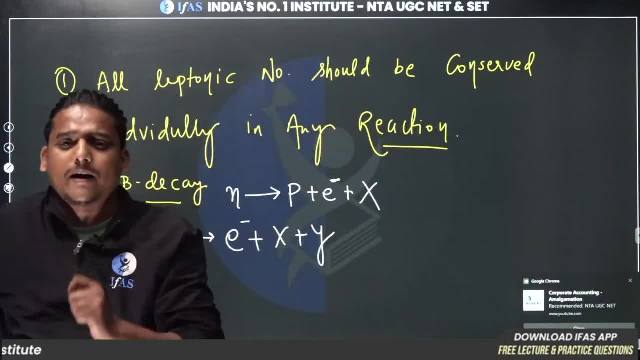 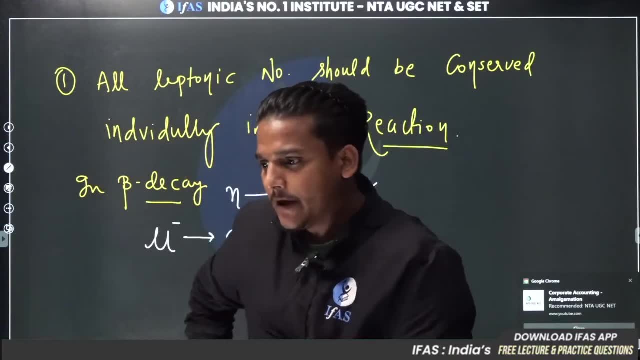 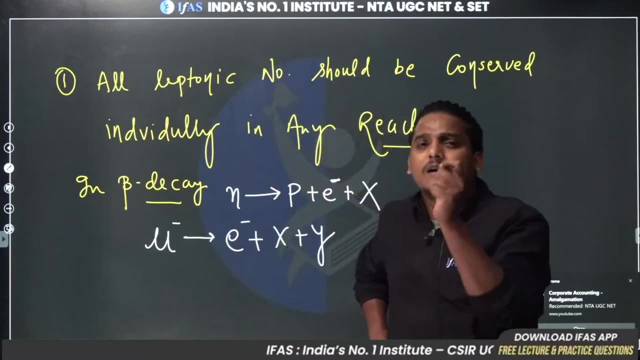 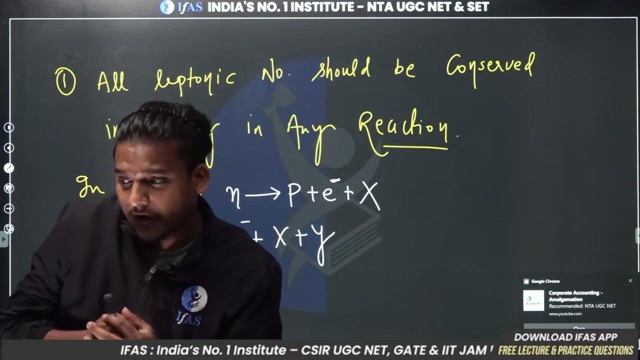 you have to find out that. what is the x particle unknown and what is the y particle unknown? tell me quickly in the comment section anyone like the section. we will choose both then exactly, I need an answer in the comment section. whether it is wrong or right, it doesn't matter. you try here: x and y. what is going to happen to me? x is a neutrino. where is the neutrino? muon, electron or tau? which neutrino? this is a neutrino. 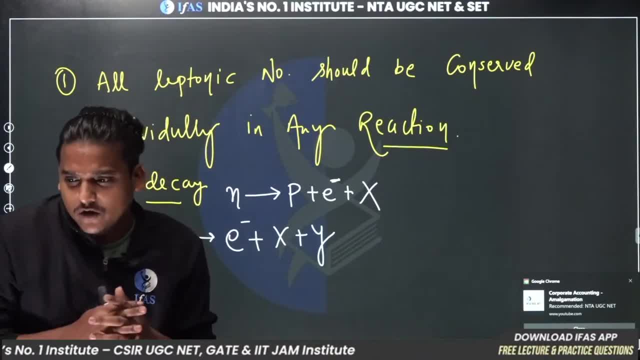 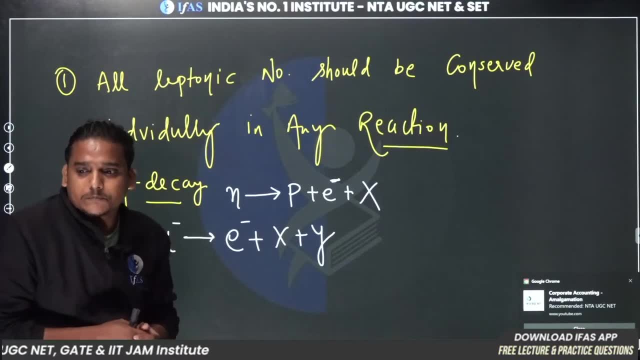 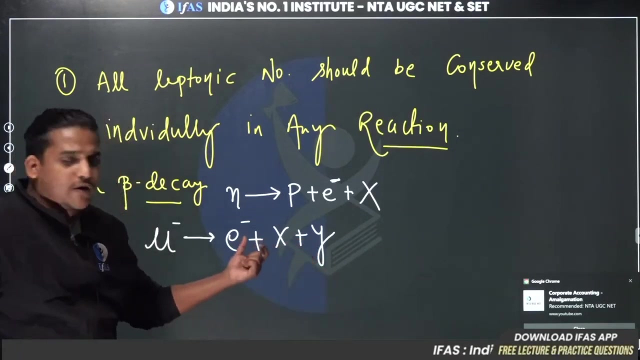 tell me x here. tau neutrino, ok, tau neutrino, ok, neutrino will be, sir, first, which neutrino will be which? tau neutrino, muon neutrino? what will happen, sir, by anti-neutrino- very good, correct, very good, perfect. by what you are saying, sir. anti-neutrino of electron, very good, electron anti-neutrino and muon anti-neutrino, very good, perfect. now see how you can do this. now think about one thing. 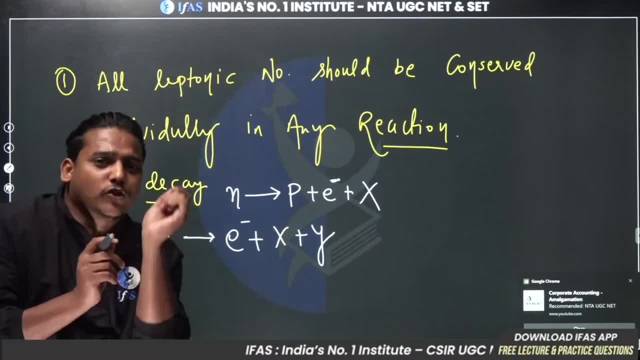 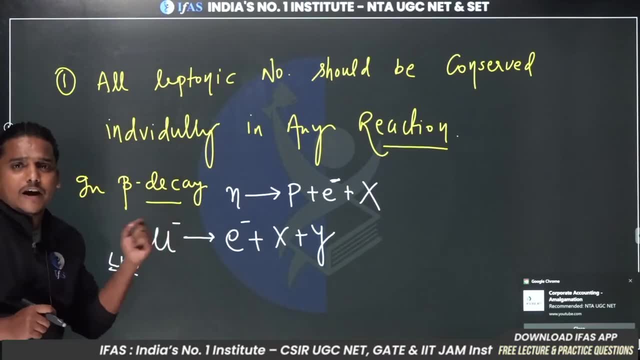 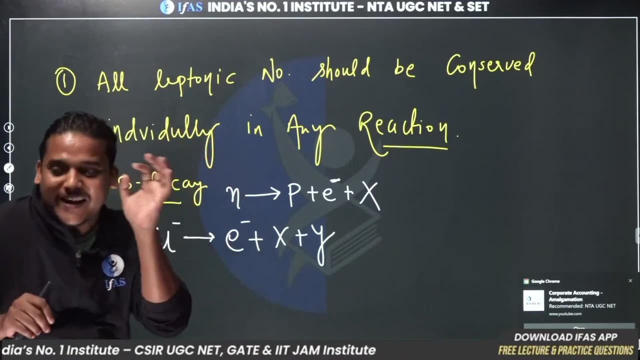 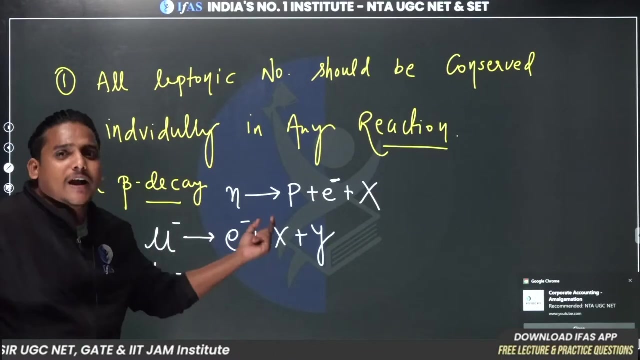 in the left hand side. I said every electron number should be considered individually. I will check individually. first of all, I check in this electron electronic electron number. there is no electronic electron number in my left hand side right. there is no electronic electron number in my left hand side. if there is no electronic electron number in my left hand side- there is zero- then there should be zero electronic electron number in my right hand side. is it clear, children? 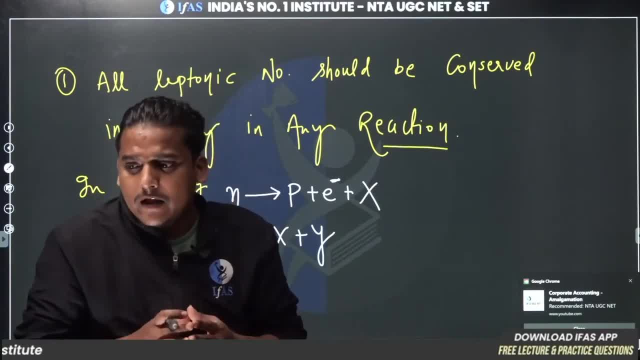 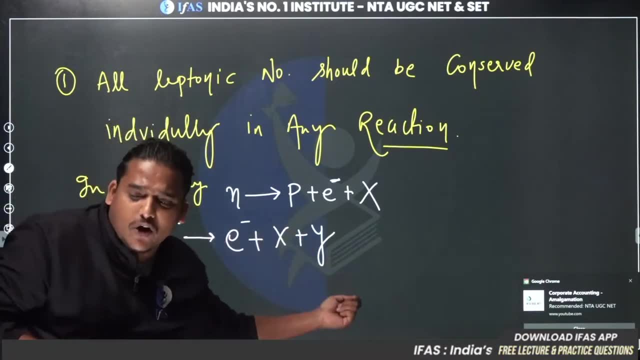 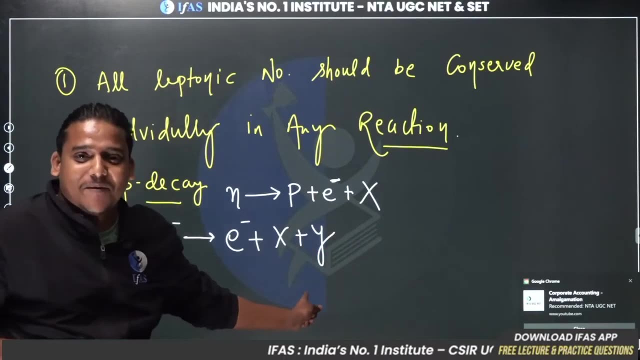 you are getting a feel from internet and you are getting the concept clear. if in my left hand side there is no electronic laptop number, that means in my right hand side electronic laptop number should be zero. but here it is, there for this beta 1, so here it should be of minus 1, then only it will be zero. 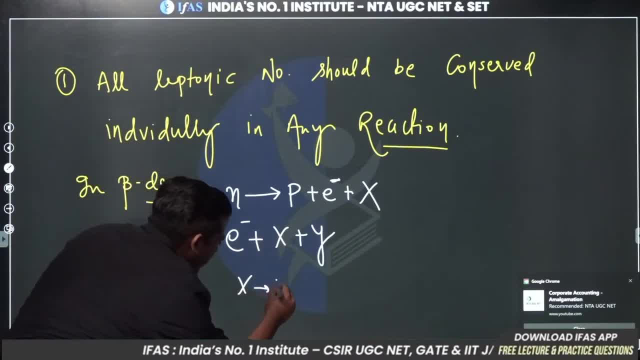 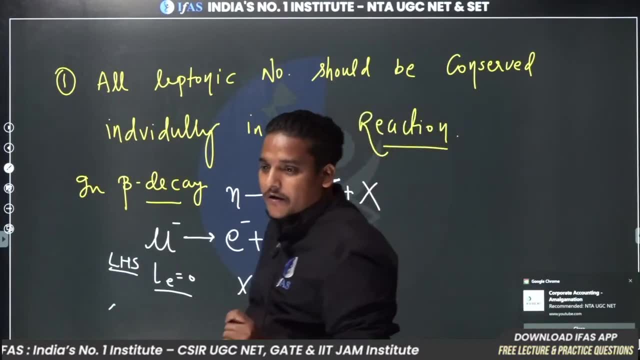 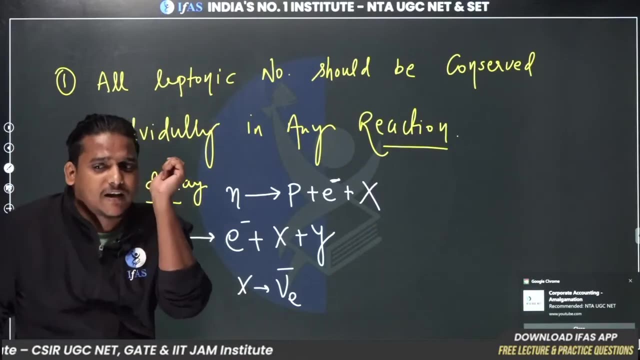 so to get minus 1, this x should be. this is it perfect? it will be shining now. now suppose here I said individually we will check individually. all electronic numbers should be conserved in my reaction. now here my l mu is 1 because it is muon particle. 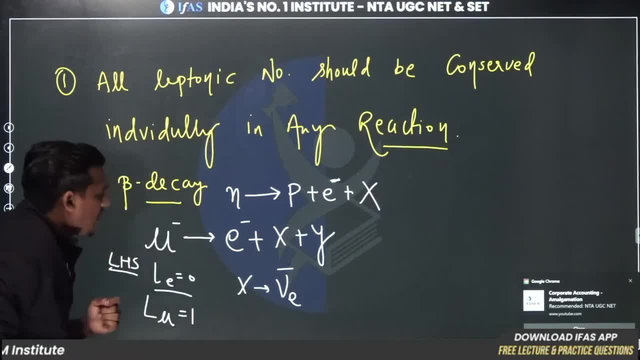 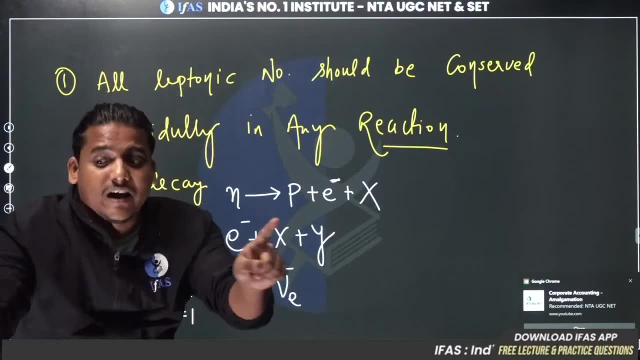 so here in my left hand side l mu is 1. now I want 1 in my right hand side. then only my muonic laptop number will be conserved, otherwise reaction will not be allowed. and I told you by default that this reaction is allowed. so what will come here? 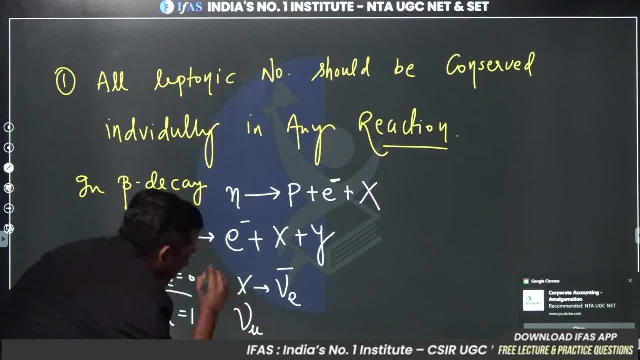 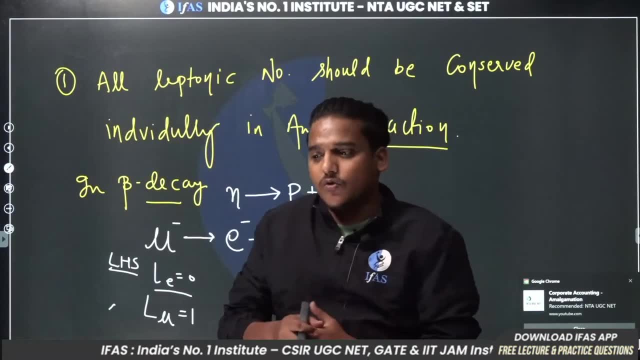 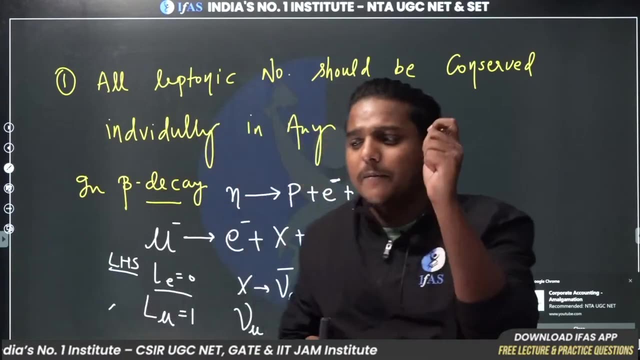 here will come your EMP. is it clear? so in this way you can identify things. I hope the concept of electronic number will be clear. if it is clear, then quickly print it. then we will move ahead. if the concept of electronic number is clear, then quickly print on the copy. 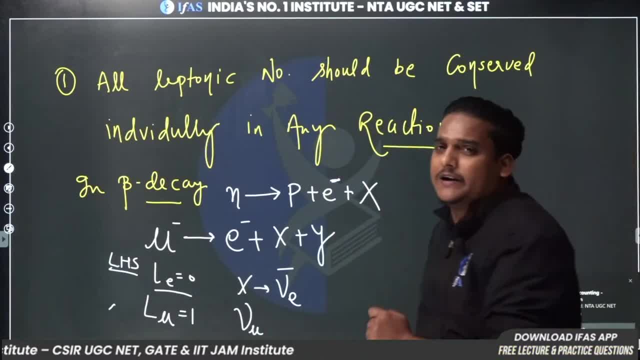 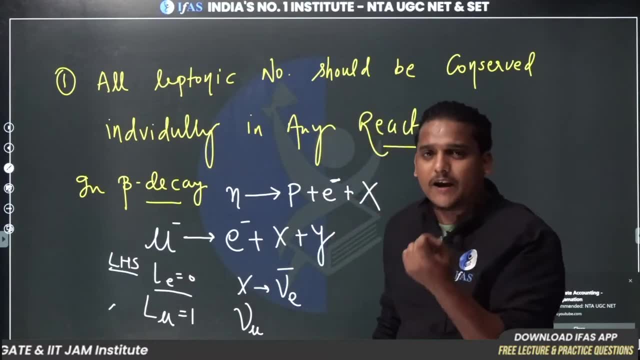 quickly put things in your notes, because I have given you the guarantee that spend 1.5 hours with me here, you will not need to read particle physics separately. you will not need to read particle physics separately. this is my guarantee. I have completed nuclear physics last week. 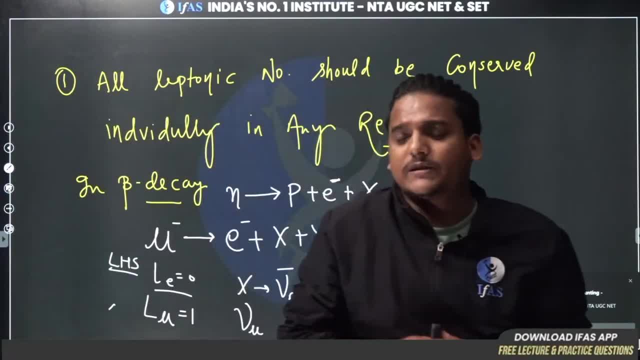 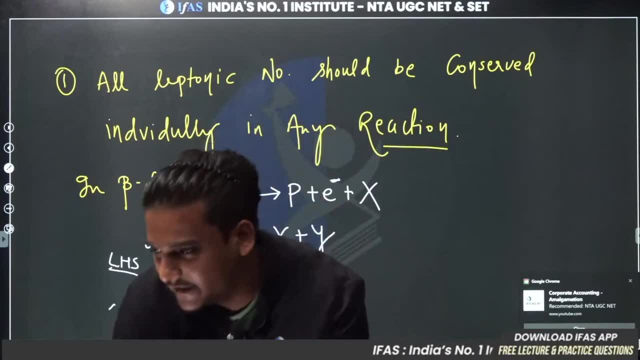 I have tried to complete the important things. those students who have not seen, go and see and keep sharing the link of the session. connect the maximum majority of students here. it is clear, sir. very good, perfect. I am not liking the session. there are 46-47 students and I have only 25-26 likes. 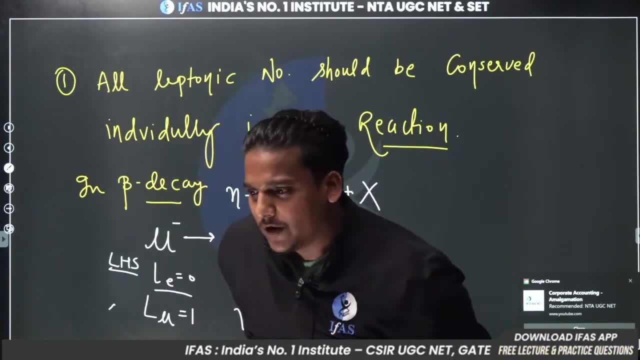 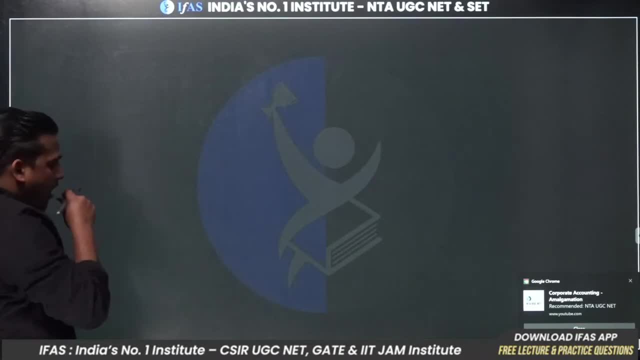 I hope it is clear for Abhirub Chaturvedi to speak. Naushin Ji sir's imagination is clear. it is very good now. second thing: our second quantum number is baryonic number, baryon number. so baryon number is defined for. 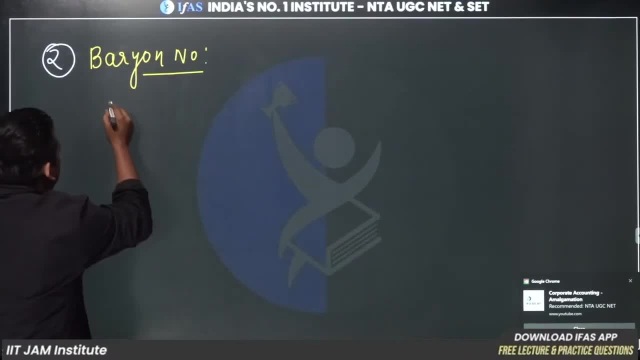 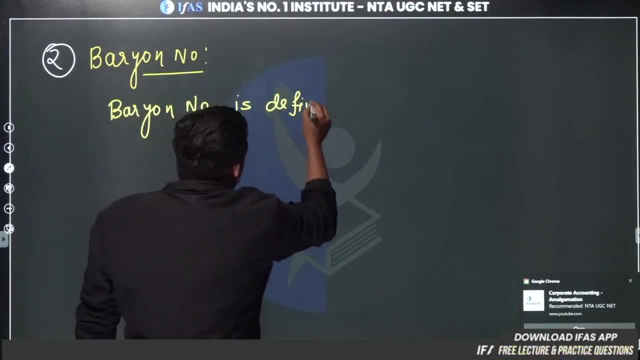 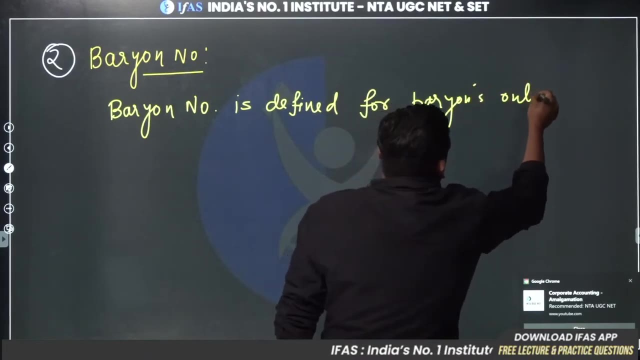 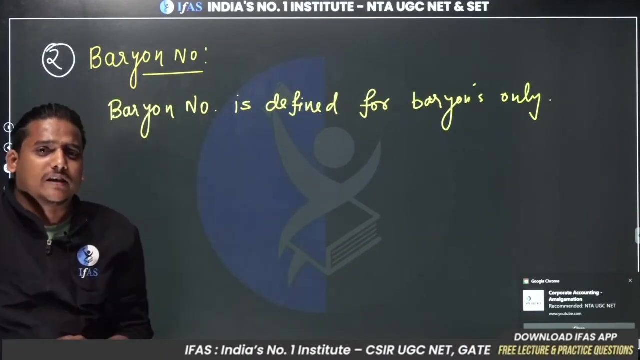 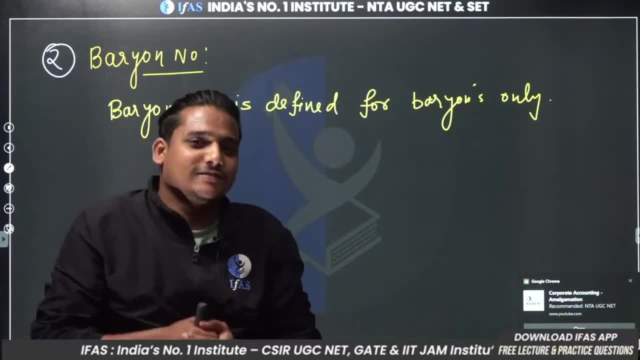 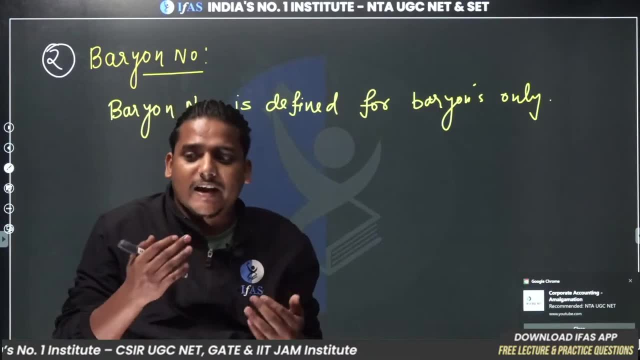 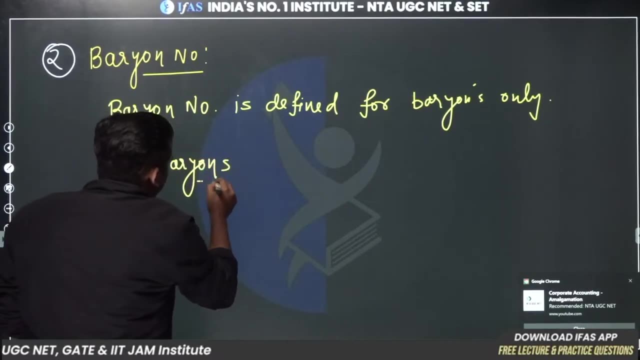 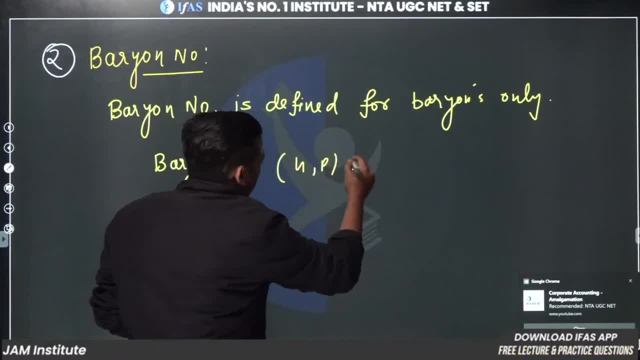 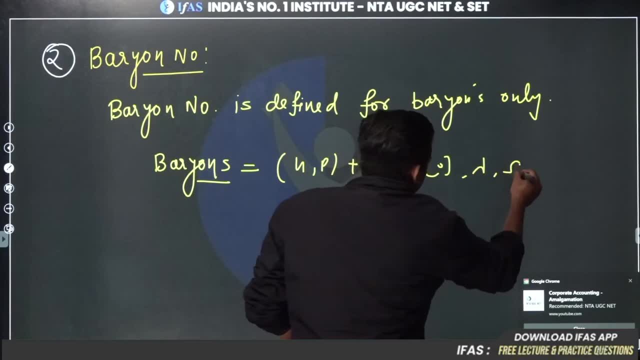 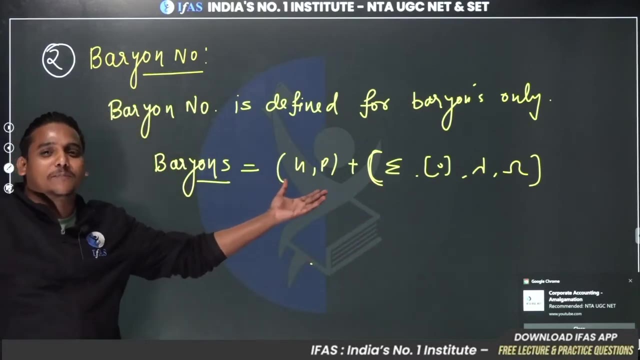 Nucleons in which Neutron, Proton Plus Hyperons, In which you get Sigma, Cascade, Lambda, Omega. This is your baryon family, Sir. you Hairstyle Looking Dressing. Thank you so much. Actually, my hair was running here and there. 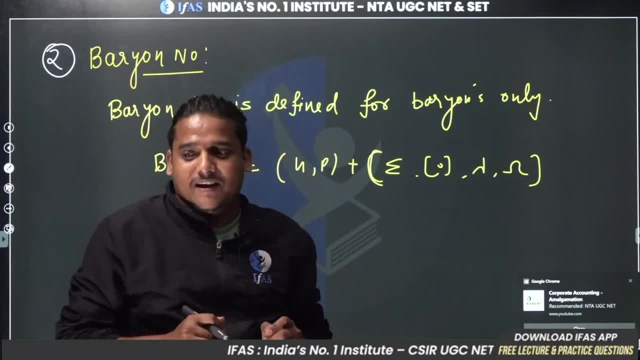 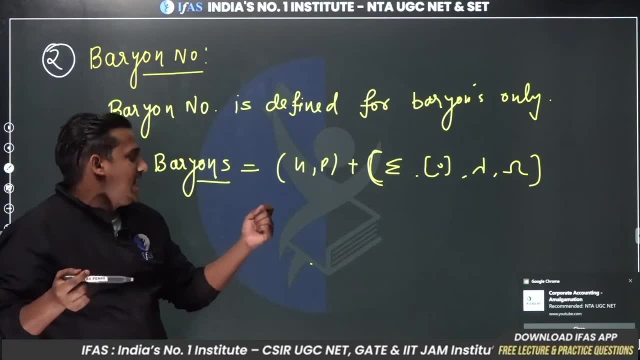 I thought: let me control my hair, Otherwise my focus gets disturbed, Isn't it? I used a hair band of 10 rupees. I used a 10 rupees hair band And some old hairstyles. My face is dirty. Nothing good happened. So what are baryons? 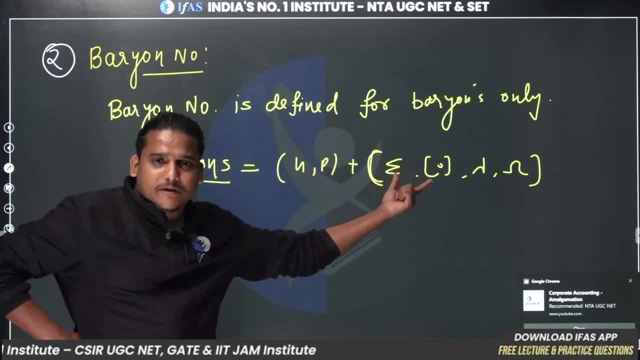 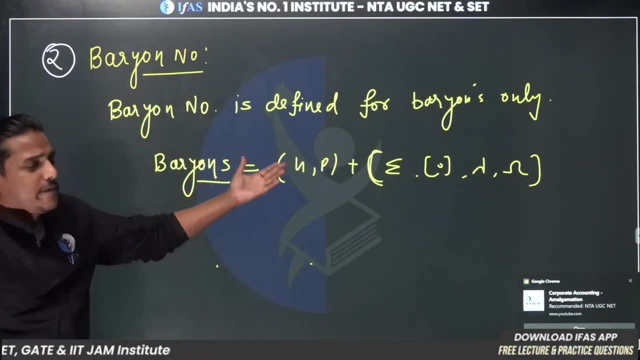 Nucleons plus Hyperons. Is this clear to all students? Is this clear? There is no doubt in this Very good Perfect. So, for all these baryon particles, A quantum number is defined, Which is called baryon number. And what is your baryon number? 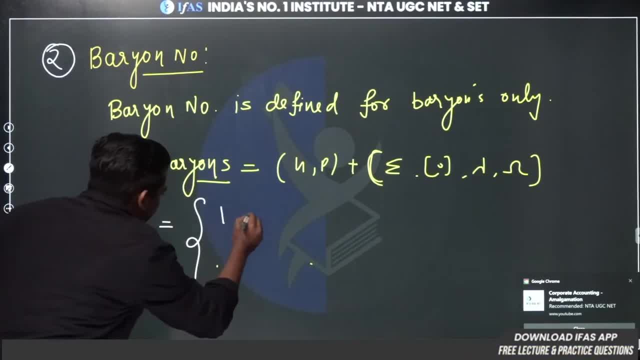 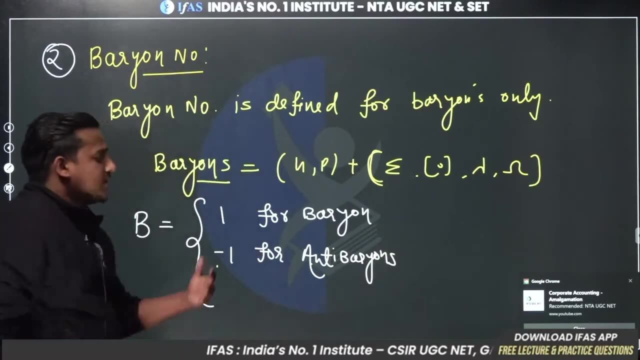 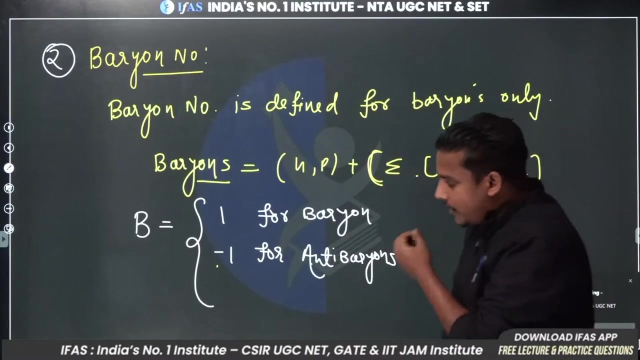 This is simple: V is equal to 1 for Baryons And Minus 1 for antivaryons. And apart from that, If baryons- I am joking- And apart from this, If there is no baryon in any reaction, Then your baryon number will be zero. 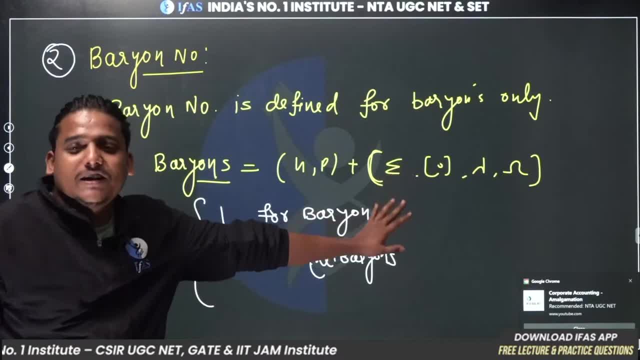 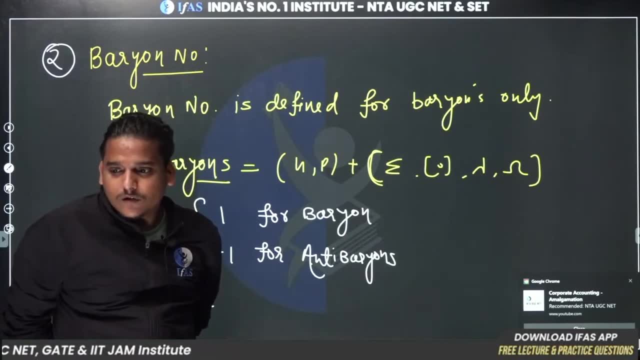 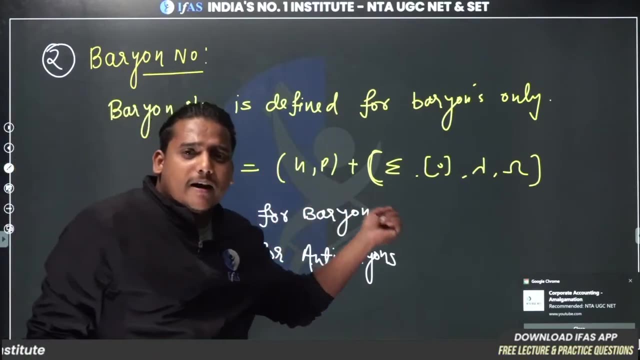 Is this clear to all students And all our dear friends? Is this clear to all? Is this clear to all students? Is this clear to all students? Is this clear to all students? And you have to keep in mind That in any reaction, Our total baryon number should be conserved. 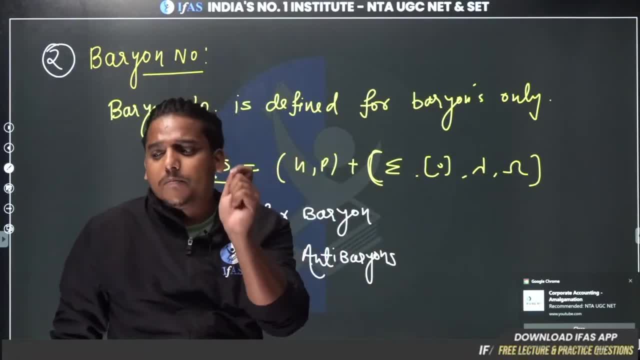 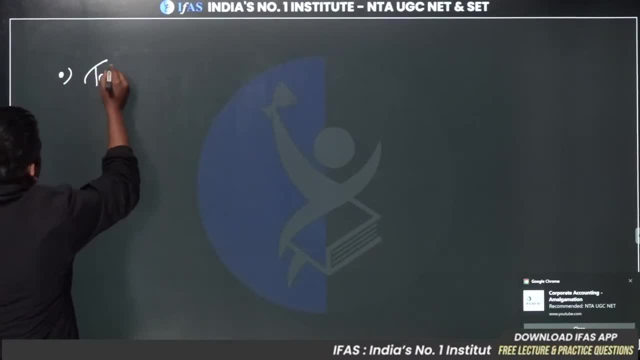 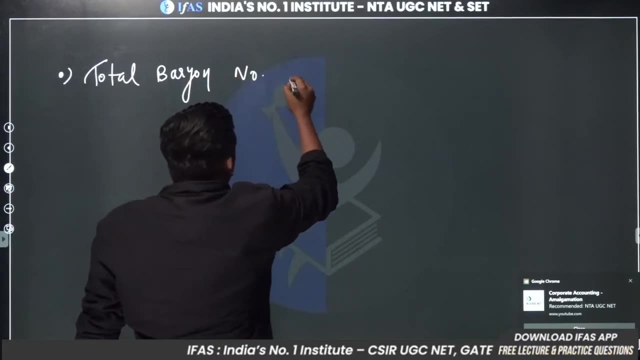 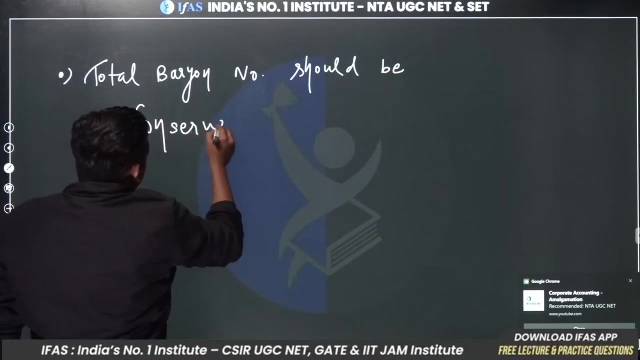 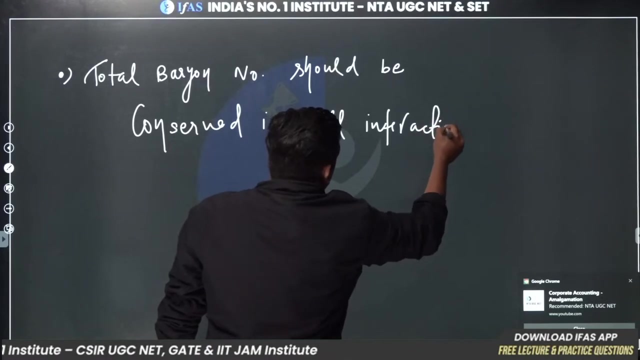 Always keep in mind Our total baryon number should be conserved. Write this statement too. Write this statement too, Before that: Total Baryon number. Baryon number D, Basics, etc, Basics, etc. This is total basic Baltonic and baryonicè. Now your important quantum number. 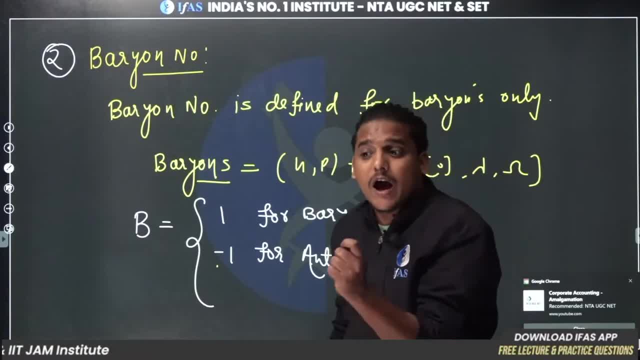 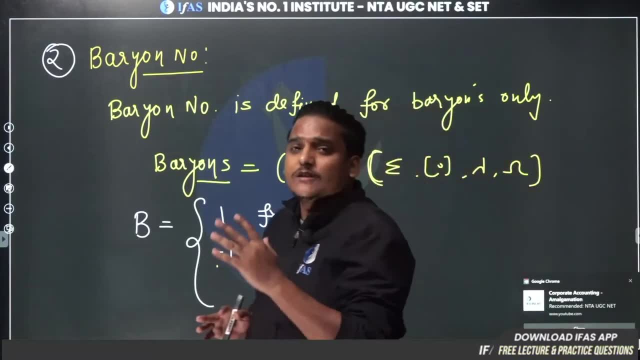 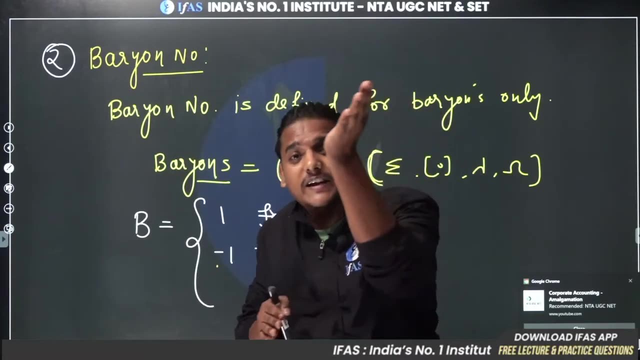 Which is 과�s, why is important, Which is very important. Let's go to the third quantum number, and this is a quantum number that will help you a lot to tell the type of interaction. If the reaction is allowed, then which interaction is allowed. Is it allowed by strong interaction? 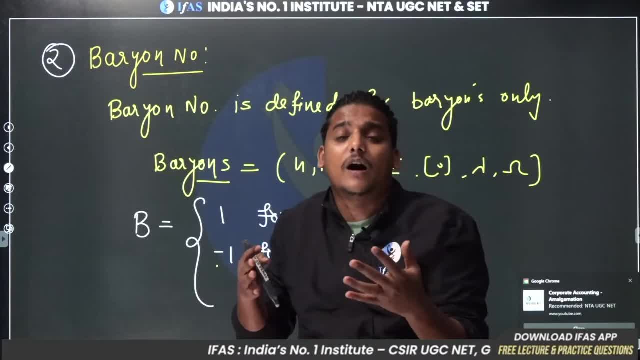 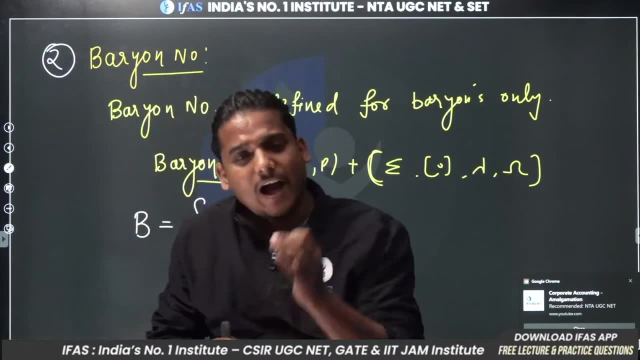 Is it allowed by big interaction Or is it allowed by EM interaction? That will help you in iso spin, Sir. do you have easy day classes? Every day, exactly Every day, you have class. My particle physics class was at 8 o'clock in the night. 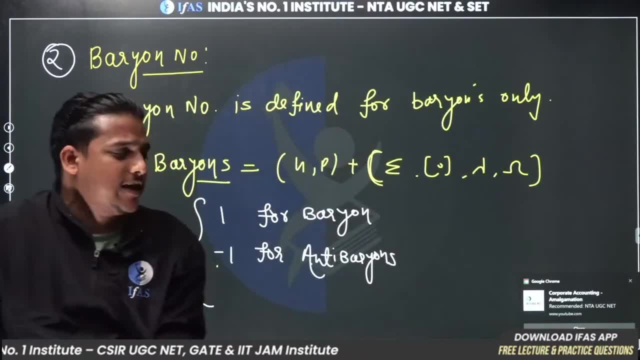 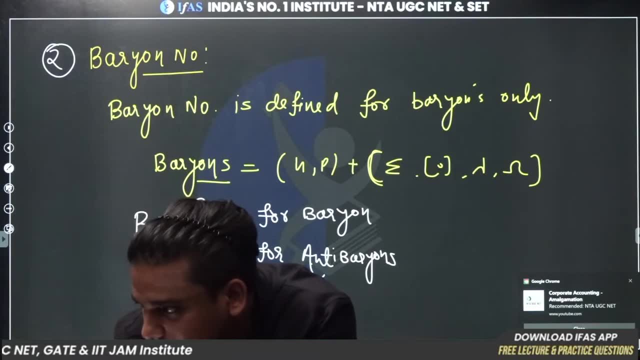 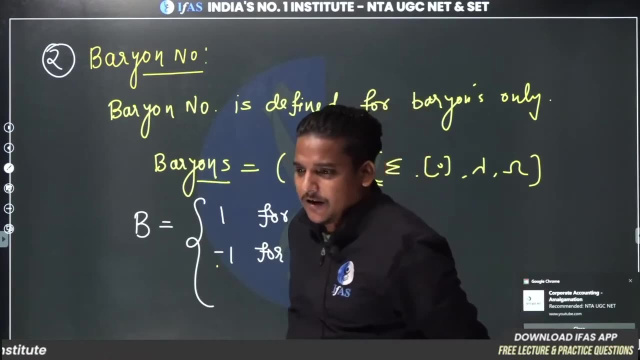 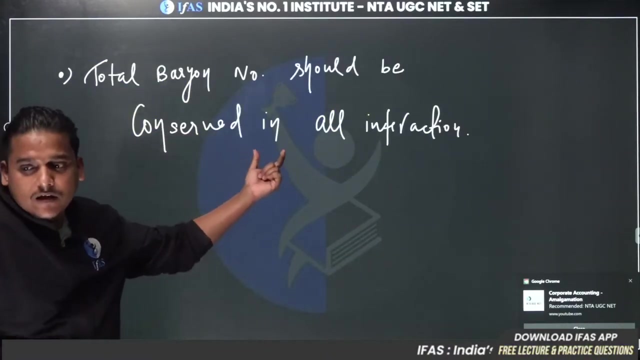 It started early. You have not lagged much yet. Then we will move towards iso spin. And give me permission in the comment section that, sir, done, Done. Okay, sir, avatar is clear. Very good, Let's move forward. I hope you have written this statement. 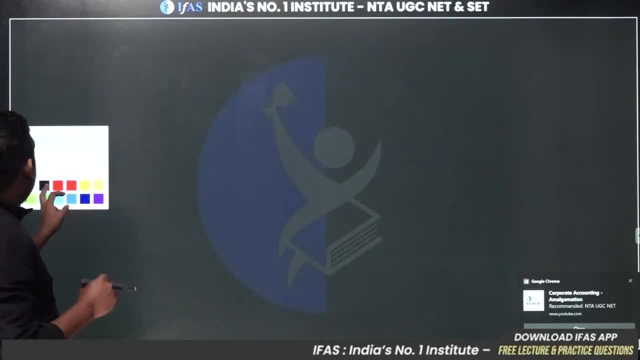 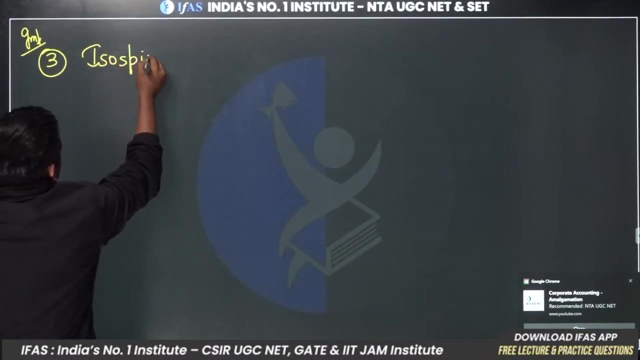 Sir, you do not apply 50.. Apply 50 a day, At least, at least. Come on Now. the third quantum number is very important. Write here important. This is iso spin. We will talk about iso spin And we will talk about its third component. 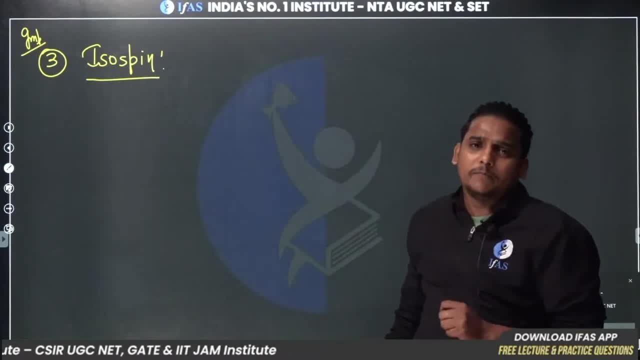 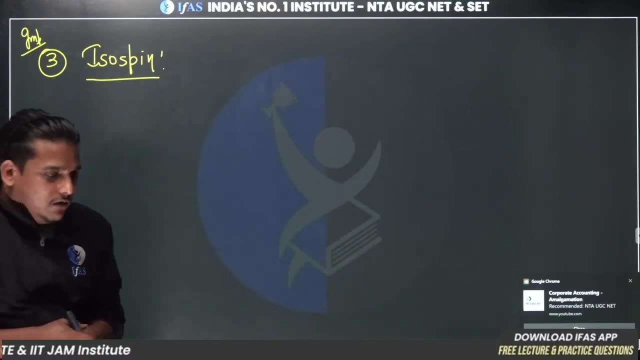 You will get the PDF. Don't worry, After the lecture, you will get the PDF. I will send it to you. You will get the PDF in the free section in the IFS app. Don't worry, You will get the PDF in the free section in the IFS app. 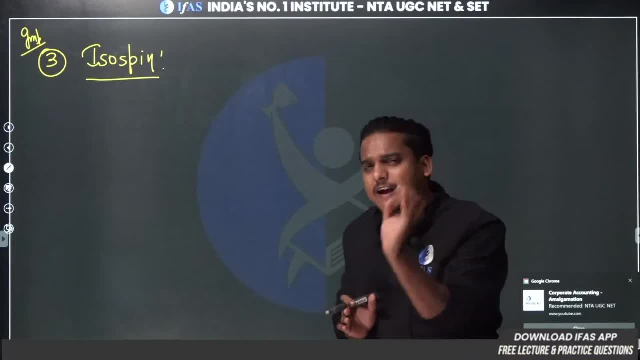 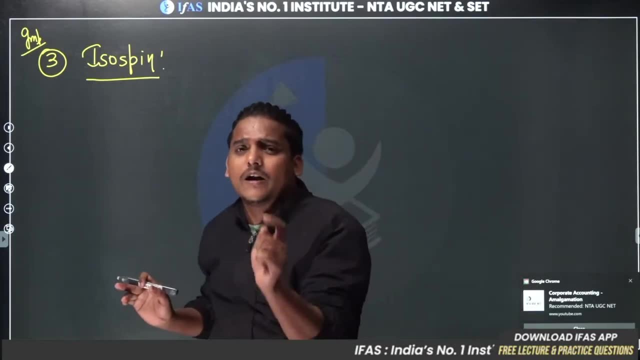 See, always keep in mind The first point. I will give you each point. Just be patient. The first thing is iso spin. It is defined for hadron particles only. It should be clear in the first mind That iso spin is. 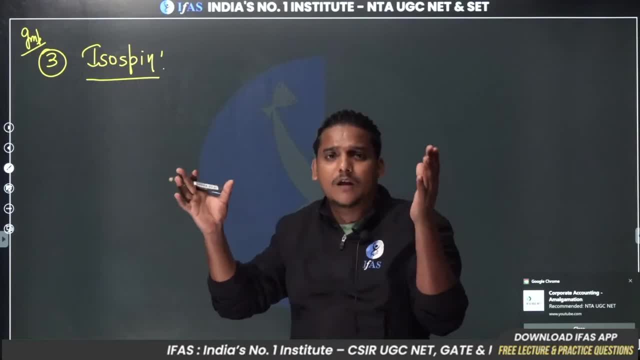 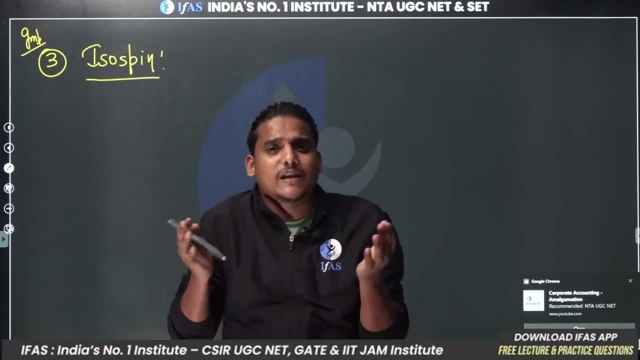 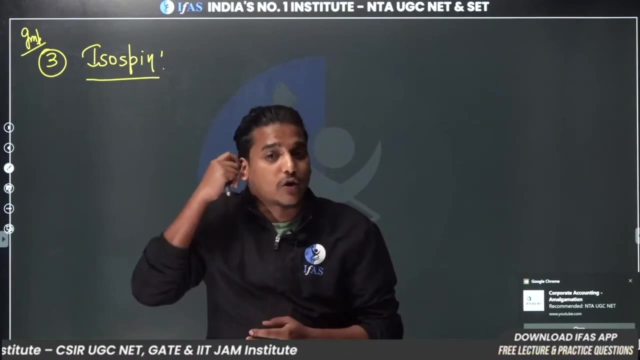 defined only for hadrons. Is it clear: Iso spin is defined for hadron particles only, Or you can reframe it and say that iso spin is defined for particles that are participating in strong interaction, Because hydrons will participate in strong interaction. 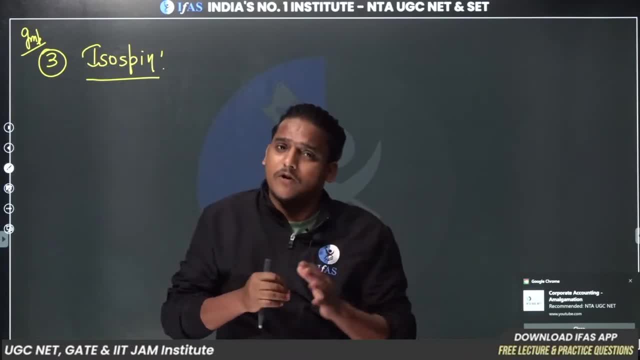 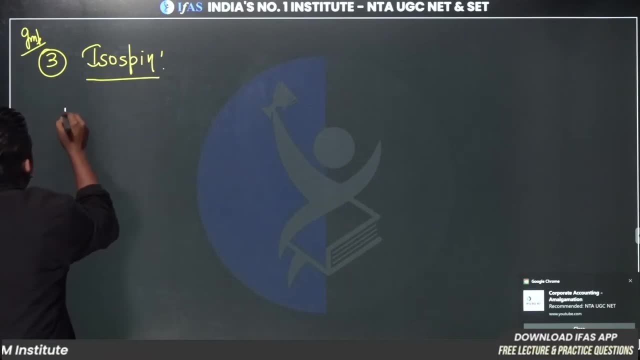 Iso spin is not going to be on your left. So iso spin is defined for hydrons. Write here the first point. Write each point. All your concepts will be clear. Iso spin is defined for. iso spin is defined for. iso spin is defined for. 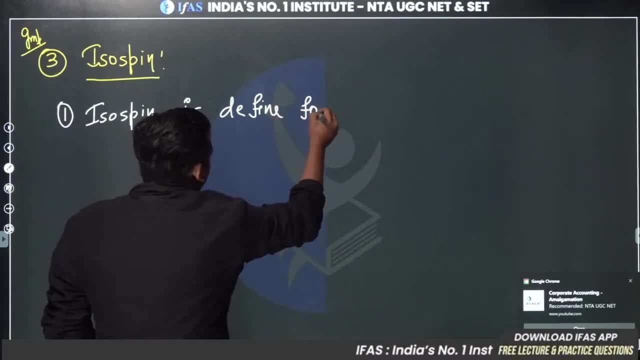 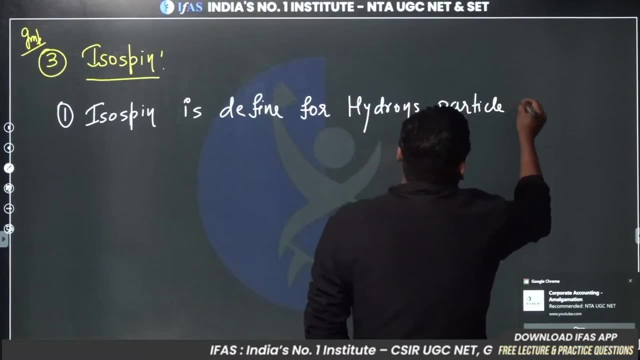 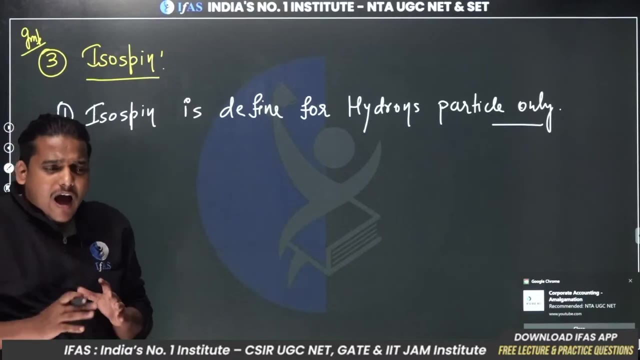 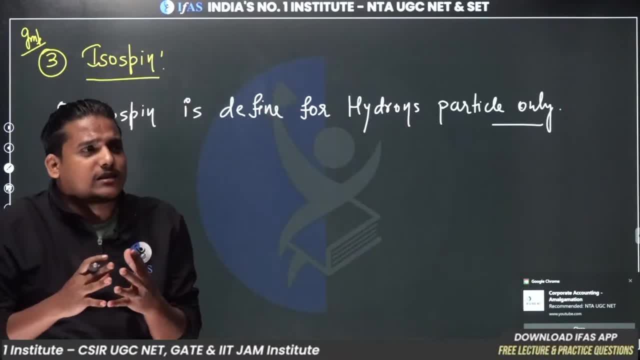 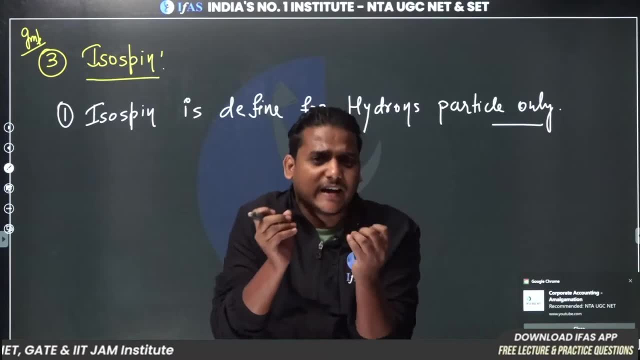 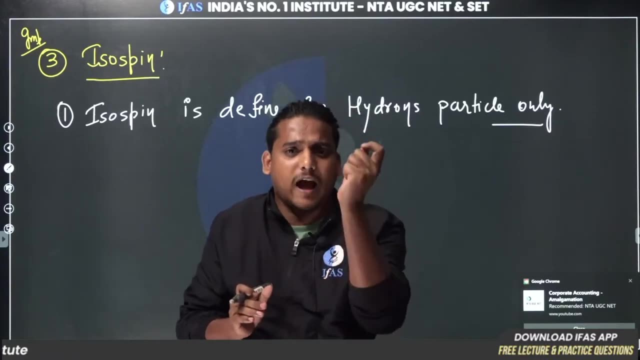 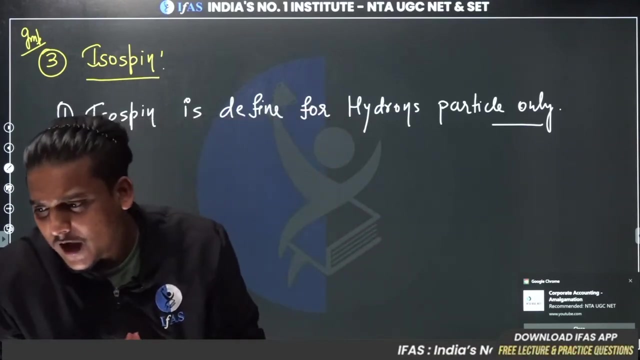 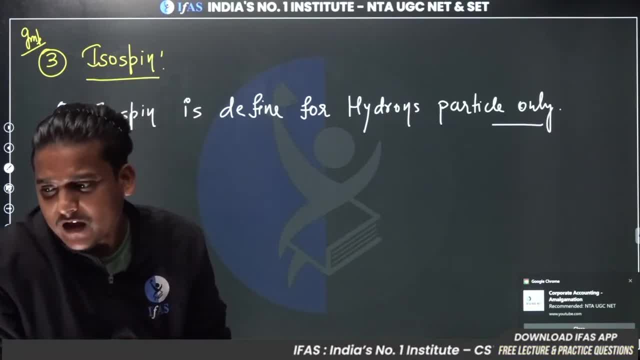 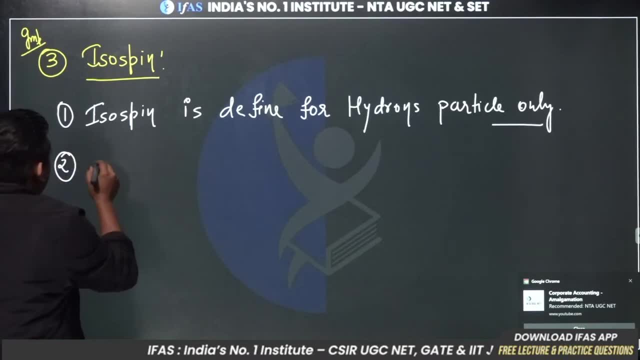 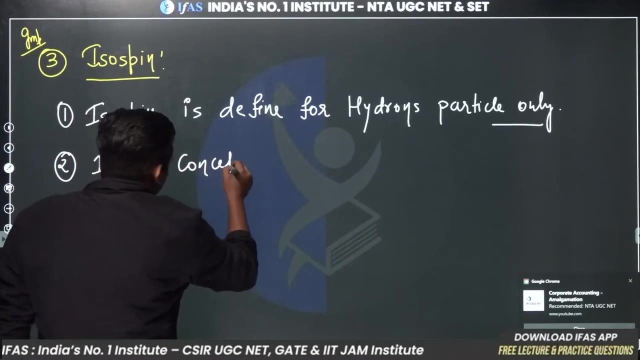 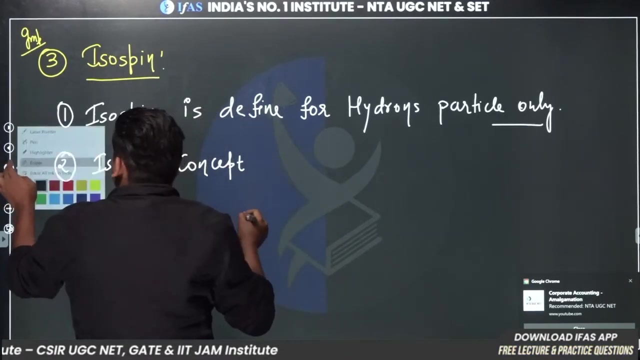 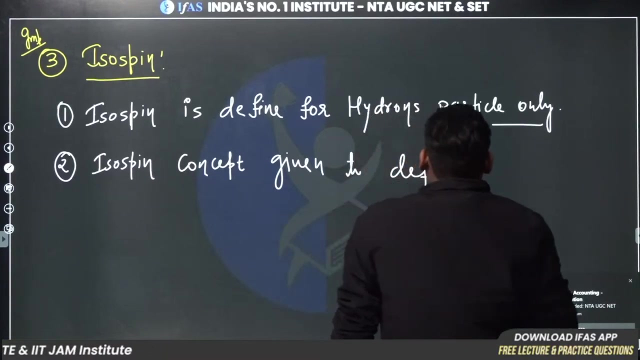 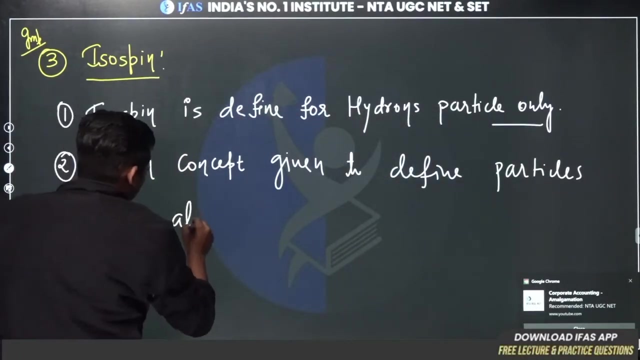 Please use more English words. Be careful, sir. It will be found on the pdf telegram. Be careful, Focus here. So iso spin concept. iso spin concept. iso spin concept gives given to define particles of almost equal masses. particles of almost equal masses. 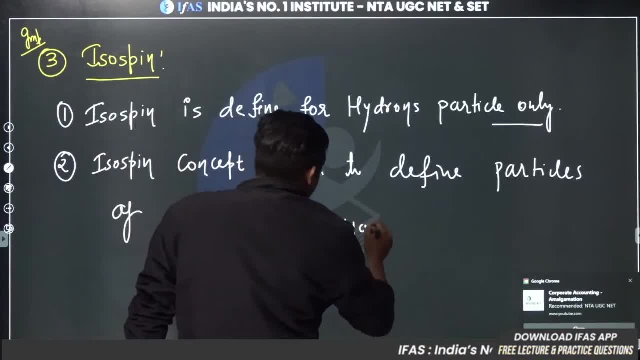 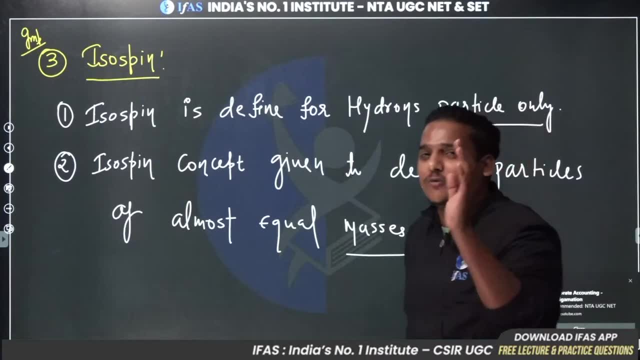 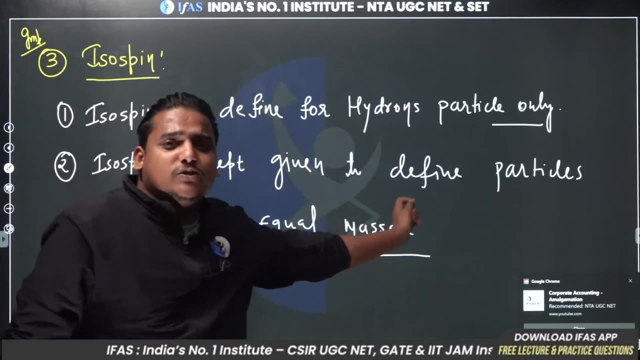 So these are all about the basics. Now for different particles. Well, here is half the step. Thank you, guys. You have oned half the step. Now let's move to the next step. iso spin is defined for hydrons particles only. 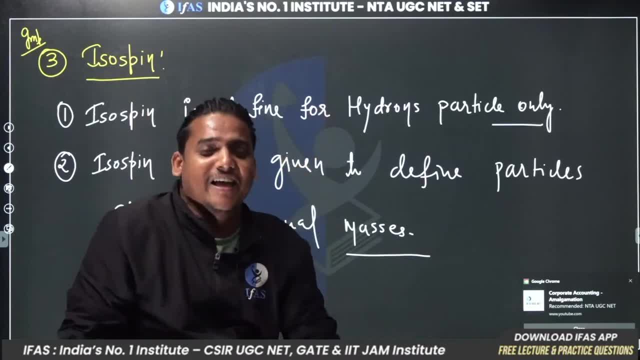 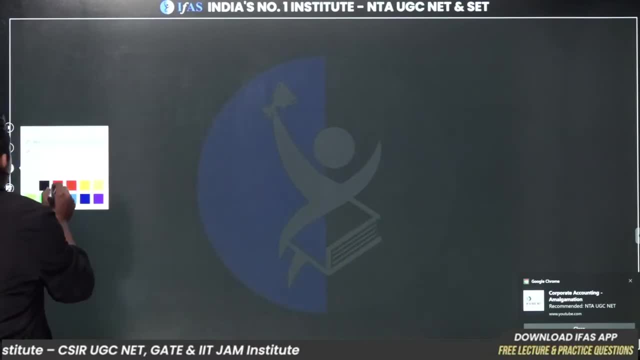 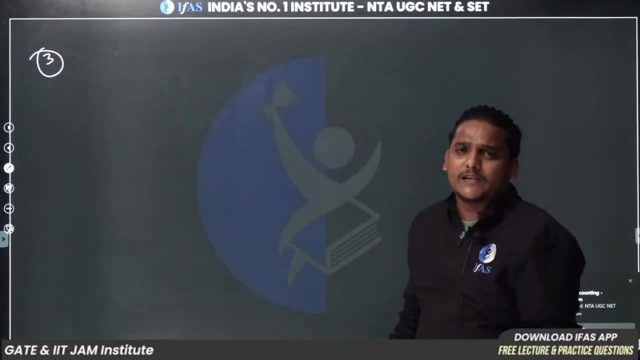 And iso spin is defined for particles of identical masses. Let's move to how iso spin is derived for different particles. Please write the important points of it. First write the points. This iso spin is more or less identical. like in quantum mechanics we study algebra of angular momentum point to be noted like: 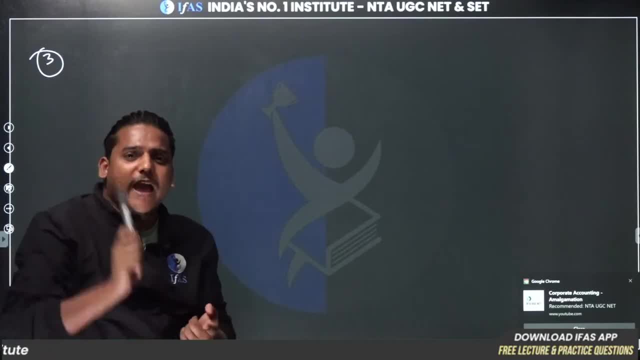 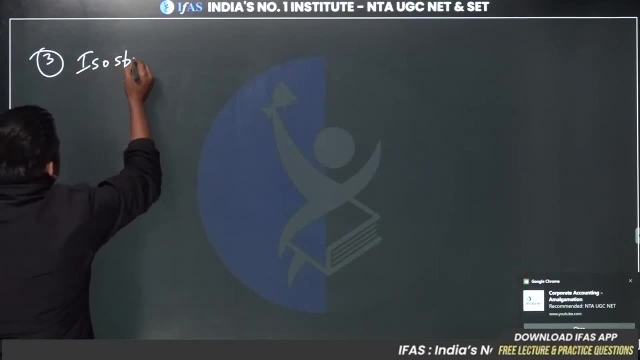 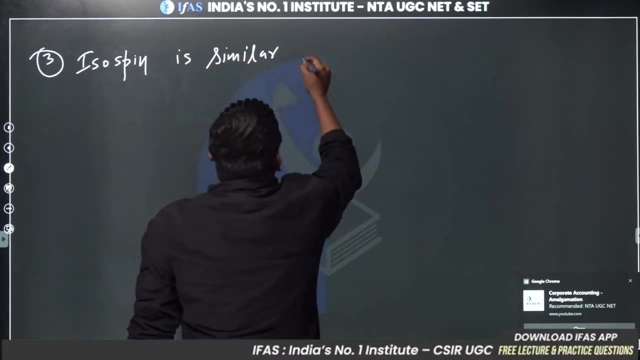 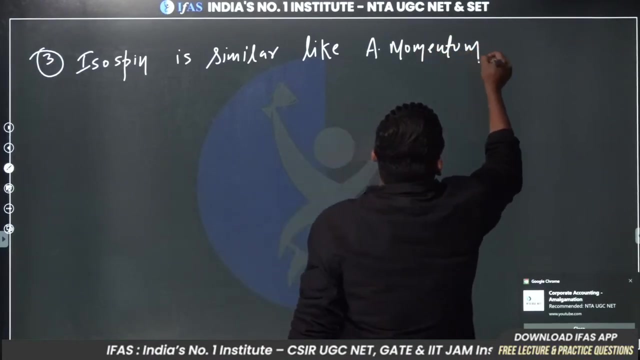 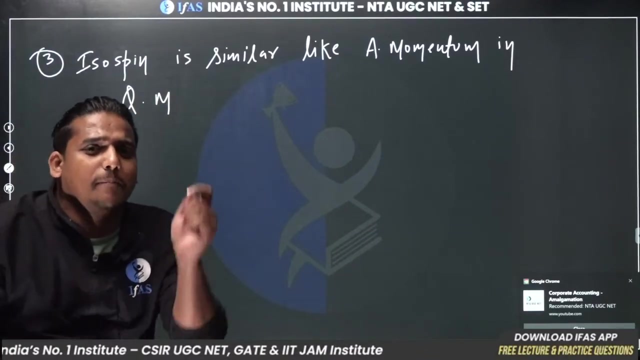 in quantum mechanics we study algebra of angular momentum. iso spin also follows the same algebra. so here write the third point: iso spin. iso spin somewhere is similar like angular momentum of quantum in quantum mechanics, like angular momentum in quantum mechanics. what does it mean, iso spin, which will always be added vectorly? suppose you have the particle? 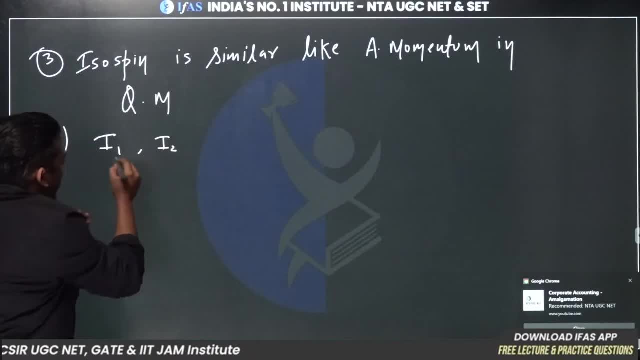 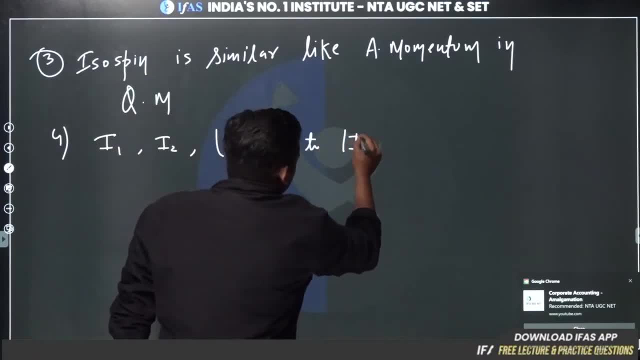 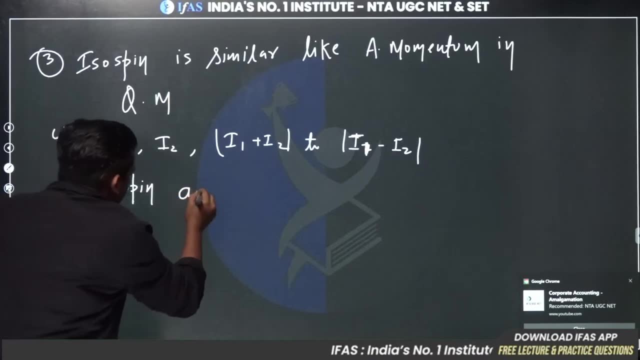 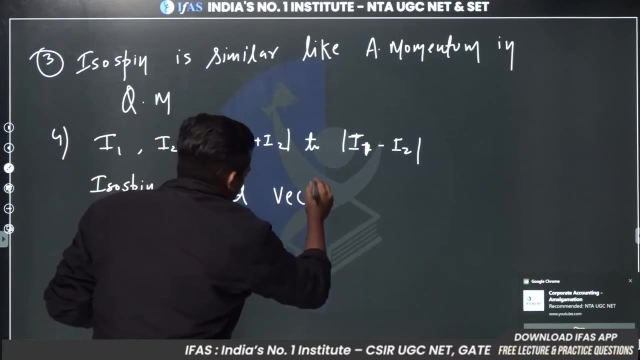 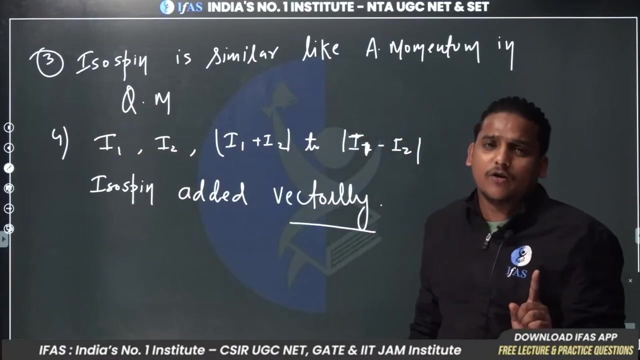 i1 minus i2. so you write statement isospin. I said I will write one point: isospin added vectorally, not algebraically. isospin added vectorally. keep this in mind. isospin will be your vector addition, not algebraic addition. now I am not talking about third component. 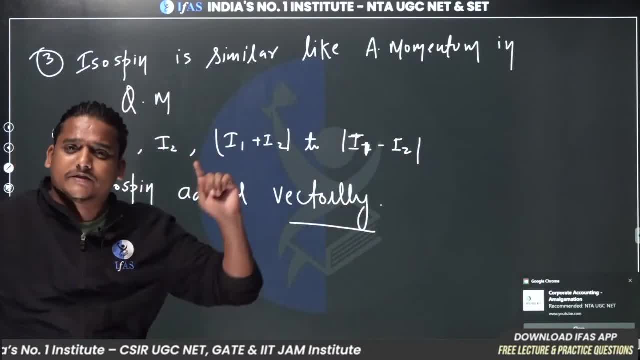 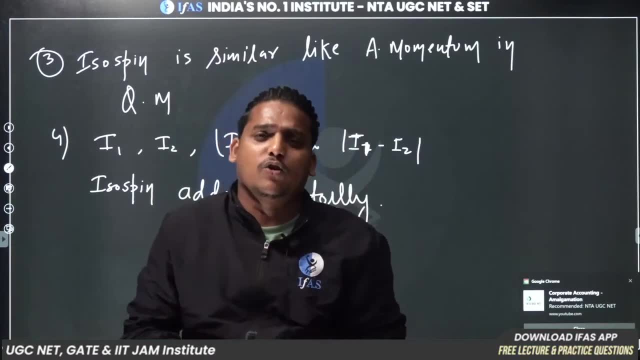 now I am talking about isospin. are you getting clear statement one by one, because all these statements are very important to know in reaction, that reaction is happening with strong interaction or with weak interaction or with EM interaction? if you will not add correctly, then what will happen to your son? 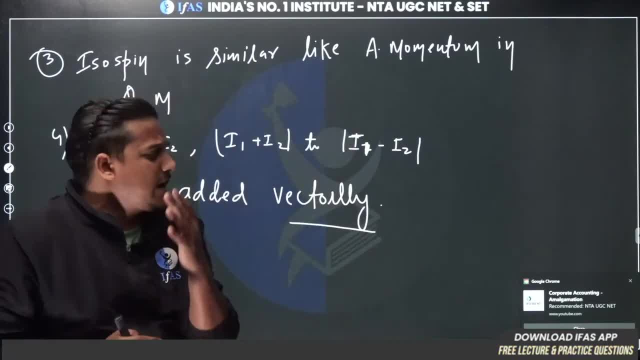 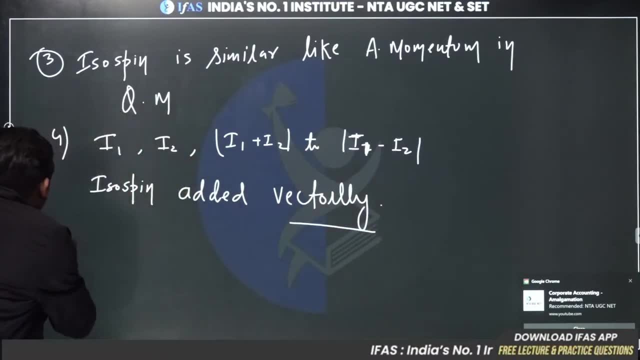 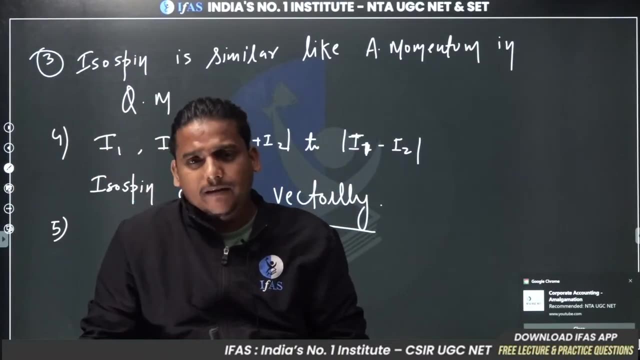 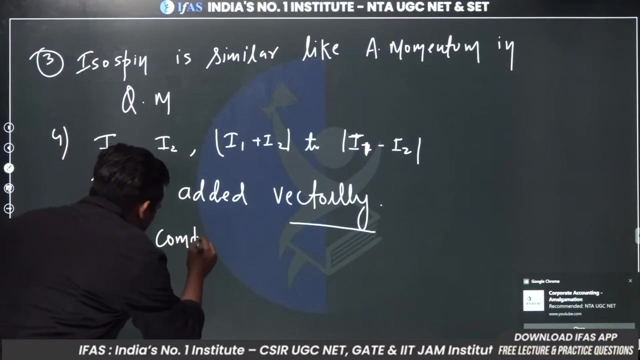 you should know one thing: that how you will work. ok, next point: write: corresponding to each isospin. a third component of isospin is defined as i3. is it clear? corresponding to each isospin third component is defined as i3. third component of isospin. 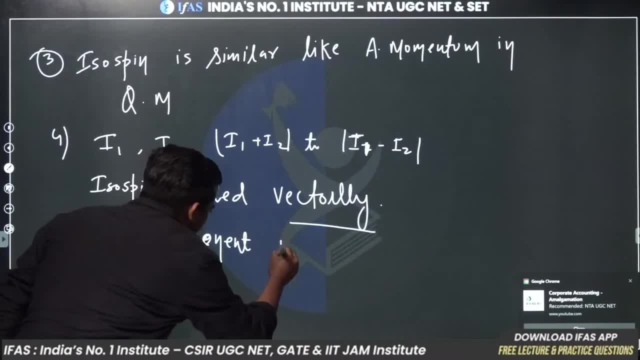 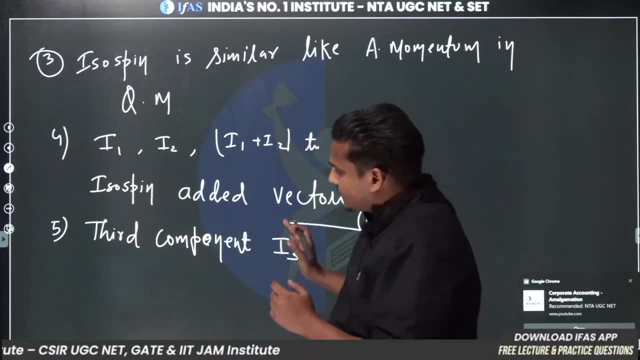 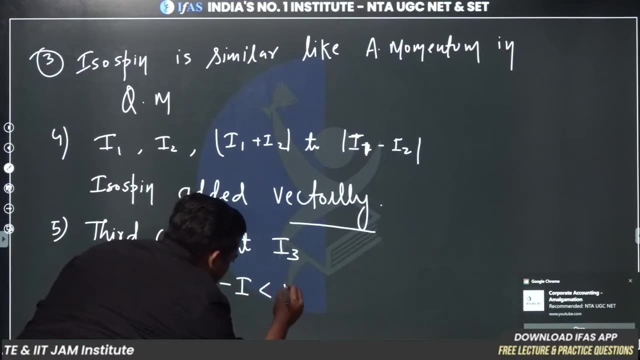 that is i3. third component is i3, but what will be the values of i3? we will discuss this later. the third component: the values of this will be from minus i to minus, i to plus. i keep this in mind. from minus i to, in steps of 1. 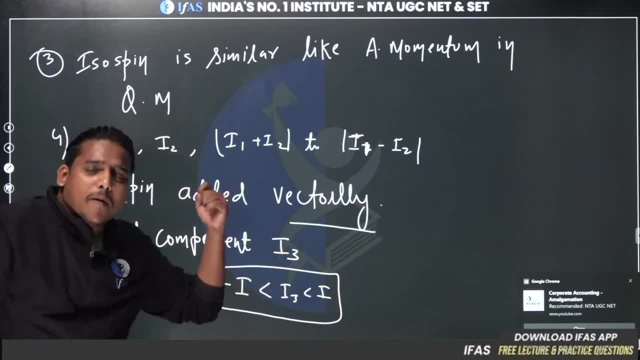 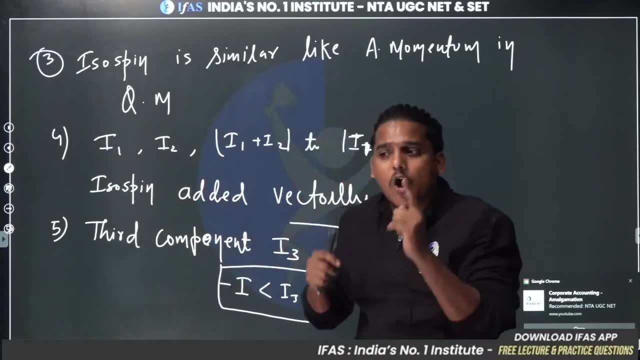 in steps of 1. point to be noted: the values of i3 will be from minus i to i in units of 1. keep this in mind. this is very important. ok, and always keep this in mind. this is algebraically added, not vectorically added. is this much clear? 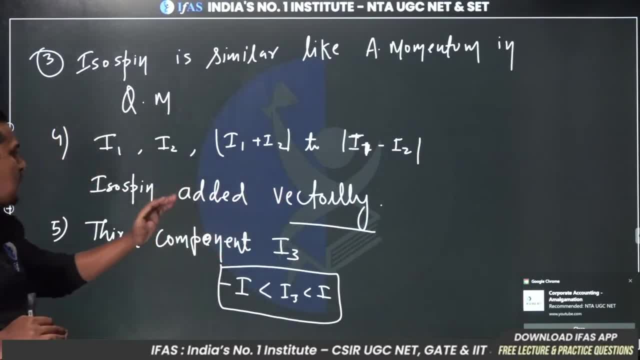 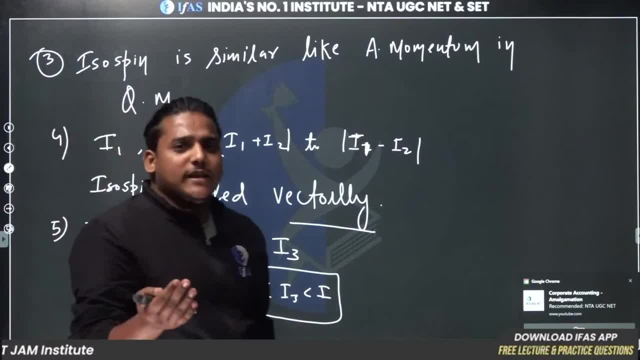 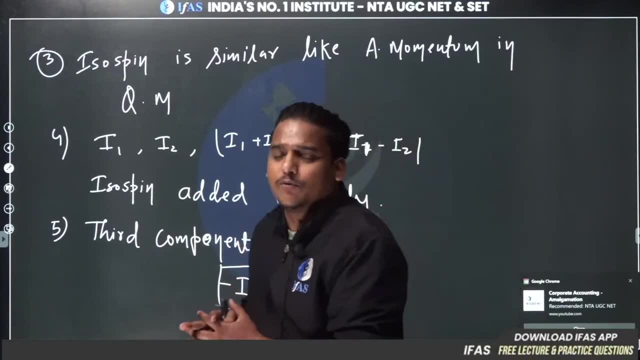 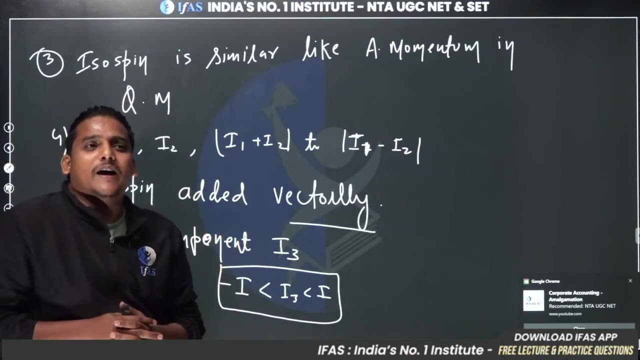 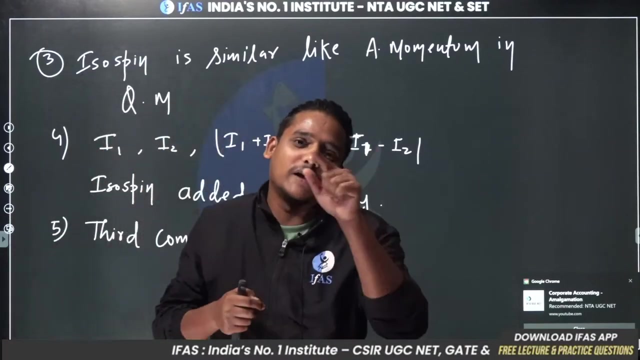 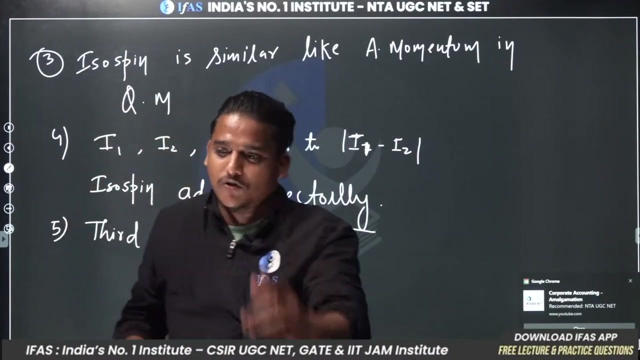 ok, ok, sleep, sleep, sleep, sleep, ok, sleep, sleep, sleep tonight, toilets, Whether Whether our students also. He is studying with me, leaving his ISTA reels. This is a huge sacrifice for him to leave his ISTA reels. I just want you to understand this. If you have spent an hour with me, then take something from here. This is my motive. 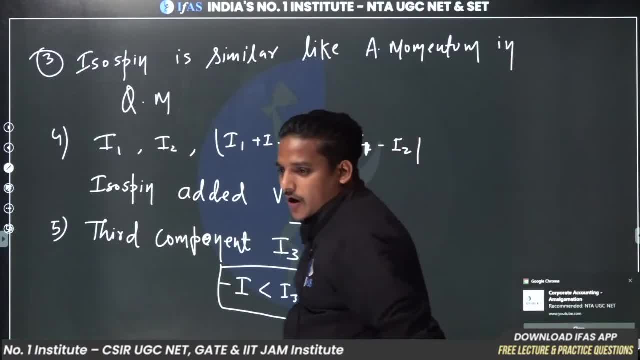 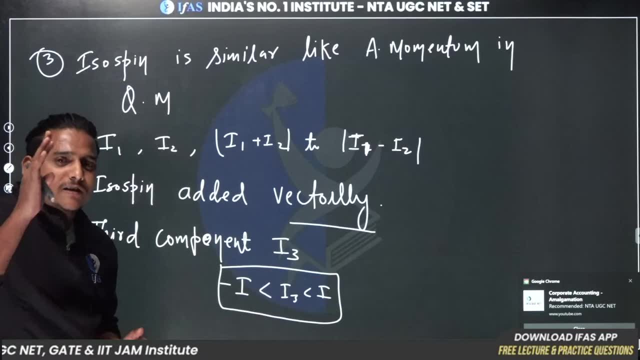 Clear. You will not go back empty-handed. I hope it is clear. Let's move forward. Very good, You have left your ISTA reels and you are giving time to your studies. This means you are going in the right direction. You are doing the right thing. Keep this in mind, Because the addiction of ISTA reels is a very bad addiction. 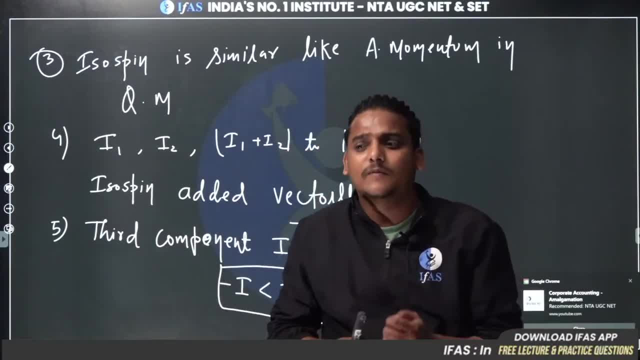 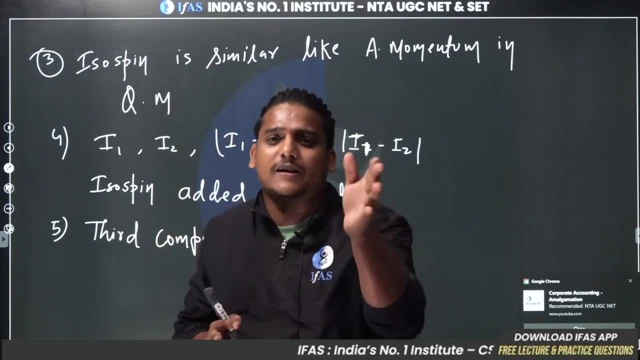 You think that you will scroll the reels for 5 minutes during your studies. The reels will pull you in such a way that it will fill your mind with intoxication. You will not know that you have spent 1 or 2 hours of those 5 minutes, Right. 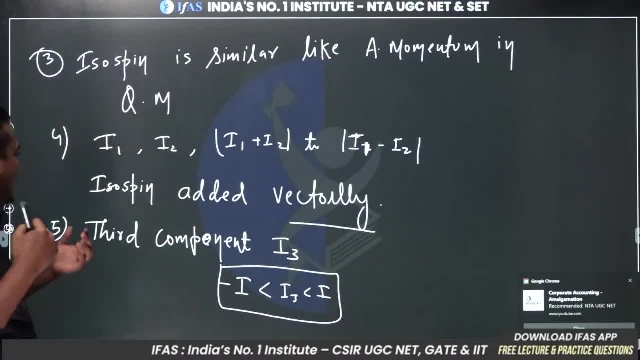 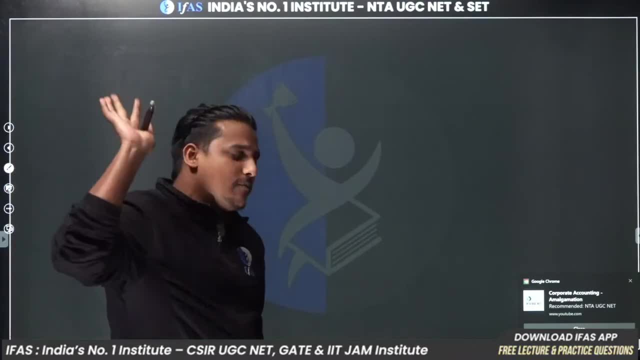 Clear. You will not know that you have spent 1 or 2 hours of those 5 minutes, Because it happens with me too. It happens with everyone. After each reel, you will find someone's father or father-in-law. Gypsy reels are very popular these days. You will find it everywhere. 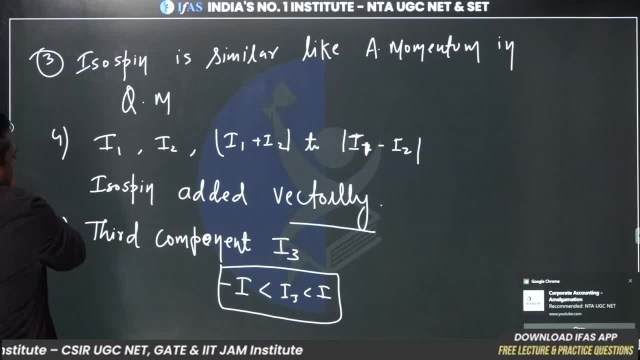 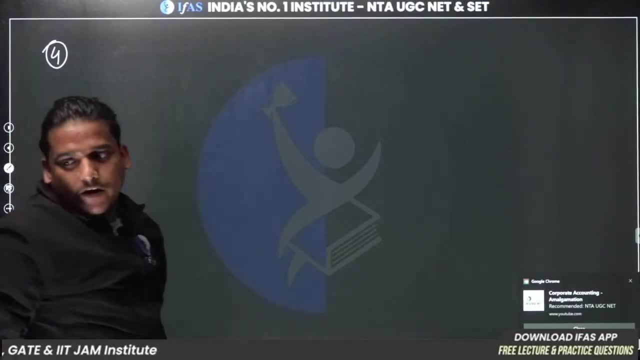 Now let's talk about a very important point: Everyone's father-in-law or father-in-law is running a gypsy, Point to be noted. The next point is very important: Multiplicity of family. Okay, Multiplicity of family. This is the last point, but it is an important point. 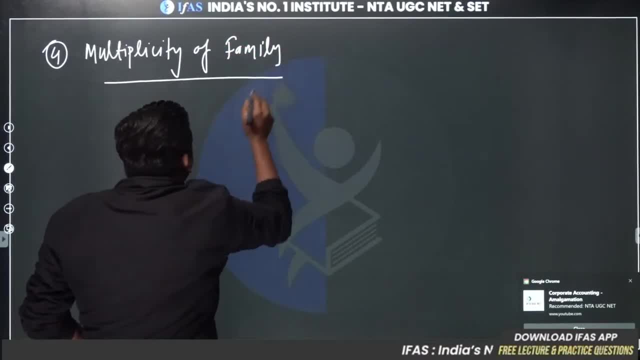 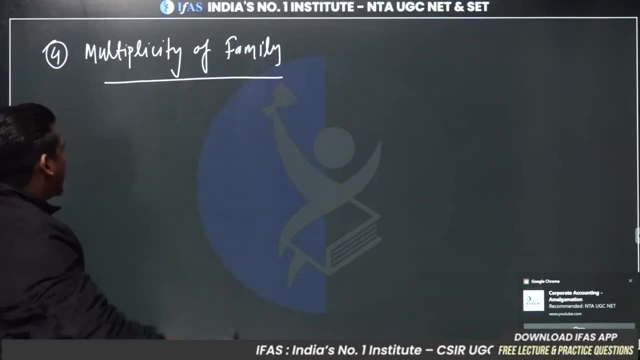 If you want to find the iso spin of any particle, then how will you find it? So keep in mind that. how is the iso spin given? How is the multiplicity given for any particle? For singlet, doublet, triplet family? 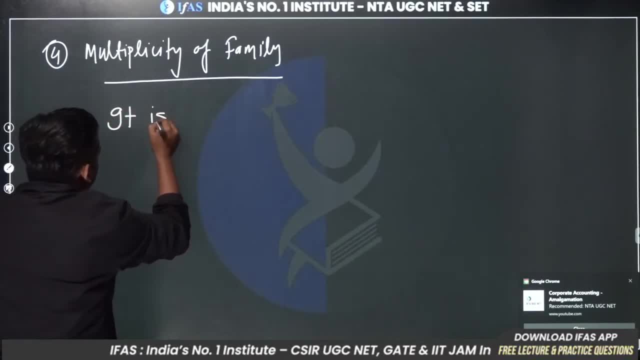 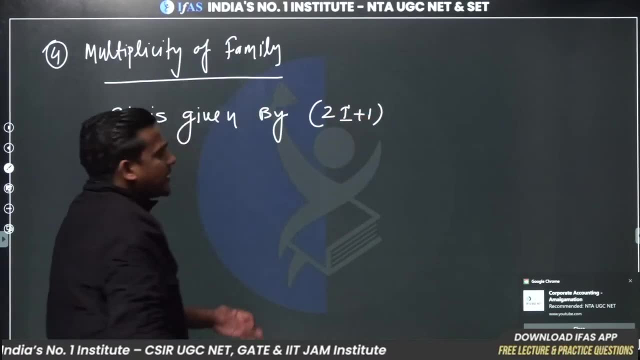 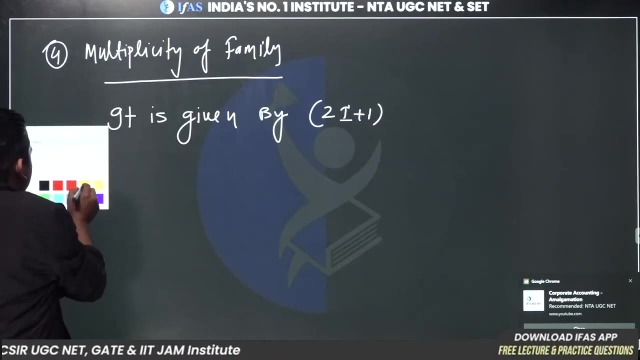 It is given by 2i plus 1.. Right, How is it given? It is given by 2i plus 1.. Okay, Keep in mind. Thank you very much. Okay, No issue, son, Welcome. Now let's do it one by one. 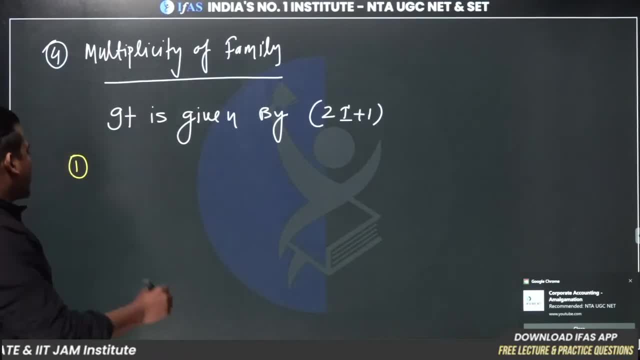 First of all, Let's do it one by one. Let's talk about whose first Suppose. I have to find it for pions. Okay, I have to find it for pions. What are pions? Pi plus, pi minus, pi zero. 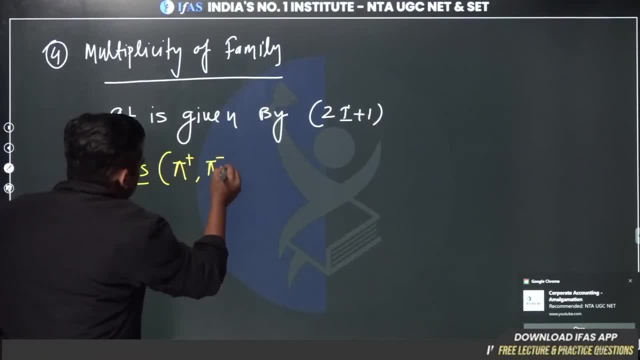 What is pion? It is your triplet. What is pion? It is your triplet. So, son, how will you find it here? Understand that approach. You will be able to find it yourself later. So 2i plus 1.. 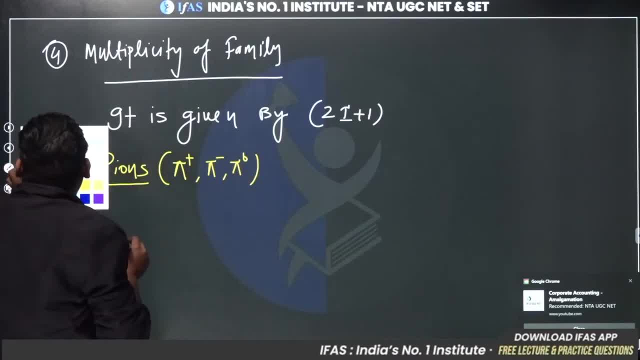 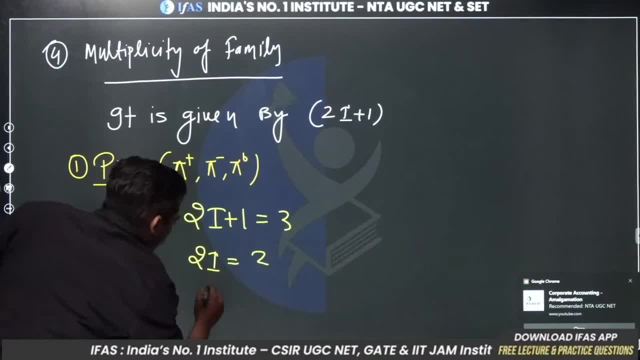 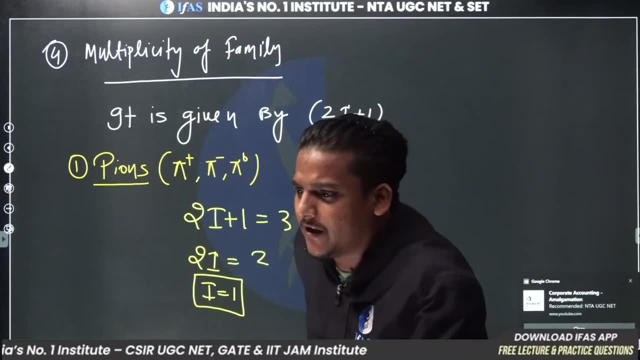 3 minus 1 is 2 and i is equal to 1.. Is this clear, son, Is this important? clear: You won't get iso, spin or particle physics. You won't get it. You won't get it much. 8 to 9 is a very important lecture. 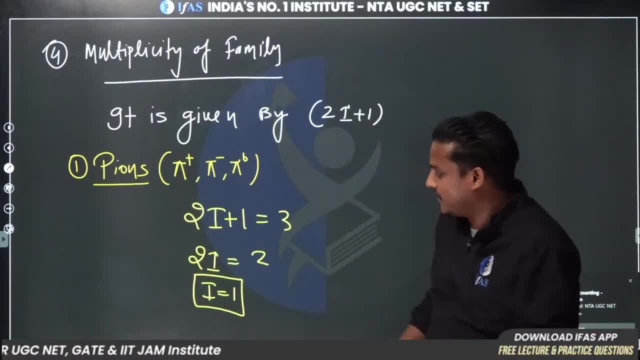 It's a very good thing. It is a good thing You are realizing this. i is equal to 1.. What is this For pions? iso spin has come. i is equal to 1.. But you cannot find it. 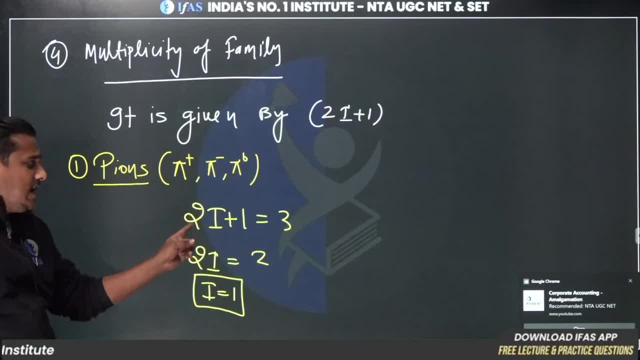 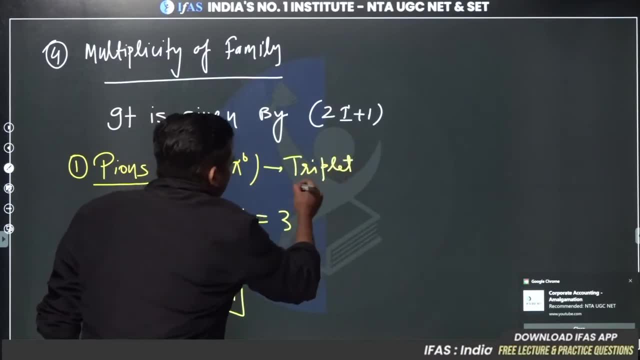 Son, how will you find it? 2i plus 1 is equal to 3.. 2i is equal to 2.. And what is this? It is a triplet. So keep one thing in mind: Any triplet family, any triplet family, will have its iso spin. 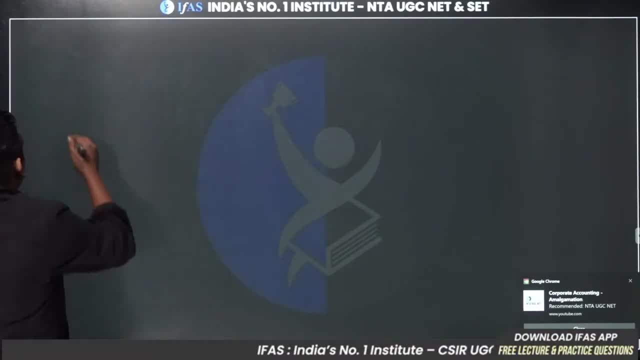 Any triplet family. Let's take out one for doublet. Let's go. What is the other doublet? we have Doublet. we have is nucleons. Right, We have nucleons. We have nucleons. What is doublet? So for this, let's see the iso spin. What will come here? 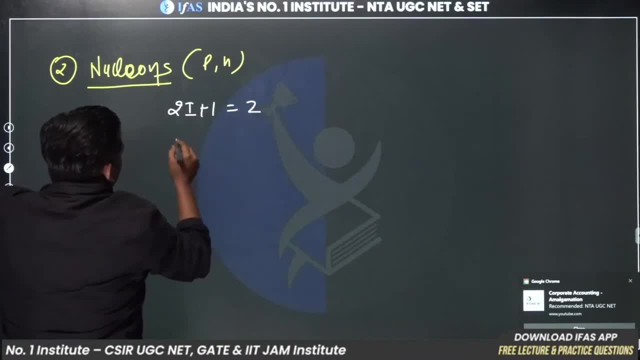 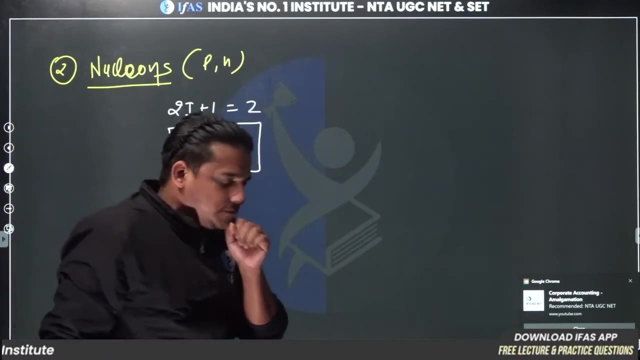 2i plus 1 will be equal to 2.. So from here, I think your iso spin should be 1 by 2.. Right, Yes, The iso spin will be 1 by 2.. Is it clear? Very good. 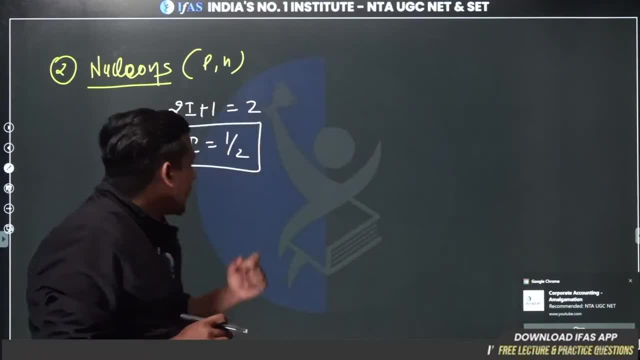 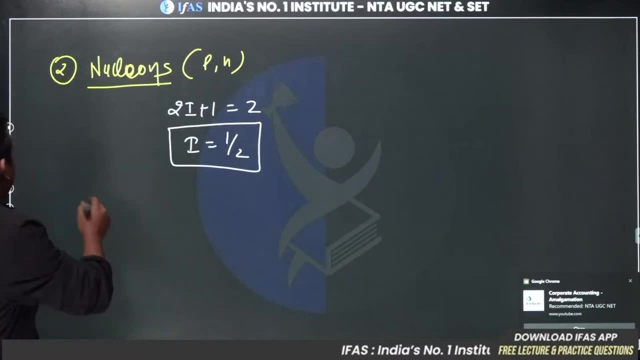 Now let's talk about triplet and doublet. Let's take an example of a singlet. I am not going to take out all of them, Son, it is a very basic thing. You can do all of them easily. One singlet. Tell me the singlet in the comment section. 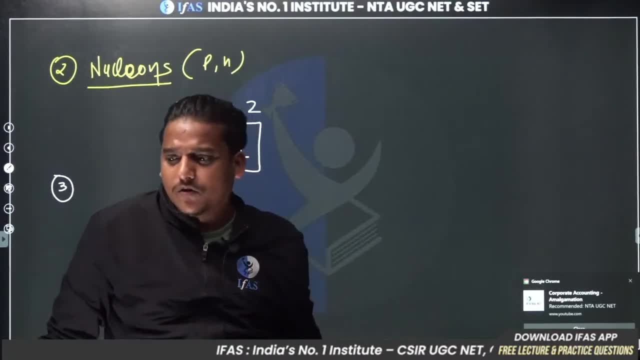 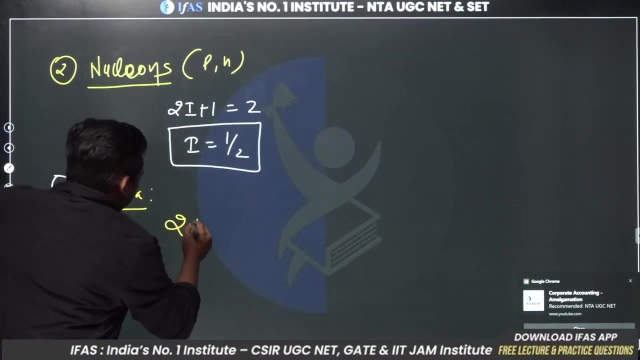 Tell me the singlet in the comment section. Take lambda: Okay, Lambda For this. what will be the iso spin for your singlet? Right now I am not talking about the third component, Son. tell me in the comment section: Will I0 come from here? Absolutely. 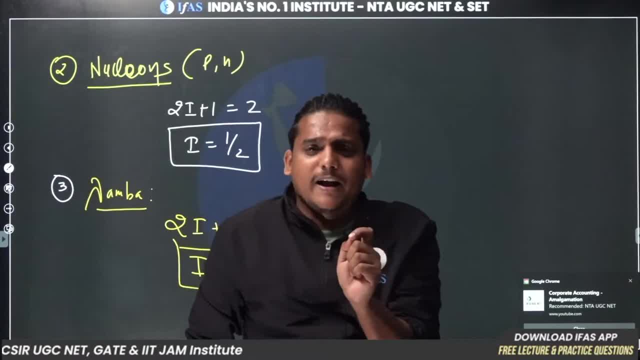 I0 will come. Hey, keep one thing in mind: If it is triplet, then the iso spin is 1 by 2.. Sorry, it is 1. If it is doublet, then the iso spin is 1 by 2.. 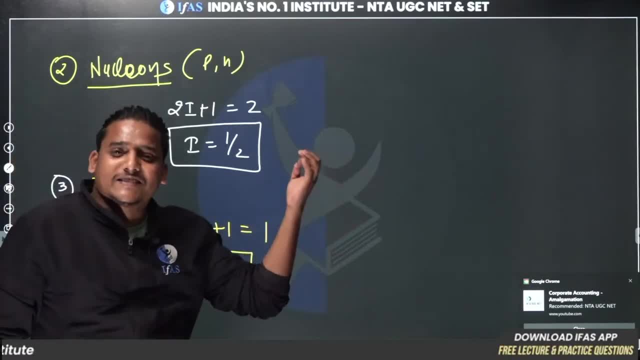 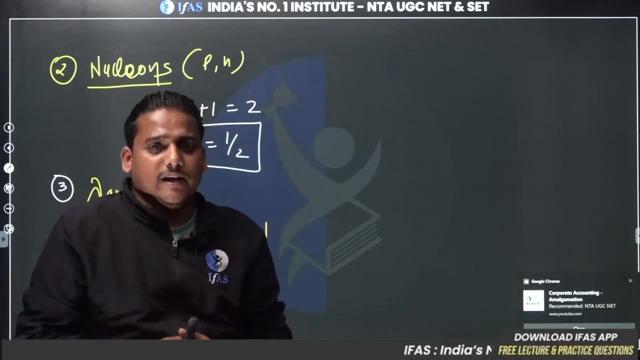 And if it is singlet, then the iso spin is 0. You have to keep this simple thing in mind. Rest, I have told you in yesterday's lecture Which family is triplet, Which family is doublet, Which is singlet. 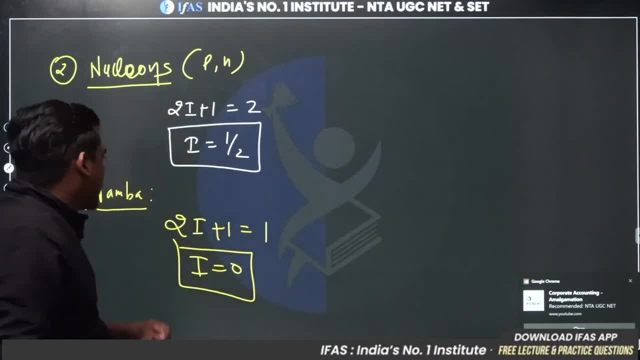 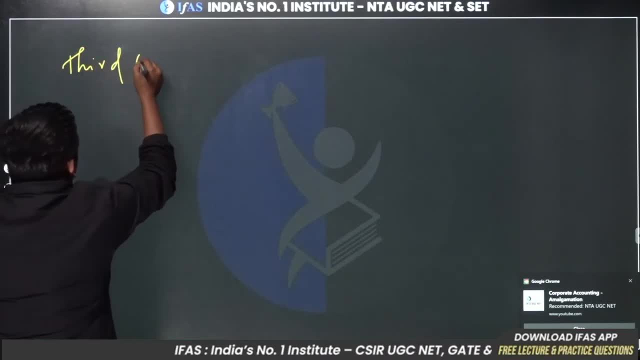 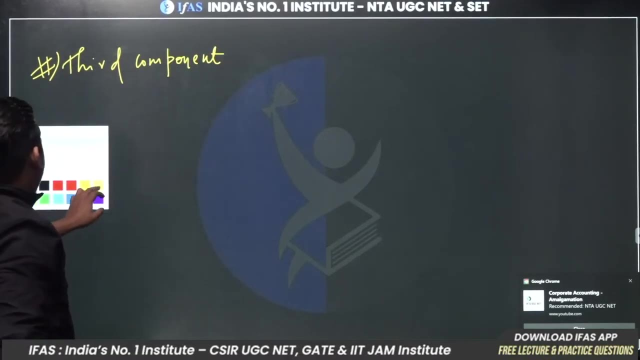 This is what happened on iso spin. 4 likes are left Quickly do 50.. Now let's talk about the third component. Now let's talk about the third component. See the third component. Did I talk about pions? 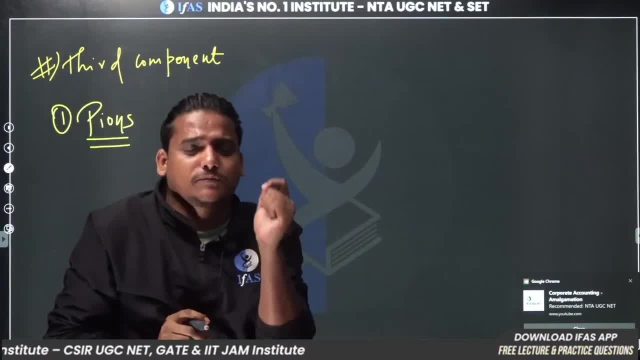 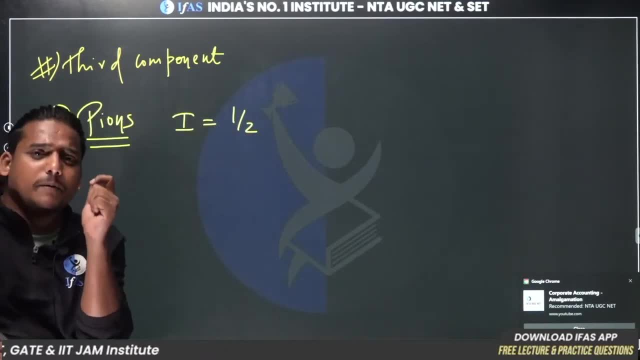 What did I say? The third component will take the values from minus i to i. Now, what was i for pions? What was i 1 by 2.. So tell me in the comment section What will be the values of the third component here? 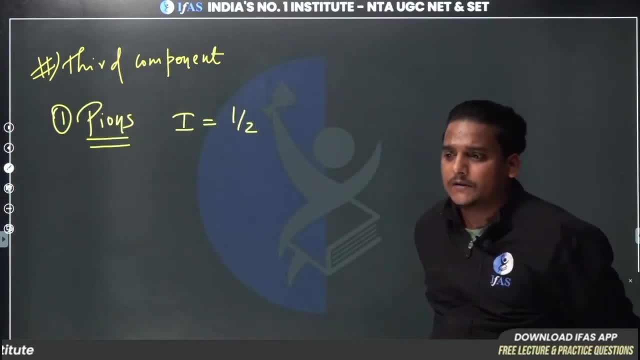 Tell me in the comment section What will be the values of the third component here. Hello, good evening. If i is 1 by 2, then what will be the values of the third component here? If i is 1 by 2,, then what will be the values of the third component here? 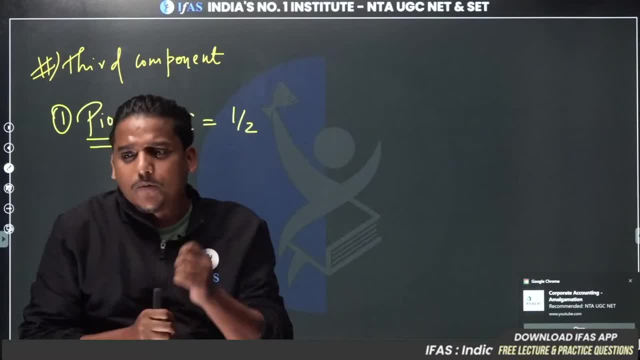 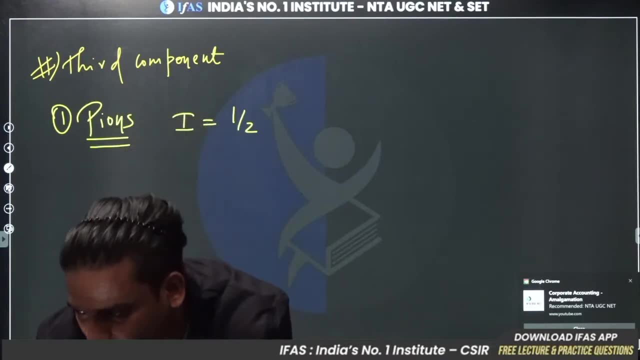 If i is 1 by 2, then what will be the values of the third component here? Tell me in the comment section, Because 3rd component take the values from minus i to i in stage of 1.. These are basics that you have to tell me. 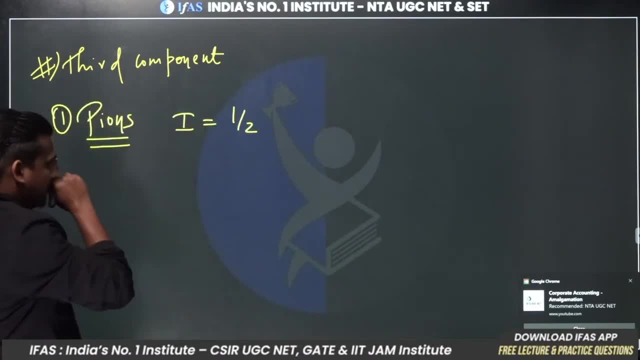 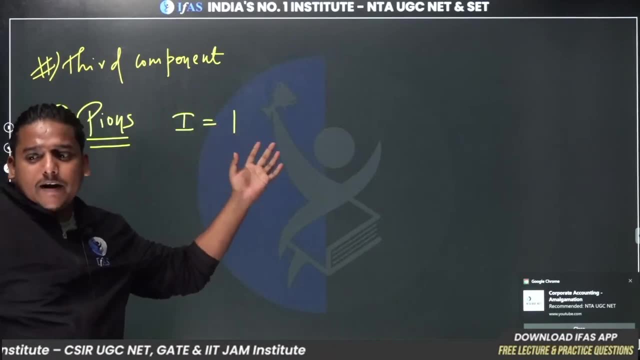 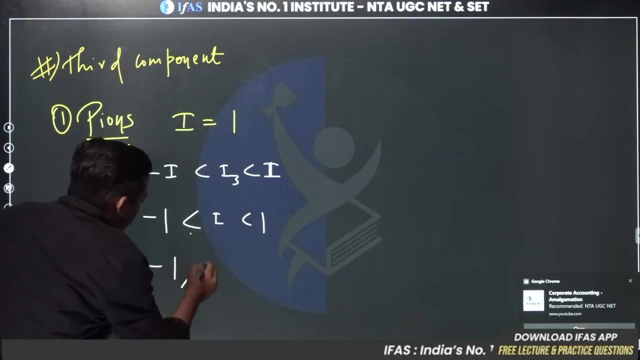 1 for pions. Let's see, Sorry, it is 1.. Fine, sorry, It is 1.. tell me what will come here in the third component. it is wrong. do your own right. they did right to me, don't make a mistake. from minus i3 to i. i3, which is from i to i, from minus i, so it is 1, so from minus 1 to where what will happen here? tell me: minus 1,, 0,, 1, you will get these three values here: i3, these three values here, you will get i3, is it clear. 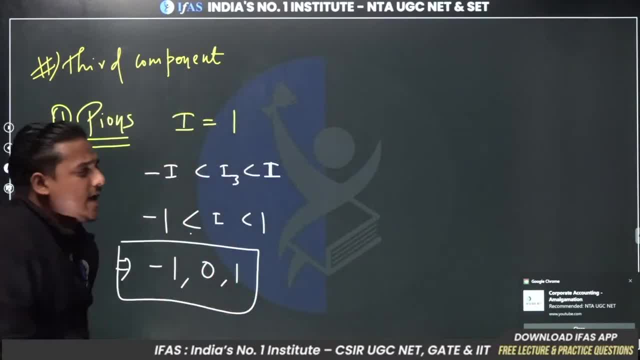 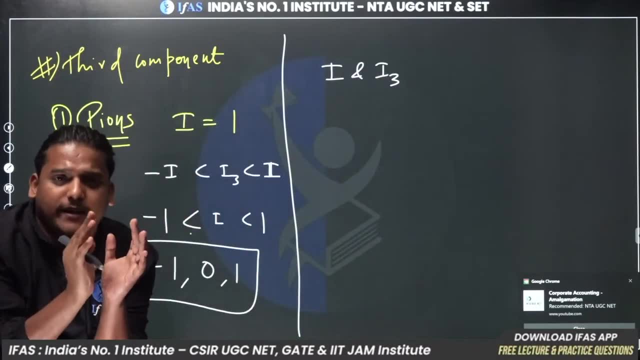 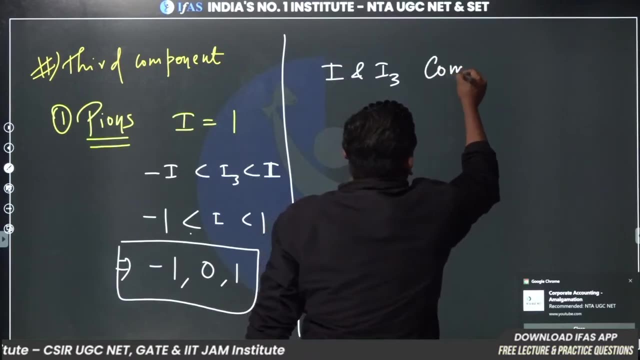 You have three values, but how will these three values be defined? always keep one thing in mind, which is i, which is i, i and i3, both combine to define one state. read: i and i3 combine to define state. how? 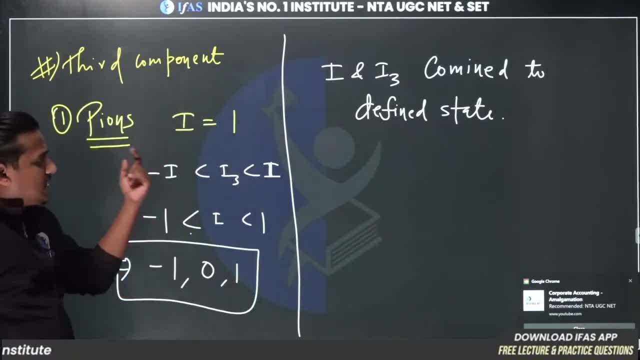 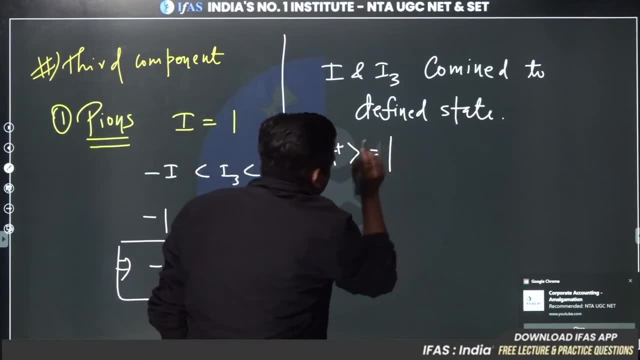 See now see in pions: pi plus, pi minus, pi zero. If I want to define the state of pi plus, then how will I write? Always, keep in mind how you will write the state First i, then its third component. 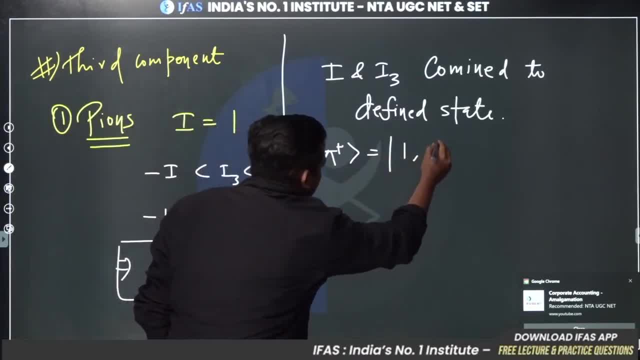 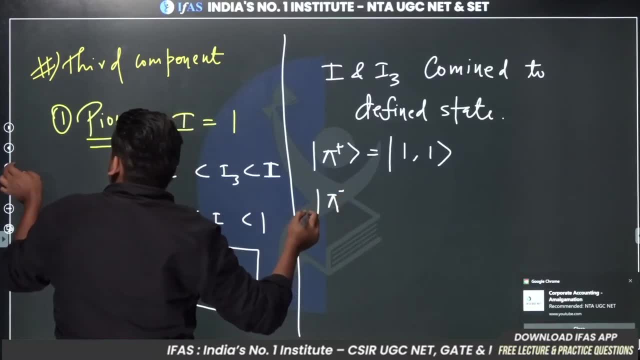 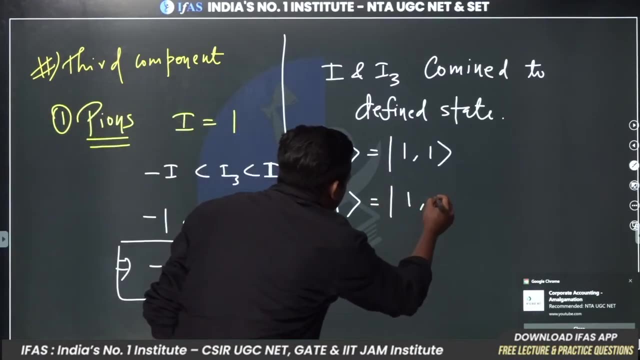 So i is 1, and its third component will come here: 1.. This is your state. If I want to write pi minus, then you can do it automatically. for the rest of the things, Here will come 1 and minus 1.. 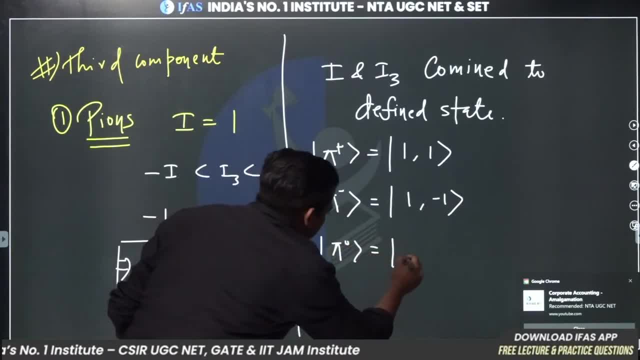 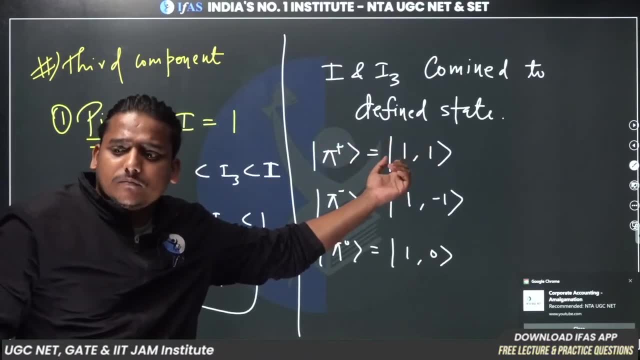 And if I want to write pi 0, then here will come 1 and minus 0. So this i and i3 both define a state. Is this clear? If anyone has any doubt, any problem, any doubt, tell me in the comment section. 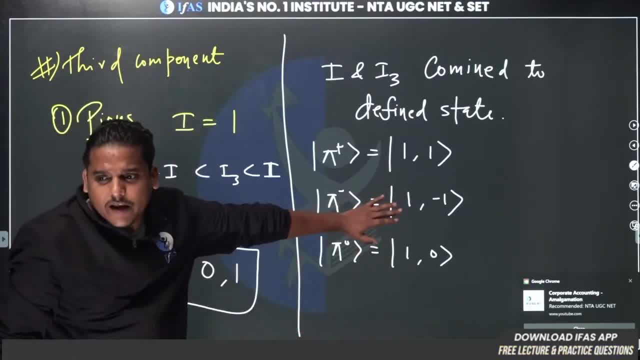 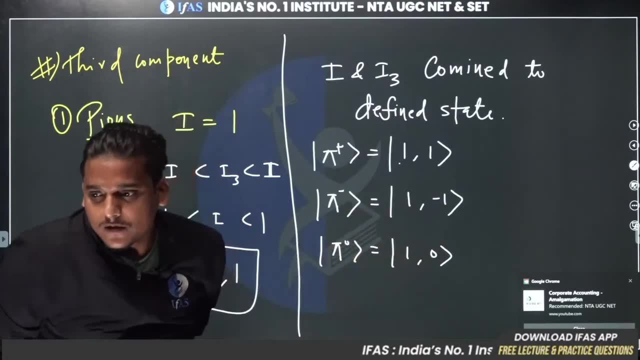 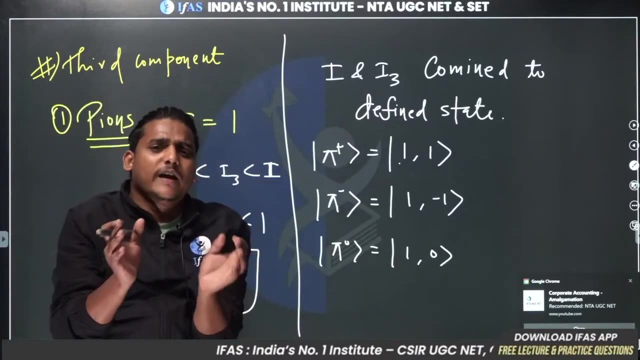 Very good, very good, perfect. Now, how do you write? No one should have any doubt in this: 1, i and i3, i and i3,, i and i3.. Iso is just a quantum number. This is a quantum number which is defined by particles. 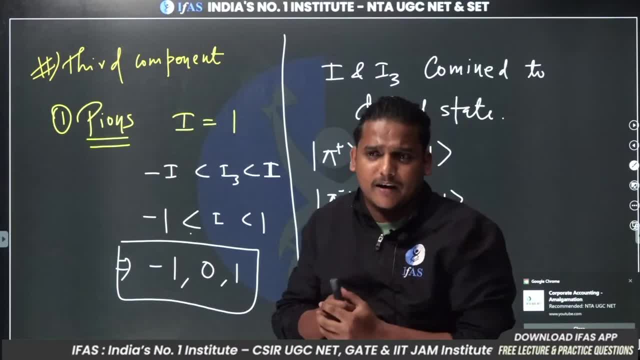 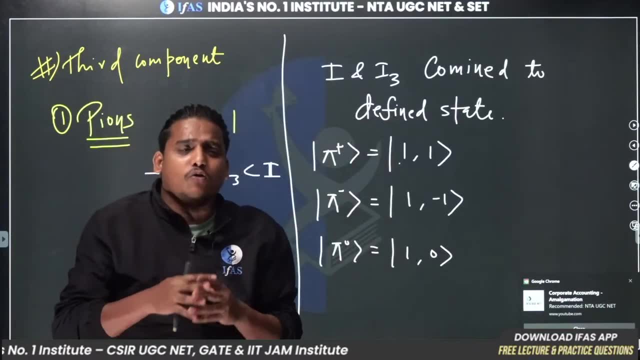 Such particles which participate in strong interactions, like hydrons. Basically you can say it like this: There are neutrons and protons in a strong interaction. You don't know the difference between them, So to differentiate between them, a quantum number has been defined: iso spin right. 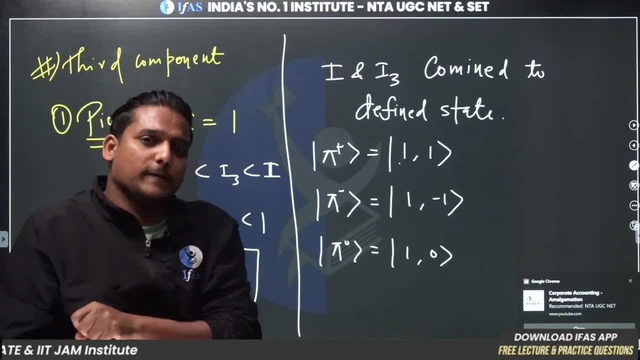 It has no such physical significance. These are all quantum numbers. These are all quantum numbers. These are all quantum numbers. Now you will read in yesterday's lecture: strangeness, Strangeness. Now you will ask: sir, what is this strangeness? 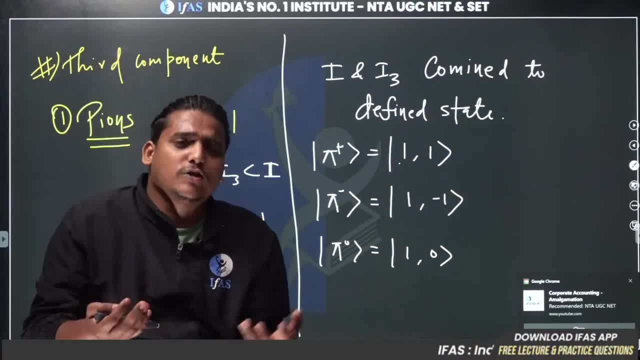 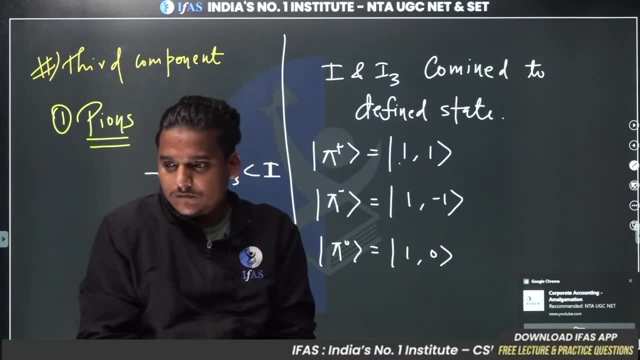 It is a number. It has been defined quantum number to define the properties of some particles. Is this clear, Clear, What can you do in this way? You can find it for doublet. You can find it for doublet. 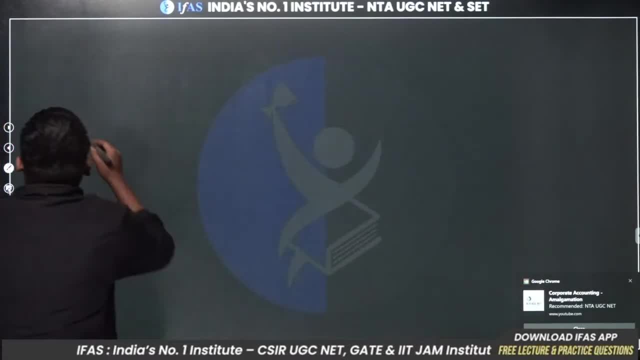 If you do one more and tell me, then you can do the rest yourself. Okay, son, Like, Like kions, Like kions, Like kions. You know kions right? This is it right. And for doublet, what did we find in iso spin? 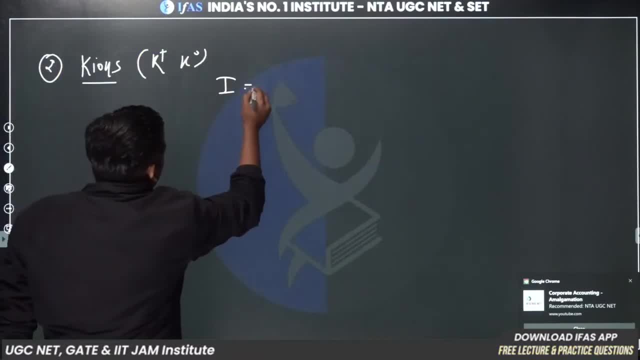 1 by 2, right. What is your i for doublet 1 by 2.. So tell me here in the comment section what will be the value of i3?. Tell me in the comment section what will be the value of i3?. 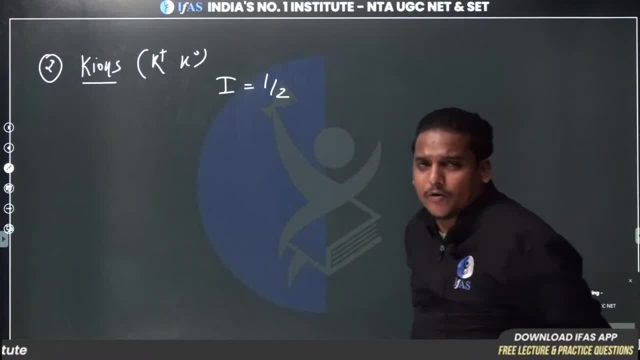 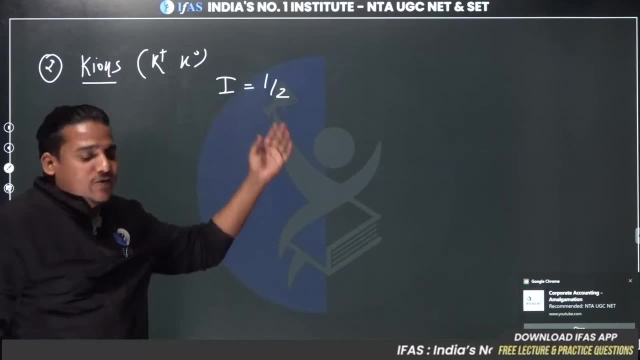 Tell me in the comment section what will be the value of i3?? You should know how to find it. it is basic. It is basic With a good math. What will be the values of i3 if you have i1 by 2?? 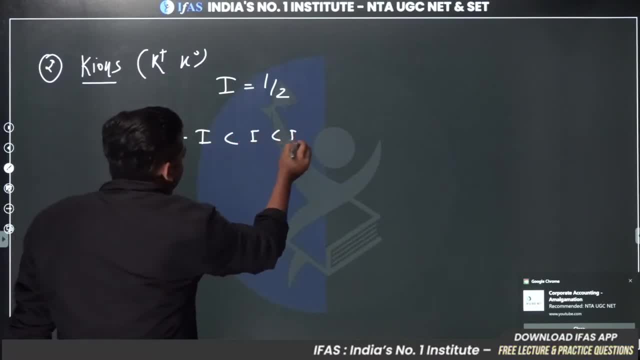 From where? From minus i to i2.. From minus i to i2.. From minus i to i2 in the steps of 1.. Tell me quickly so that I can write here: 1 by 2 minus 1 by 2.. 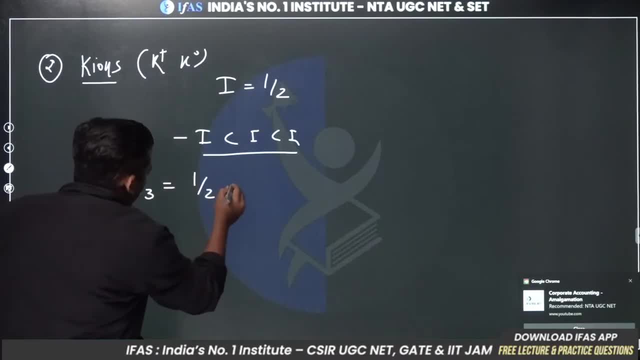 Very good, Perfect. The value of i3 will come here. that is, 1 by 2 and minus 1 by 2.. So how will you define the state? So k plus 1 state will be there. You will write the corresponding of k plus. 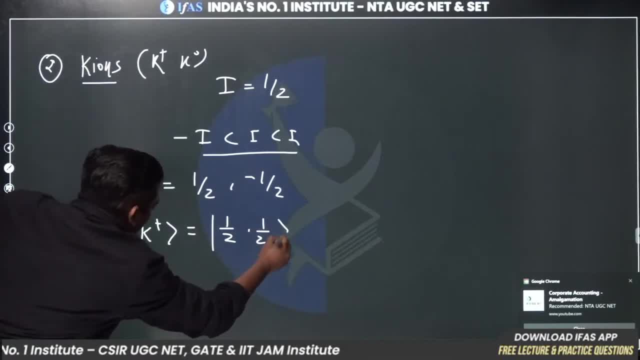 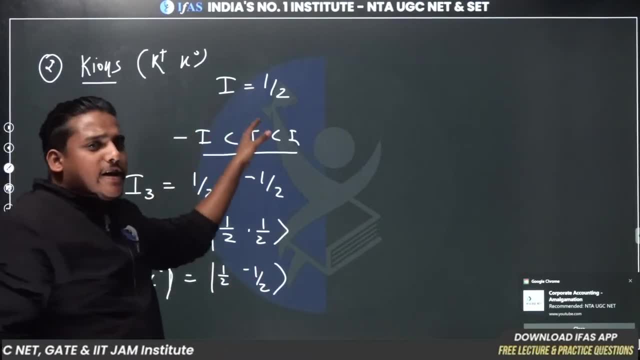 So the value of i is 1 by 2 and here 1 by 2.. And what will happen for k0? here 1 by 2.. Simple, So in this way you can easily remove the third component of i and iso spin. 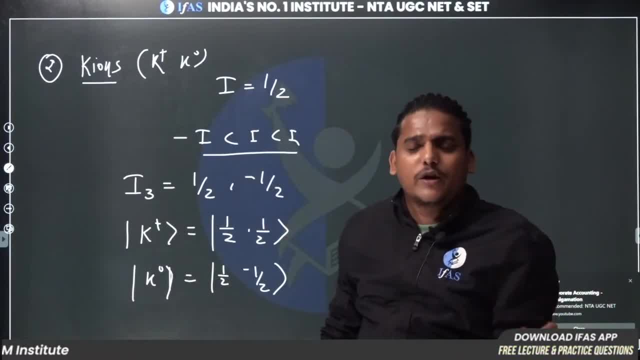 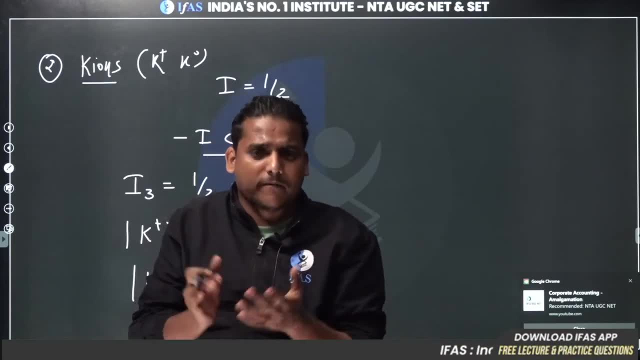 Is this clear. If anyone has any doubt, any problem, any problem. any doubt, Take care. for triplet iso spin is 1.. For doublet iso spin is 1 by 2. And for singlet iso spin is 0.. 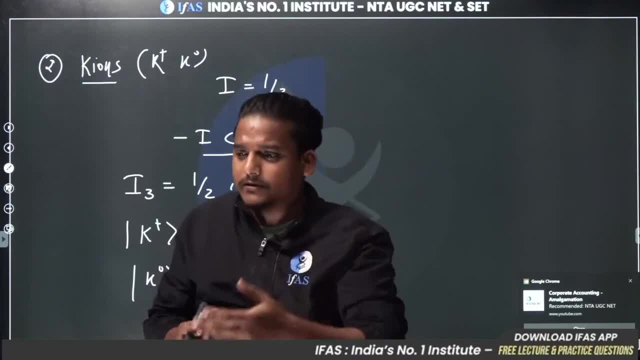 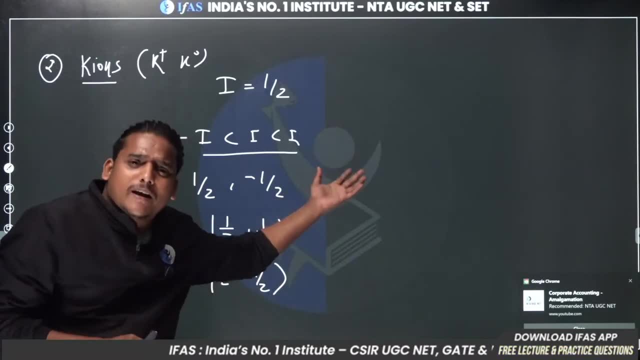 Third component: from minus i to i in the steps of 1.. Simple, Easy. Now let's talk about its importance, Sir, why are you telling What will help in its numericals, Sir? how will my number come, Sir, how will my question be solved? 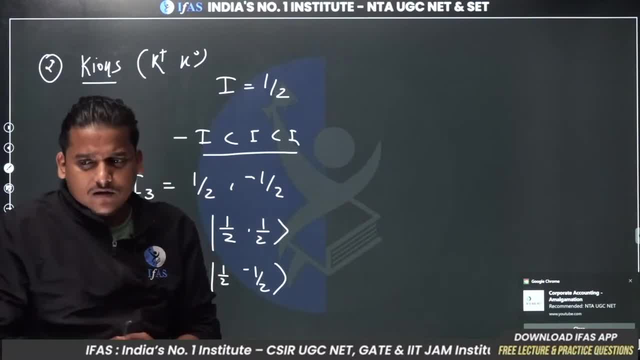 Sir, tell me about the topic. Sir, tell me about the topic. How will it help in the questions, Sir? how will it help in the questions, Sir? how will it help in the questions? Let's talk about the topic. 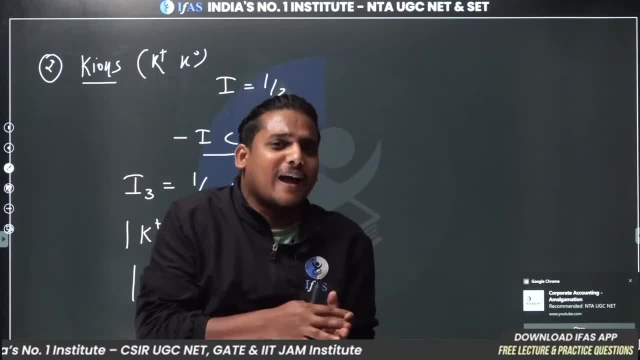 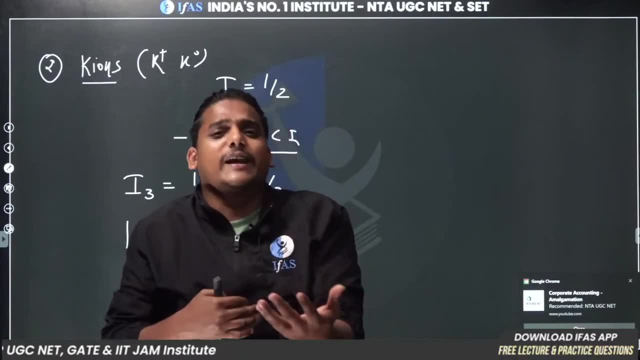 Iso spin conservation is going to tell you which type of interaction is allowed. If it is forbidden, Which interaction is going on? reaction: Is it going on with strong interaction? Is it going on with big interaction? Is it going on with EM interaction? 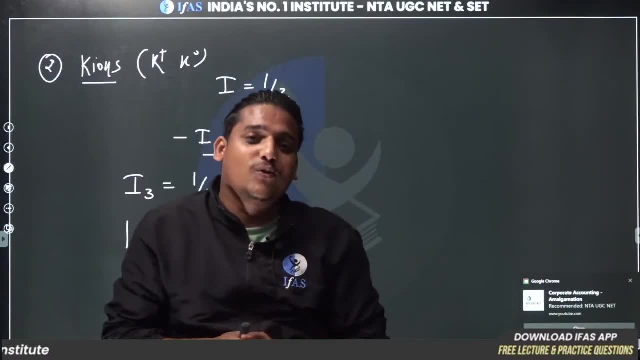 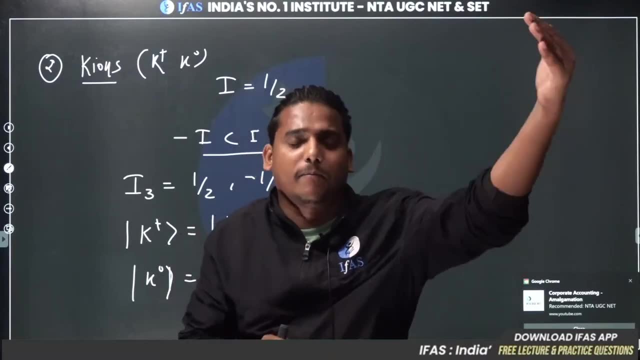 Is it clear. Today I will not discuss its strength, because its lecture is available tomorrow. Okay, I have divided each and every lecture so that you can study it slowly. Okay, Dheere, dheere, achche se padh pahun. Now see how it is used. 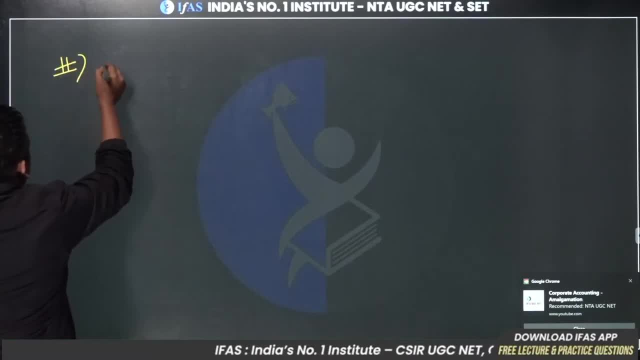 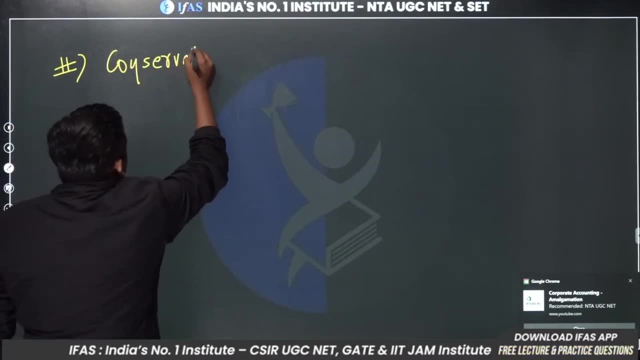 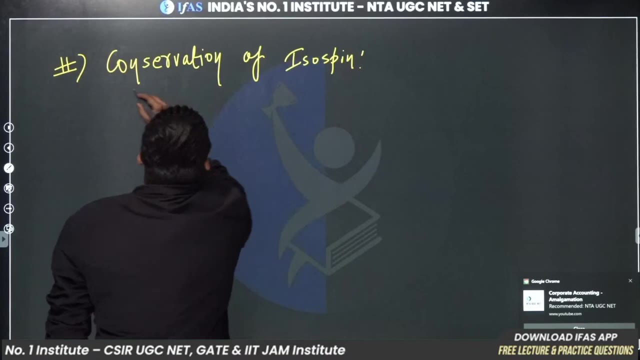 This is an important parameter. Conservation of isospin: Now I will also tell you about resonance particles. Patience, Conservation of isospin is important. Conservation of isospin. Conservation of isospin is the most important point of today's lecture. 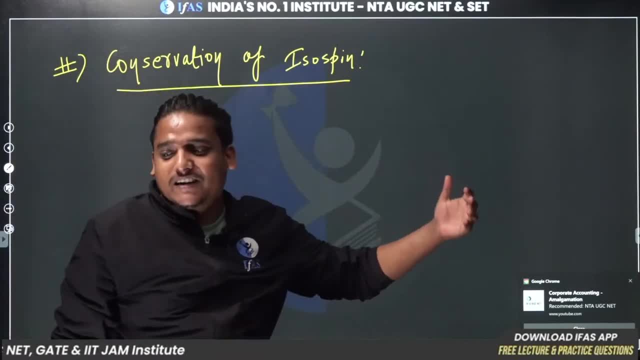 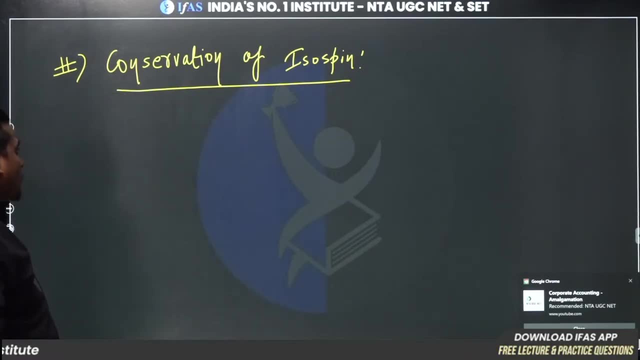 Which will give you questions in CSI or NET exam or GATE exam And will give you marks. Now see Conservation of isospin. How will we use it? Suppose you have 1 plus 2. Because children don't know how to use it. 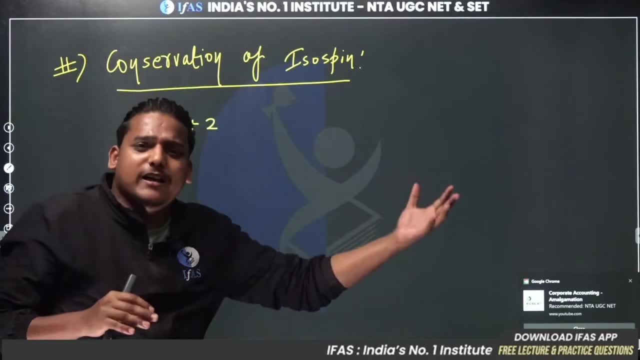 They know that if there is B contraction Then in B contraction I will not be conserved. I3 will also not be conserved. But actually they are not able to add in the reaction And they make a mistake there. Understand this carefully. 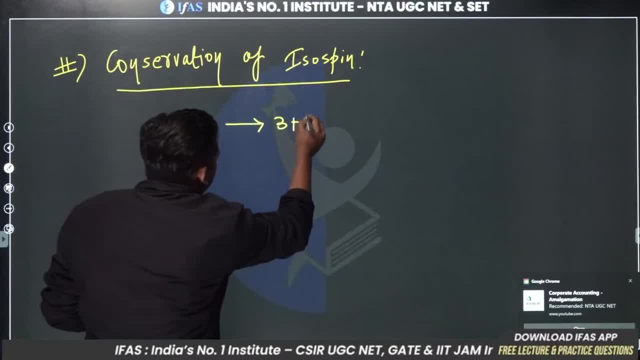 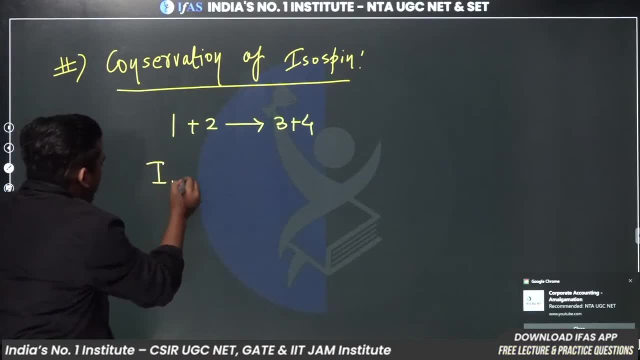 If you have a reaction 1 plus 2. Gives us 3 plus 4.. Right, Suppose there is a reaction like this, For example, And I will tell you that I1's isospin is I1. And 2's isospin is I2.. 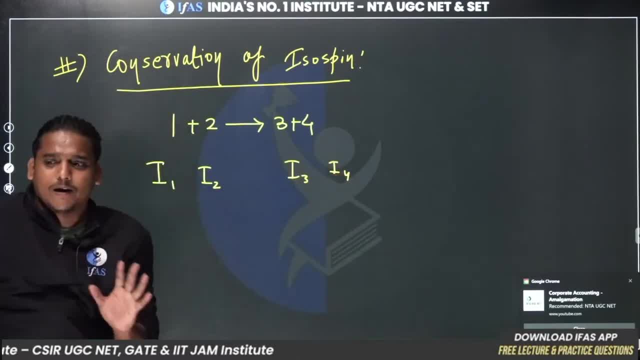 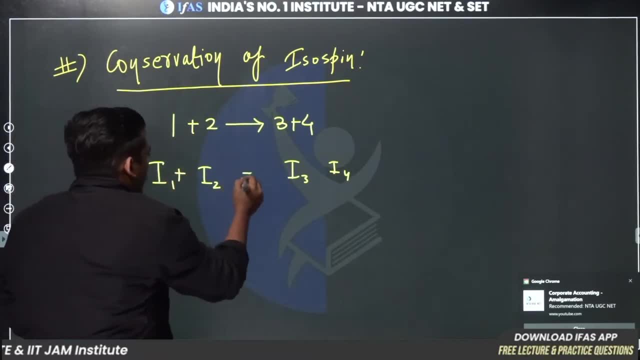 3's isospin is I3.. 4's isospin is I4.. For example, I have said this: Okay, If Bacterially. Now what will you do in this? also Inca Bacter? Okay, 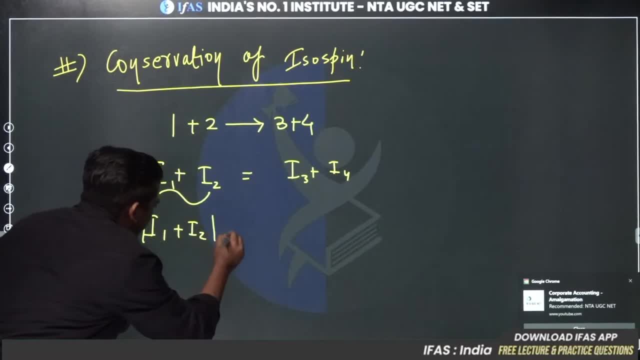 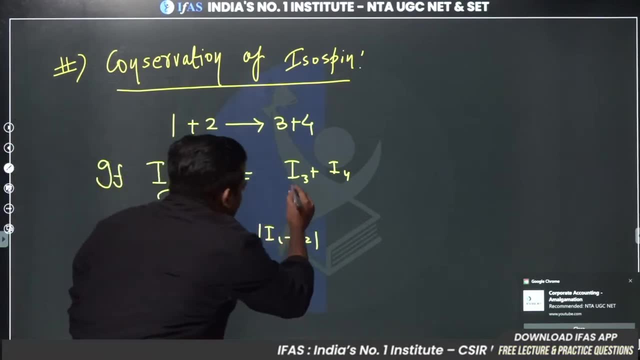 From I1.. Understand this carefully. From I1 plus I2.. What will be its value? I1 minus I2.. Understand this carefully. There will be no mistake. Understand this carefully. Ask doubts later. This Like this here: 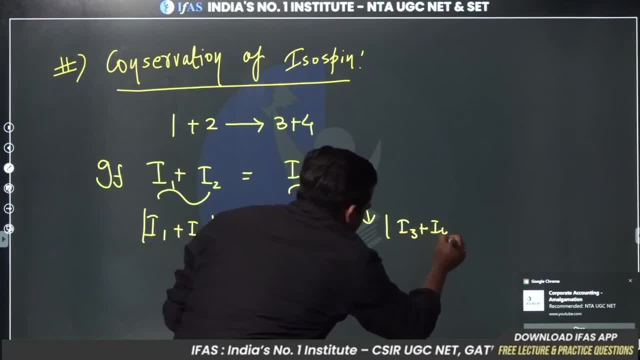 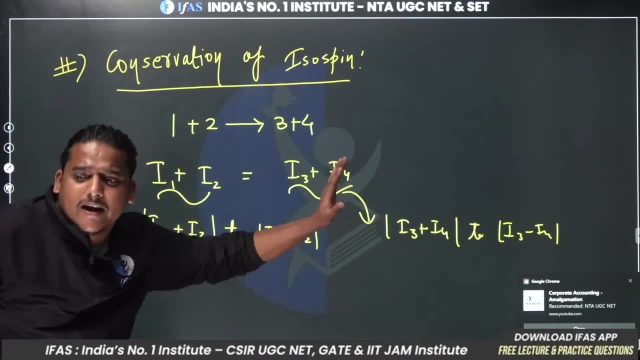 Where will you get its value? From I3 plus I4. I1.. I3 minus I4.. So when will you be able to say that isospin is conserved or not? Understand this carefully. If, in this scenario, All the values you will get, 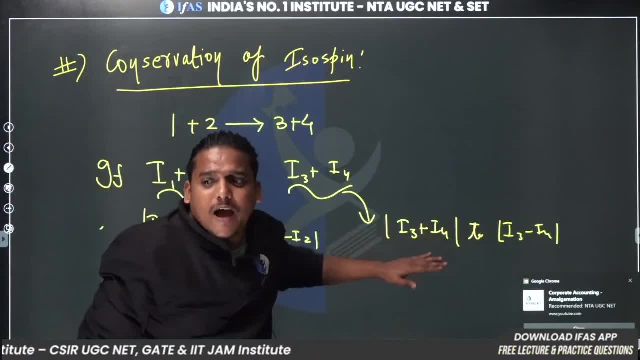 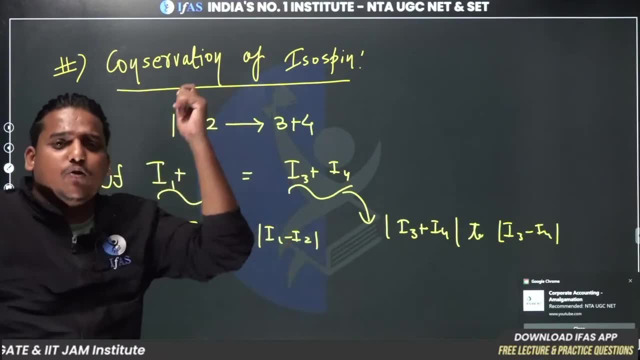 You will get multiple values here And in the scenarios here You will get multiple values here. If you are getting any value in LHS and RHS, That means you can say your isospin is conserved. Point is clear or not. 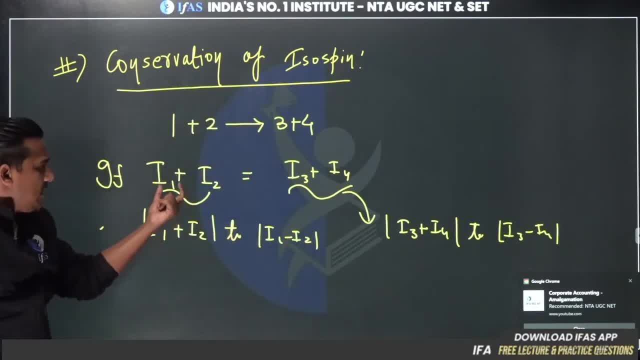 Is the point clear or not, What you have to do From I1 plus I2.. You will get values from I1 minus I2.. You will get a lot of values From I3 plus I4.. You will get a lot of values from I3 minus I4.. 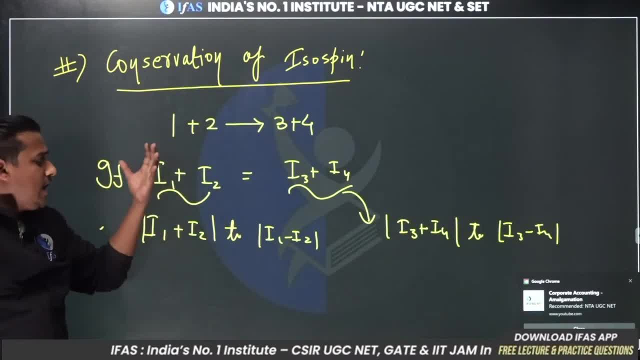 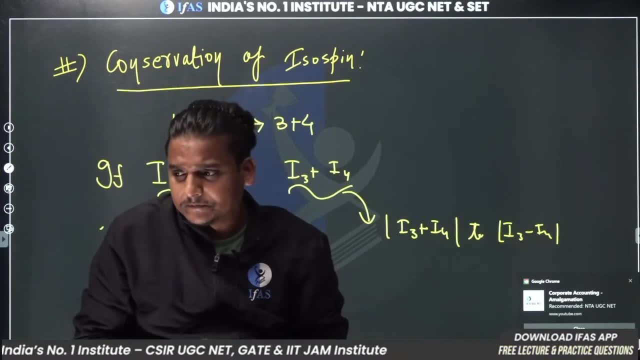 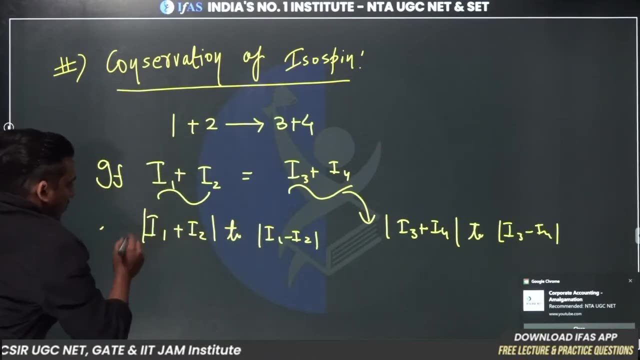 You just have to see here That any isospin, if you are getting in LHS and RHS, That means your isospin is conserved. Is this clear? So write here, If. If this. Write here, If Any value. 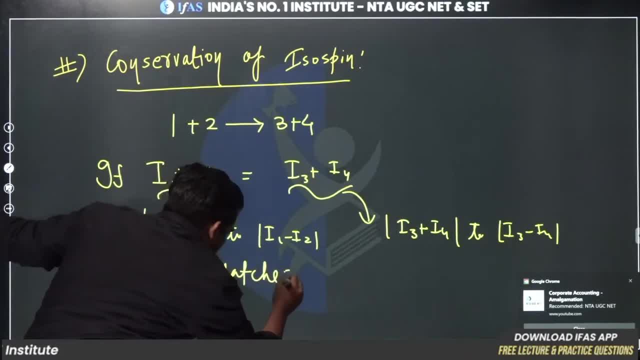 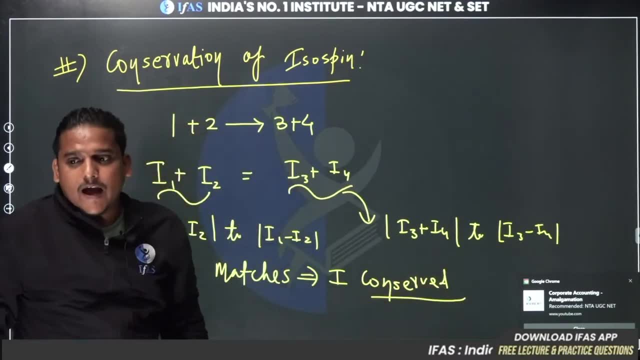 Any value matches. It implies that I conserved. I hope this is the motive to explain to you. That was the motive. I hope this is clear to you Because there is doubt. I also have doubts Because I learn from my mistakes. 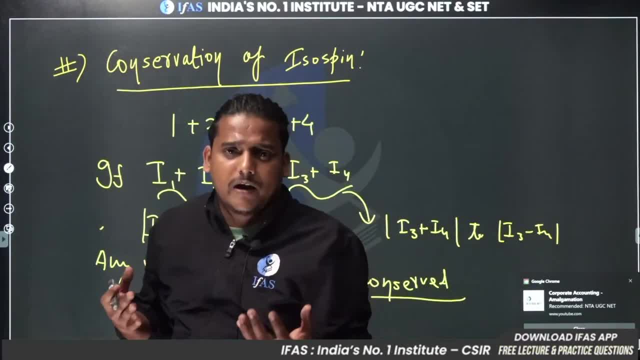 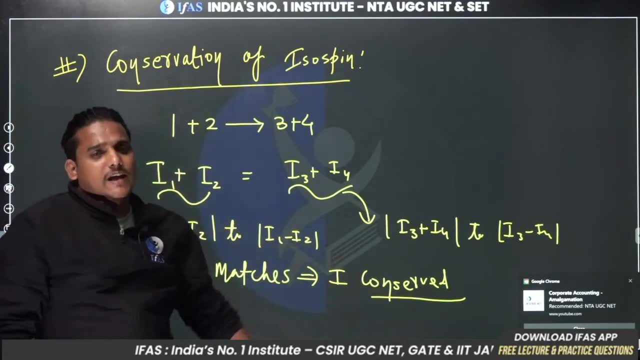 When I have doubts, Then I can also understand that we are all normal. You are people, So you must also have doubts in that thing. When I used to study in starting, Then I used to have a lot of problems here. You have to follow things like this. 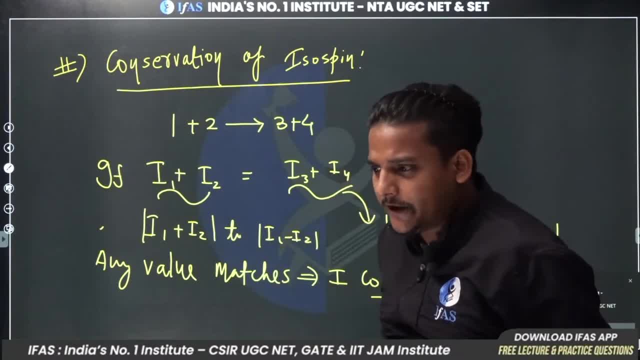 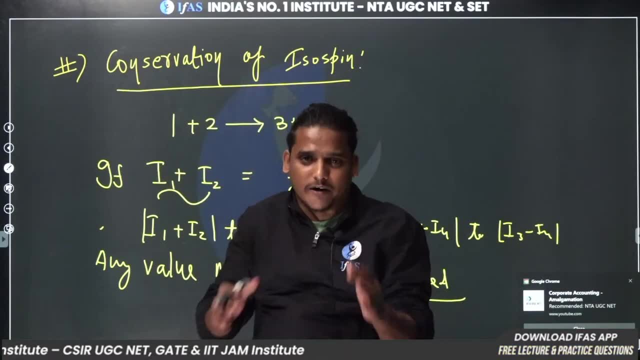 Is it clear? Is it clear? Naushreen Abru, Faraz, Udayraj, Avatar, Aarti, Are you enjoying the session? Tell me quickly. Is the session looking good? Are you getting some important information? Are you getting any useful information? 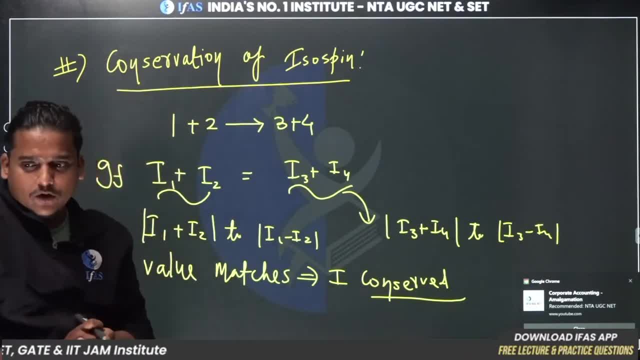 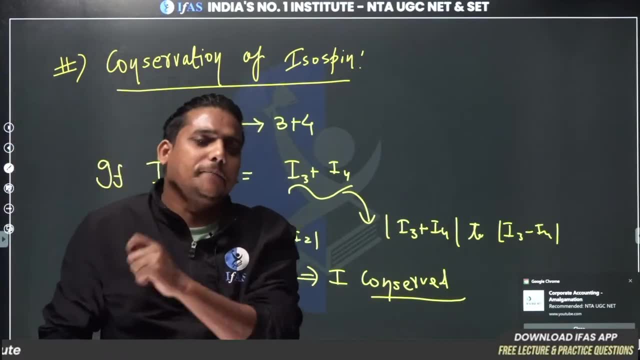 We are not talking much here and there. We are talking directly on the important points. Come on Now: In which interactions, in which things are conserved. We make a table on that Which will help you, For whom We will do numericals. 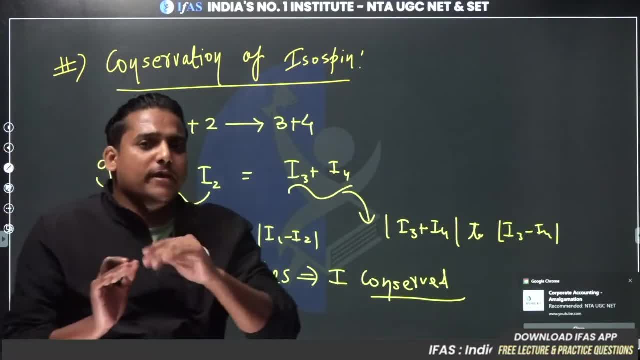 Don't worry, We will do numericals Now. we will define the whole. Now we will define the strangeness, Because the numericals will be with you. I, I3, Strangeness, All the things will be with you. 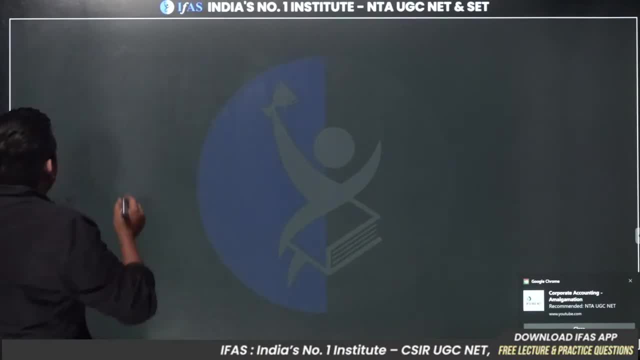 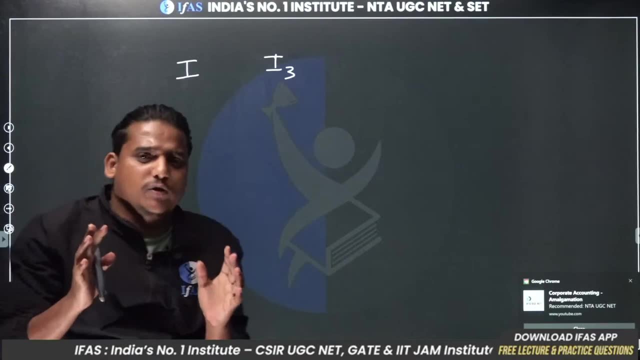 Okay, Come on. So you make a table here. Important A, A, A, A, A, A A. One is I And another one is I3.. Now, I haven't talked about the strangeness, dear students. 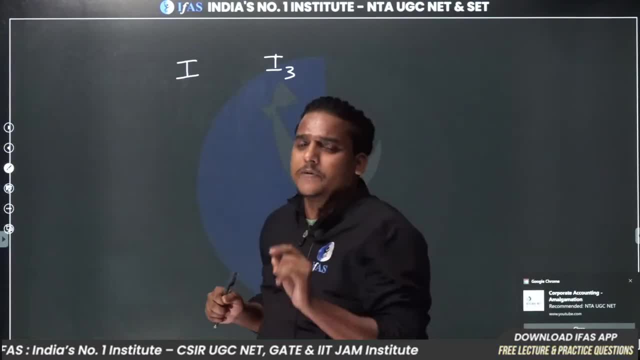 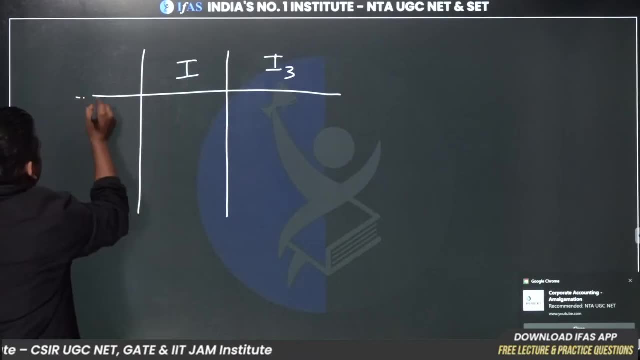 So I will not bring the strangeness here In tomorrow's lecture. we will also conserve the strangeness. we will talk about how and what. Now I am just talking about two, and here you should write Type of interaction. If you write strong here you have three types. 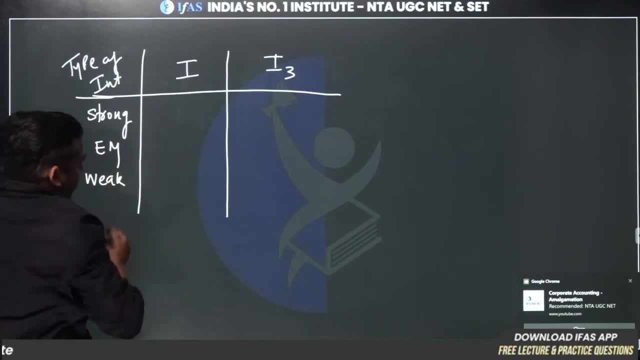 Em and big. So first of all, you have to keep in mind that if there is a B contraction, then I3 will not be conserved in it and I3 will not be conserved. Is it clear? If there is a B contraction, then I will not be conserved in it and I3 will not be conserved. Read Point to be noted. 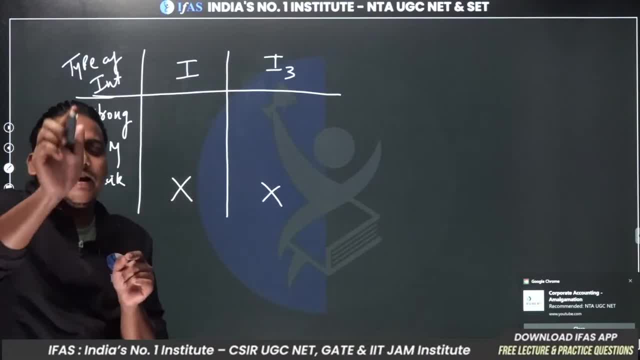 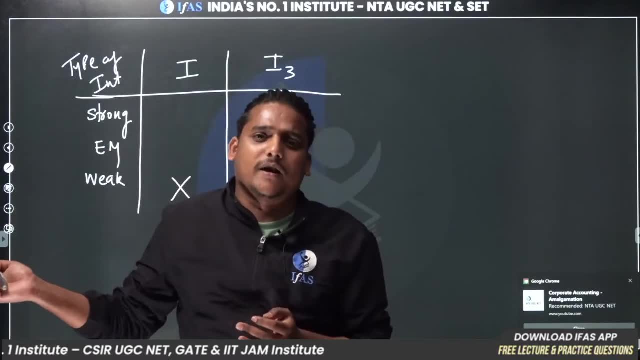 Now, when you read the cork model, you will get it out. Don't get tensed. You guys don't have patience. There is no patience. There is no patience. Look at the lectures ahead. There is one thing Strangeness: CPT rule, conservation laws. cork model part 1,. cork model part 2.. 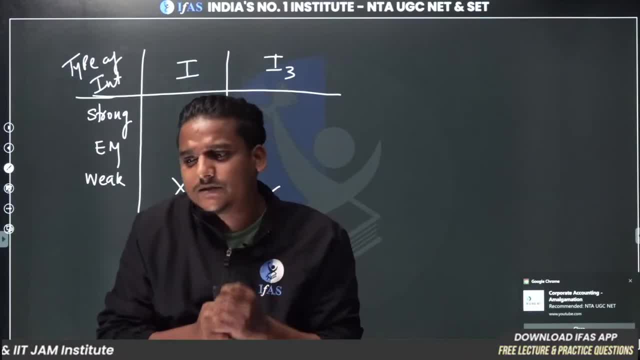 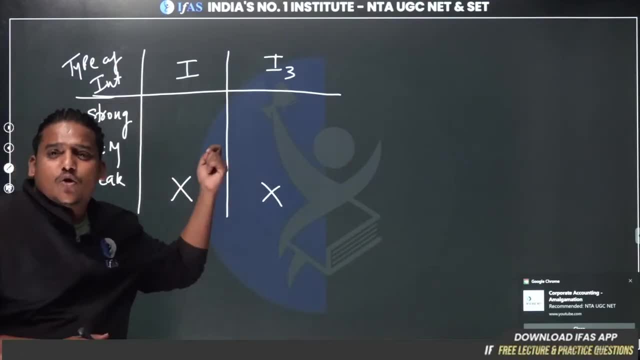 Learn with patience. Learn with patience. All the things will be told to you. Is it clear All the things that I am trying to say? So if you have a B contraction, then I will not be conserved and I3 will not be conserved. Point to be noted. 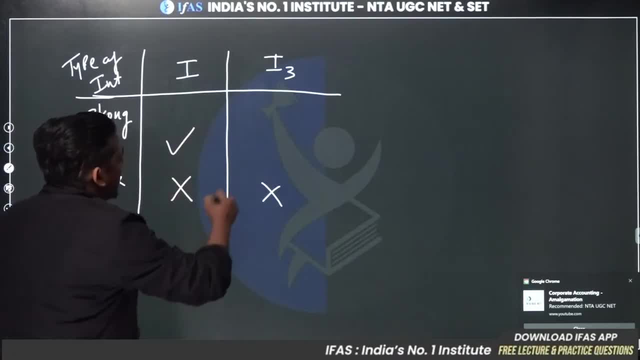 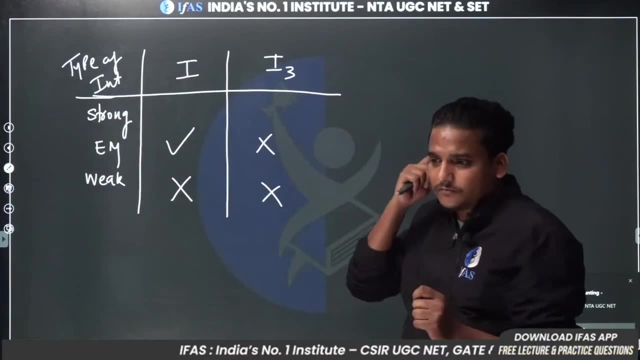 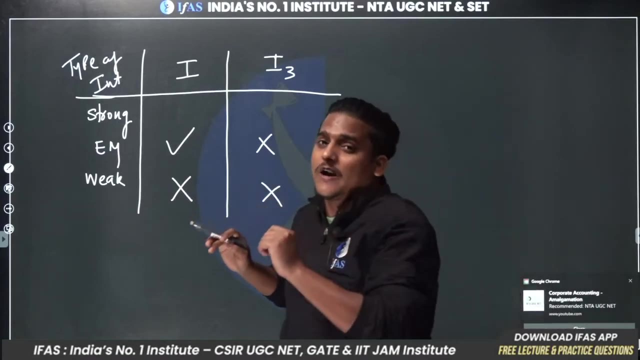 If you have an EM contraction, then in the EM contraction I will be conserved, but I3 will not be conserved. Is it clear? If you have an EM contraction, then in the EM contraction I will not be conserved, but if there is a strong contraction, then in the strong contraction both of you will be conserved, whether it is I or I3.. 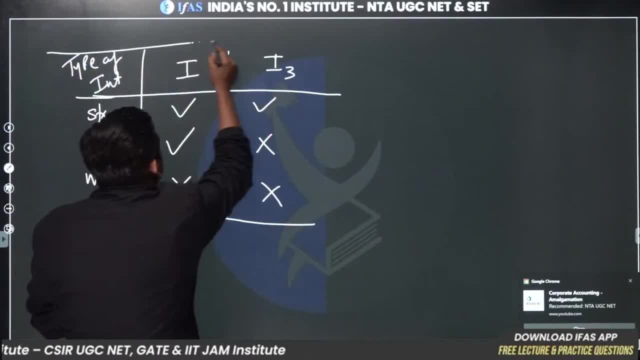 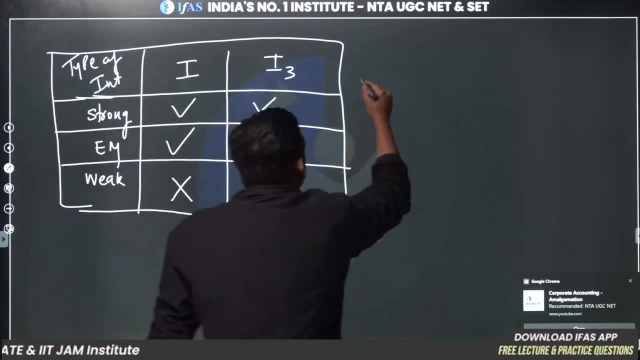 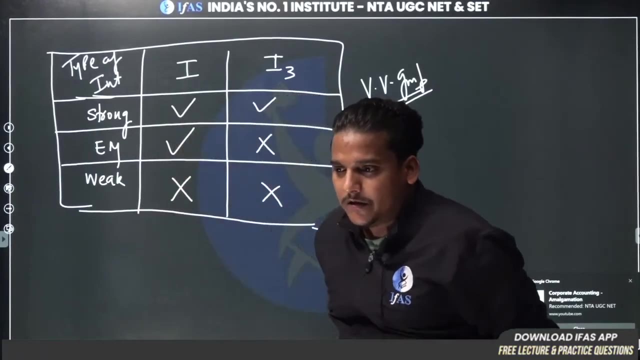 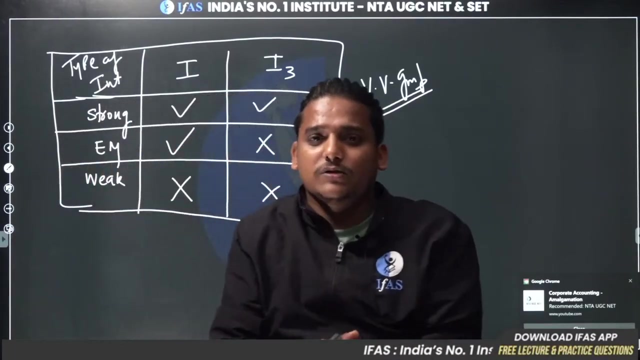 This is a very important point that will help you in your questions to identify the type of contraction in reaction. Is it clear? If you are liking the session, then keep liking the session. right, my brother? Keep liking the session. Give a like to the button with which you scroll through the reels. 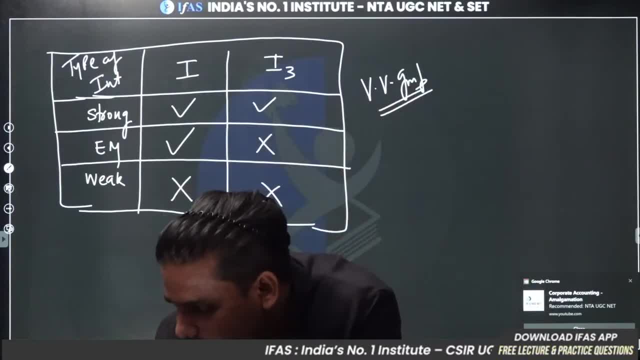 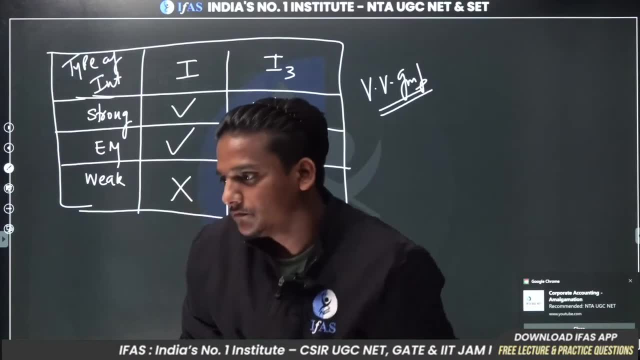 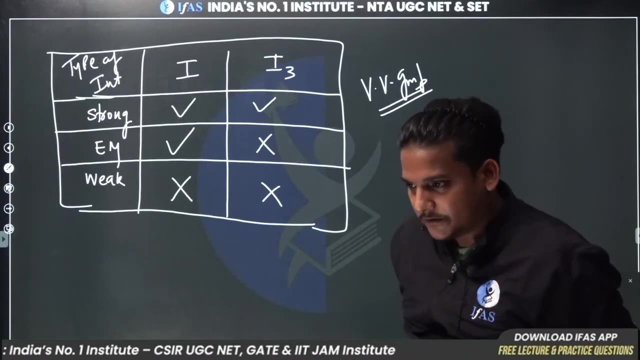 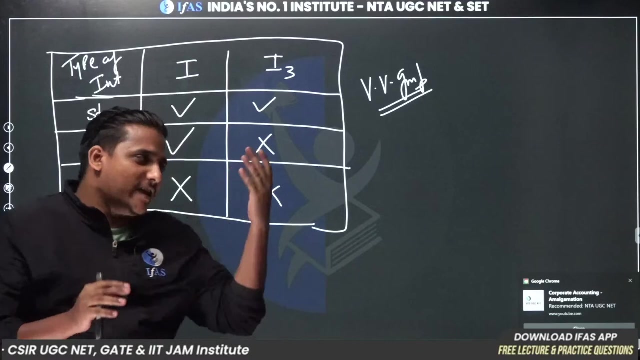 Come on, Is it clear? Is it clear? Are you enjoying the session? Are you getting all the important things? Are all the concepts clear so far? This was the most important concept of today's session, which will help you in numericals. 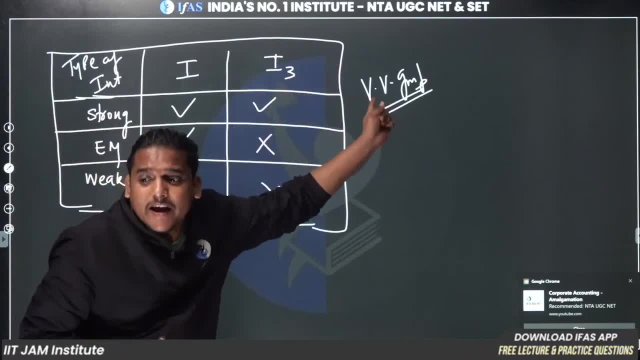 I hope you have printed this In front of this. in tomorrow's lecture, one more column will be added. The column of strangeness will be added. Why am I not adding today? Because I have put the lecture of yesterday on it. 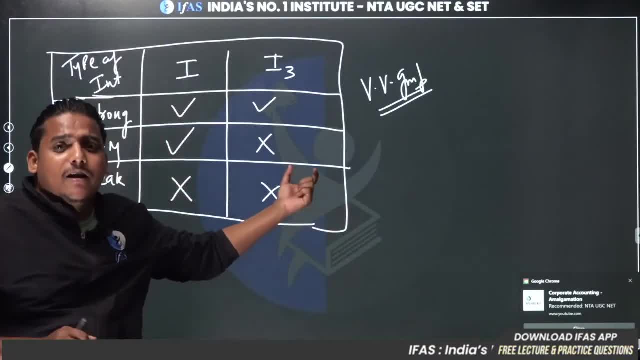 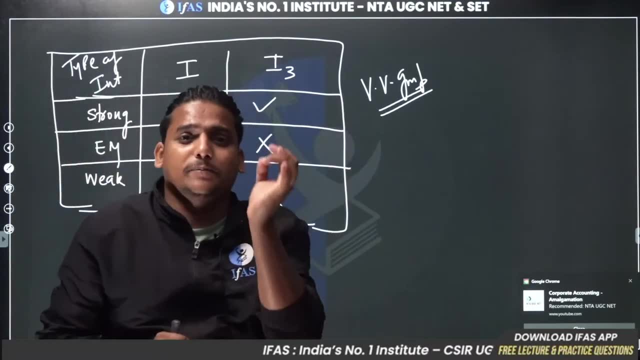 In that we will talk about how strangeness will help us in telling the type of interactions. Tomorrow we will add one more column on it, after understanding the strangeness. Now we will talk about the important topics: Resonance Particles. 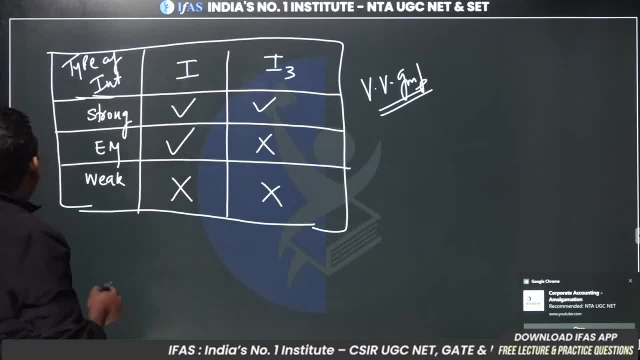 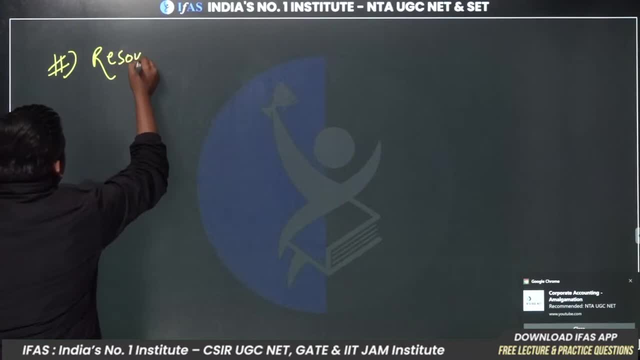 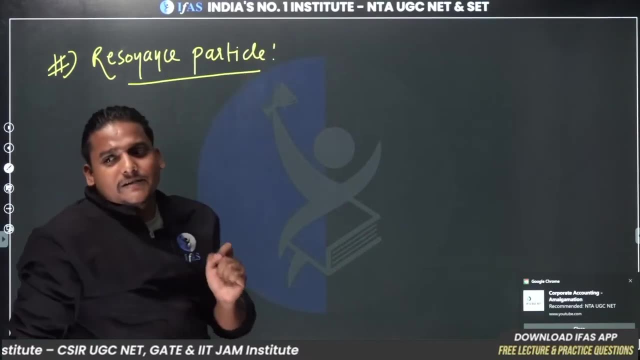 We will talk about resonance particles. What are resonance particles? Let's understand it a little basic. If any student knows, then tell me in the comment section what is resonance particles? How do you define resonance particles? It doesn't matter if any student is wrong or wrong. 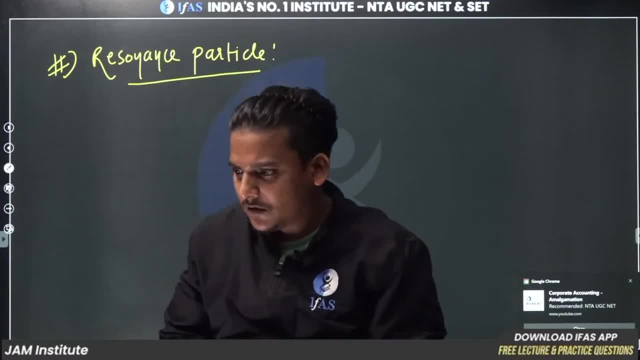 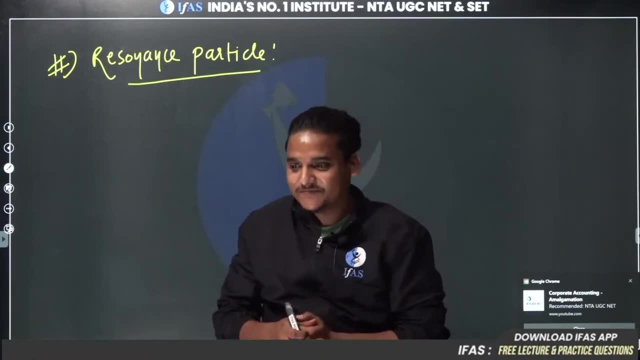 Answer me in the comment section. What are resonance particles? When you do the questions, you will know that I am a conservative and Y3 is a non-conservative. You will get to know that, Don't worry. Tell me who knows about resonance particles. 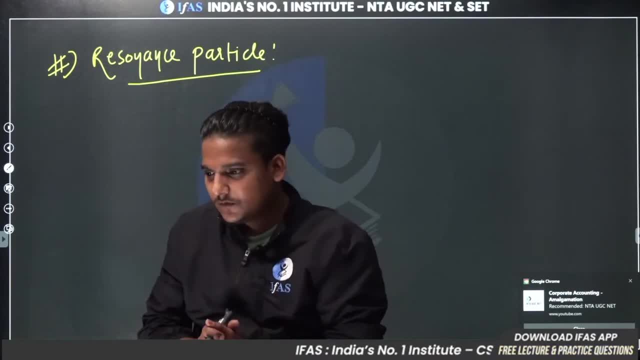 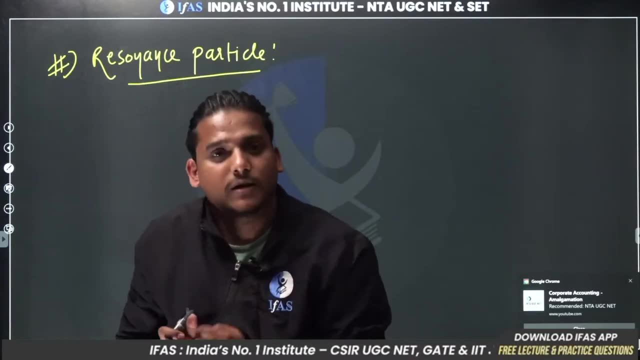 What is resonance particle? The particulum, Actually short-lived, That is correct, Very good, Short-lived, Very good, You said a very good thing. Let's define it in the basics. Actually, the resonance particles, What is resonance particles? 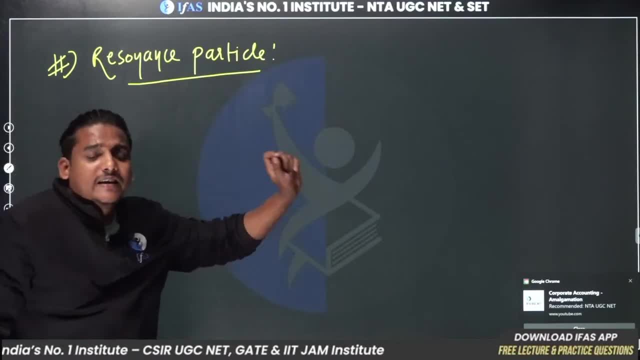 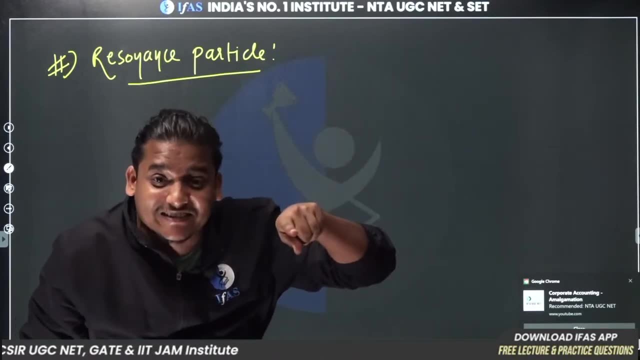 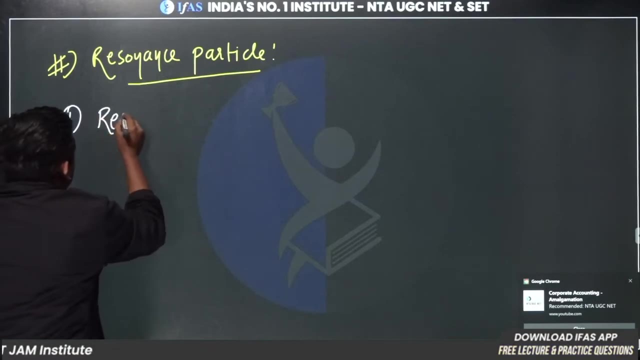 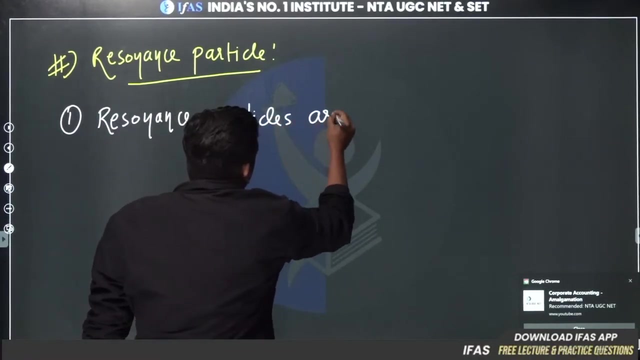 What is resonance particles? Well, the resonance particle, The resonance particles, are the excited states of the known particles. That is��는 far stairs komplete The emotions of the particles. There is no beginning or end. This is the start of the continuous change of the particles. 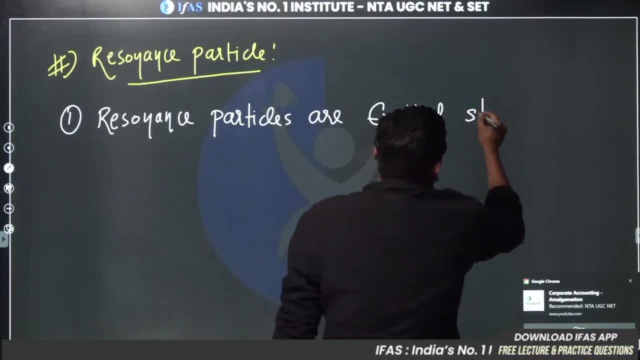 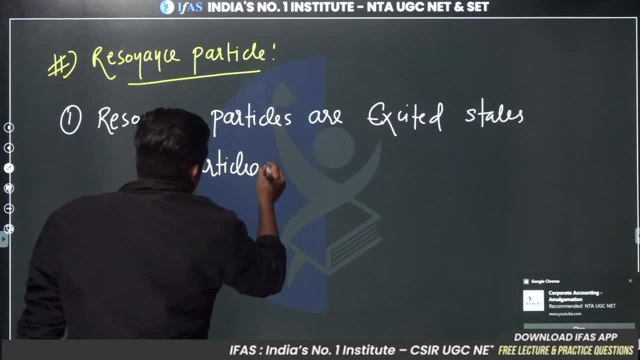 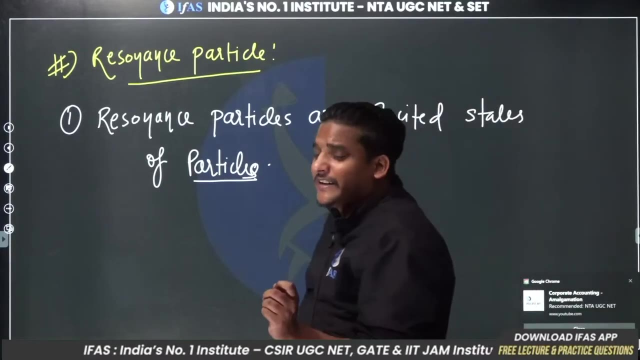 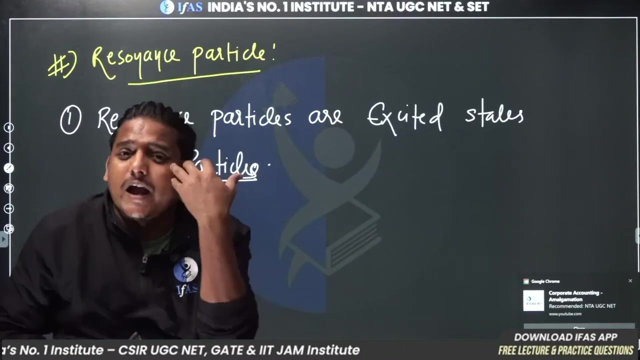 Excellent incentives, Perfect, Excellent of particles. these are the excited states of particles. now, the first point. is it clear, Sir? second important point: what information are the excited states giving to us? the excited states of particles are existing. what information I am getting from it is the most important. 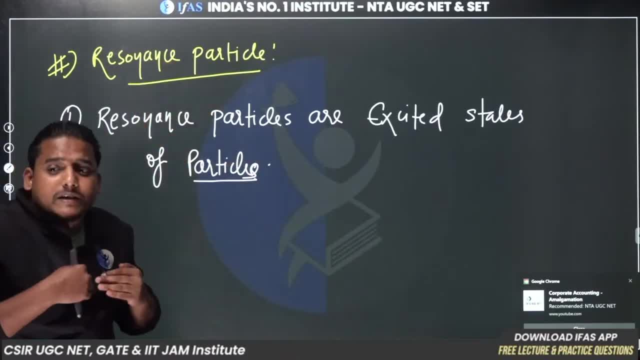 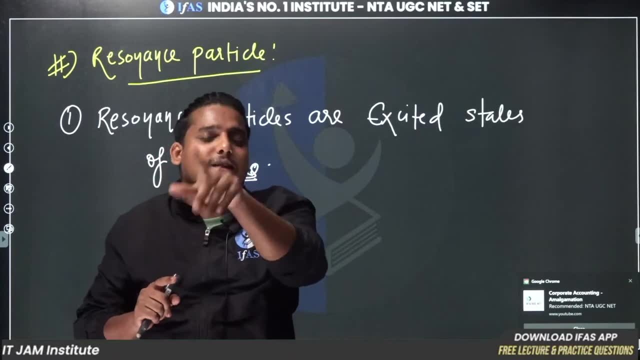 point that if I have a resonance particle, that means it is the excited state of some particles. and if the excited state of any particle is existing, then what information is it giving? let's talk about it. see, keep in mind that the excited state of a resonance 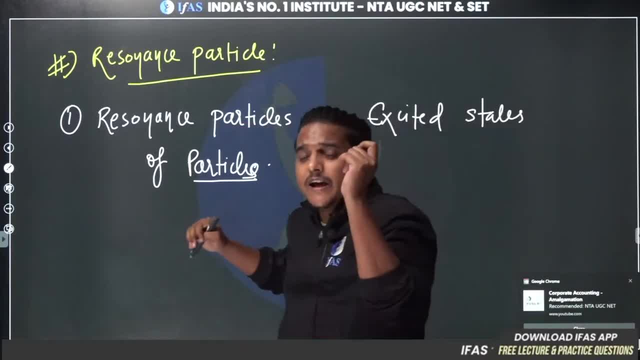 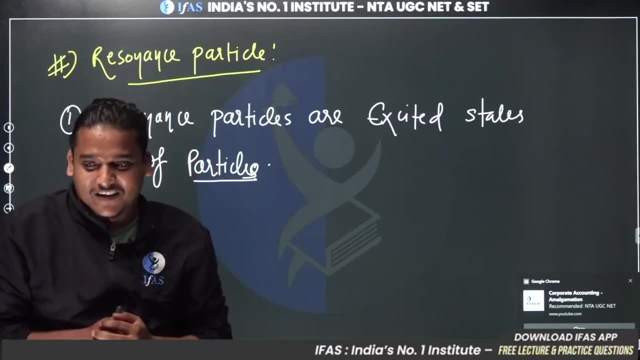 particle or any particle is existing. it gives us the information about the internal structure of the particle. is this thing clear? it is a very important point. keep noting: the excited state of the particles tells us about its internal structures. that, yes, that particle. 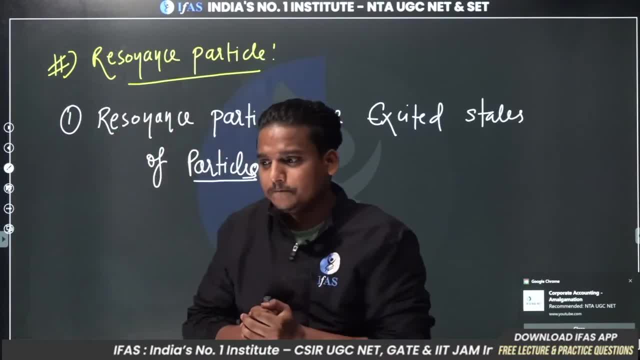 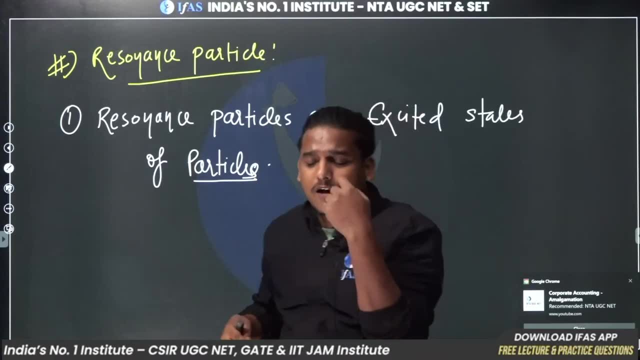 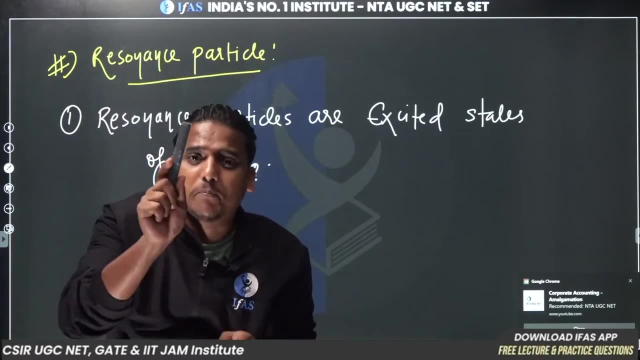 will have some internal structures. is this thing clear? Good evening Sochita. as you know, the excited state of a nucleon exists. with this, you can give an evidence that the internal structure of a nucleon is there and you know that the 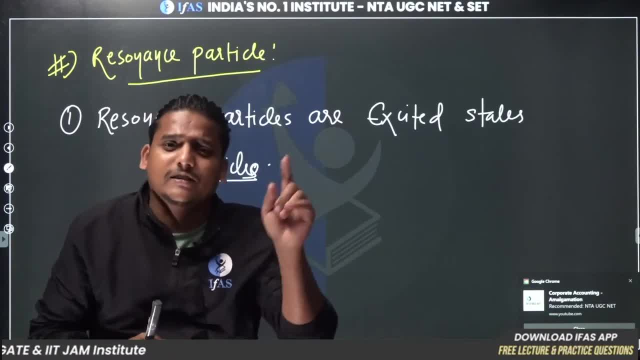 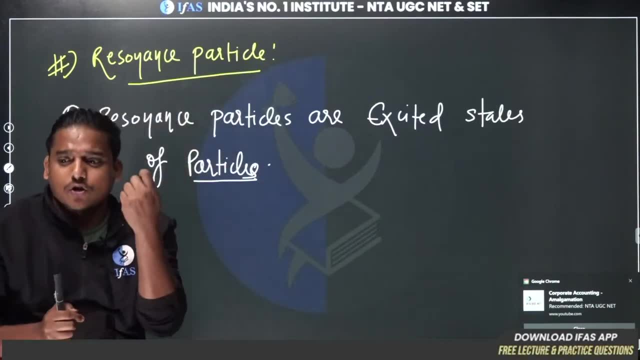 internal structure of a neutron is there. the internal structure of a proton is there. they are not structuralized particles. they have their own internal structures. they are made up of quarks. right, the protons or neutrons are made up of quarks. and who is giving the? 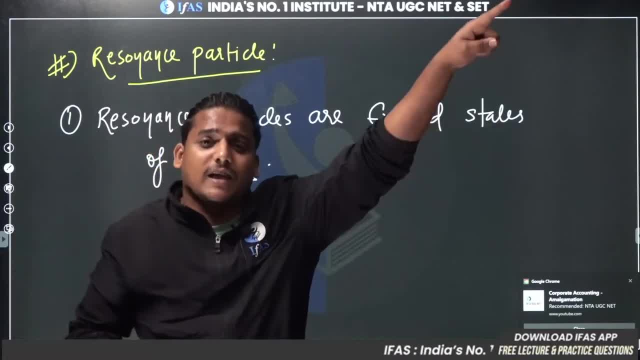 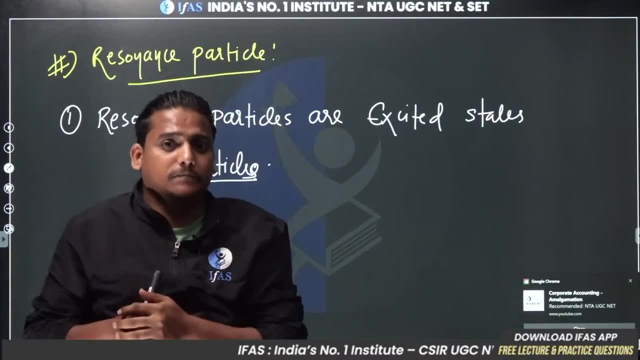 evidence of this? Because their excited state is existing. resonance particles are existing. and what is the second evidence of this? I will tell you when I will teach you quark. if someone asks you that the neutron is because we cannot see it, it is a proton. we cannot see it. what is its evidence that the neutron? 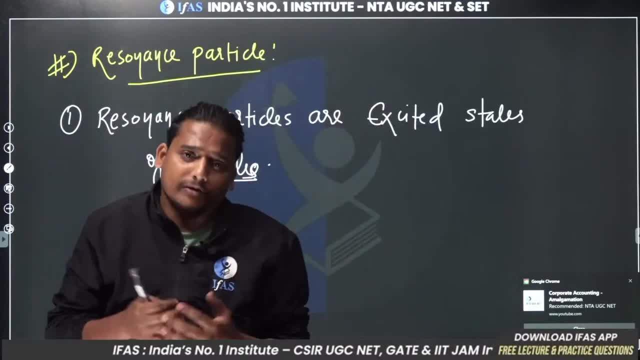 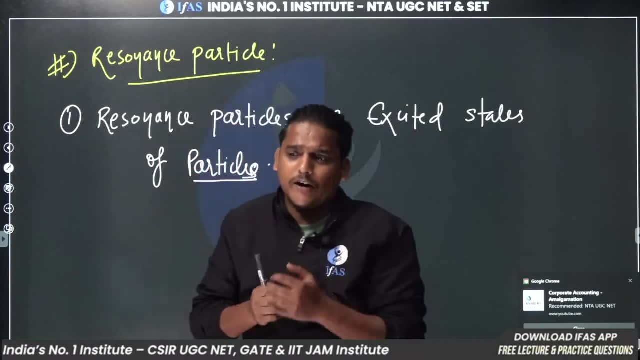 is a proton. it is made up of quarks. someone can ask you. it is an important question. if someone asks you, then what is the answer to you? as its evidence, first of all, what I just told you. secondly, you have to tell you that the length of the neutron is equal. 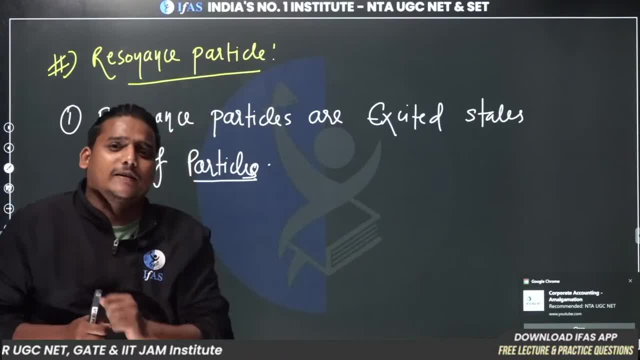 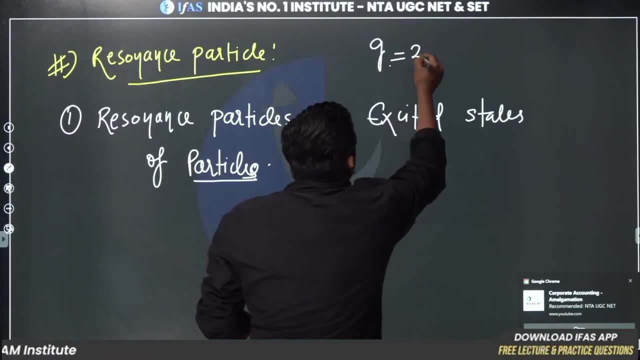 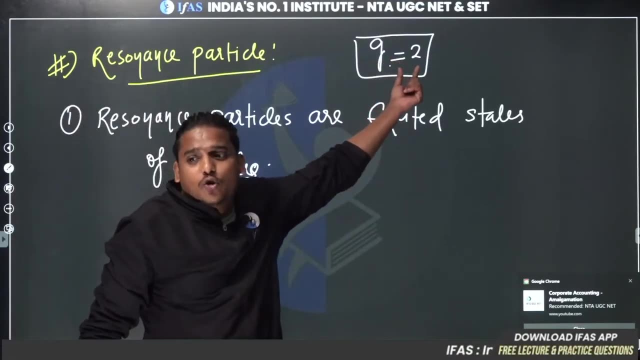 to the length of the quark. the length of the neutron is equal to the length of the quark, ie any particle in the neutron particle can have a decide only in one, or often in one case. because of which, friends in a neutronRIS? Na, there are two factors that giving the information. 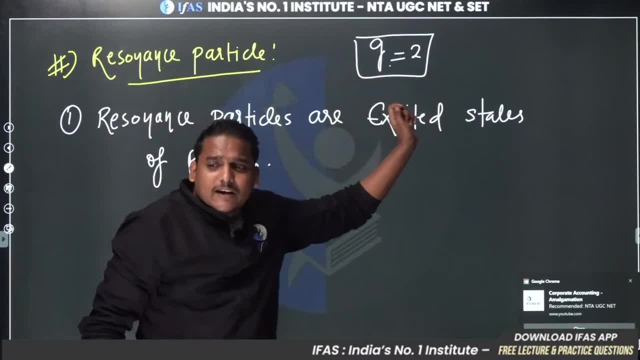 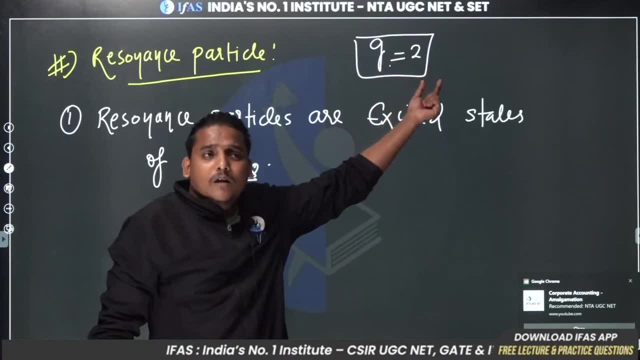 to this neutron n. the first one is the free - that is, the first is the packed part, And the third is fahily satureless particles. Okay, Here you can see. for neutrons and protons, the value of the Landry G factor is 2.. 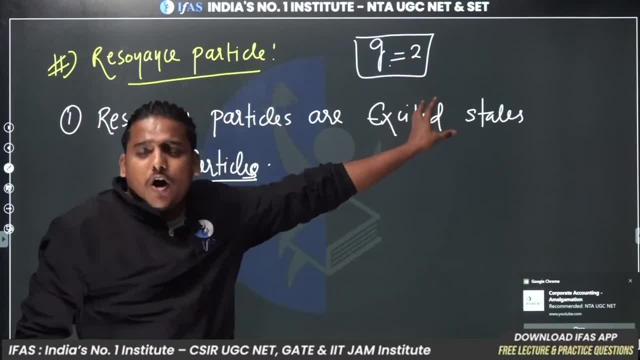 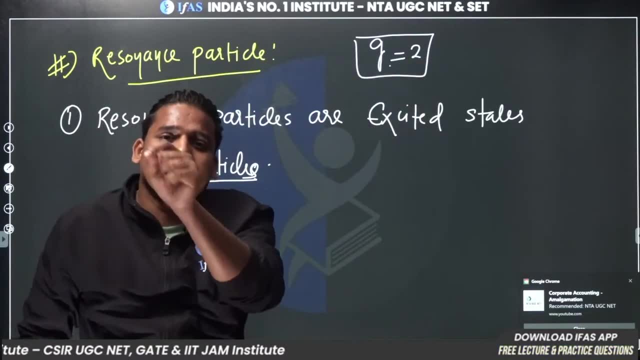 But if you look at the cork model, I will tell you that for protons and neutrons, the value of the Landry G factor is less than 2.. So this is the evidence that the internal structure of protons and neutrons is existing. 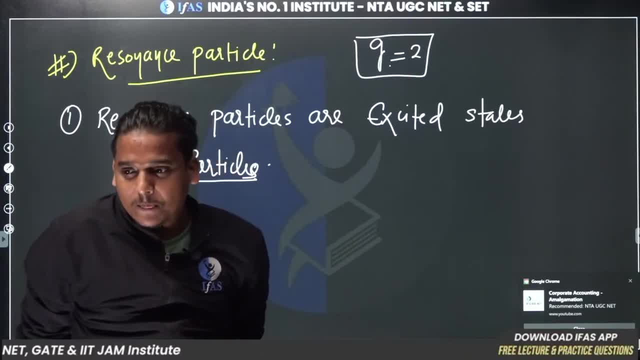 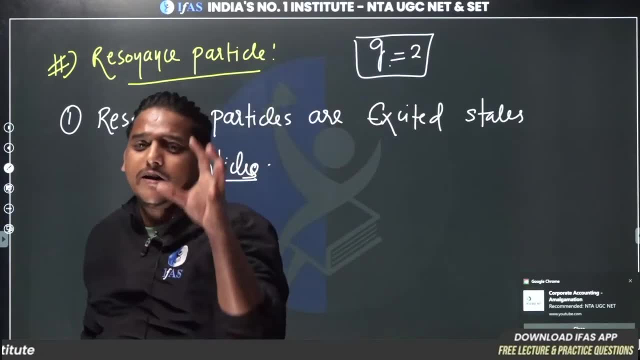 it is not a structure-less particle. Did you feel this? Did you feel this? Tell us in the comment section. The Landry G factor is giving us an evidence that the internal structure of protons and neutrons is not a structure-less particle. 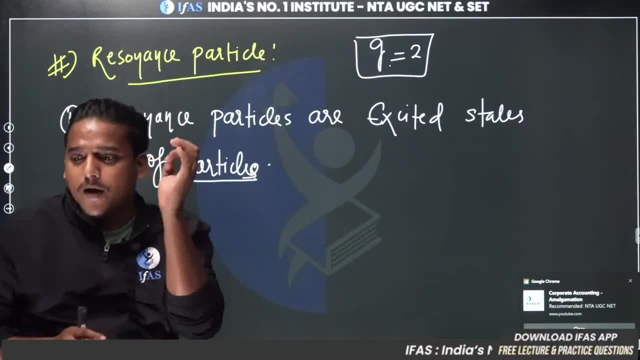 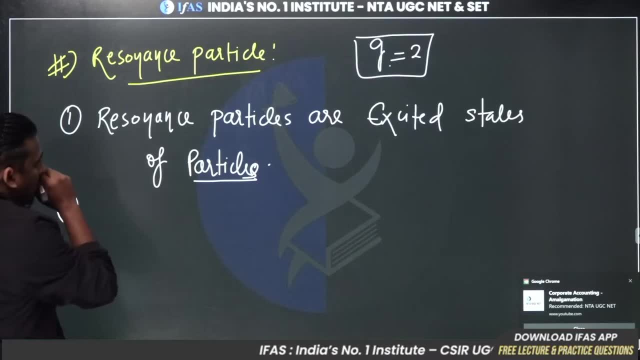 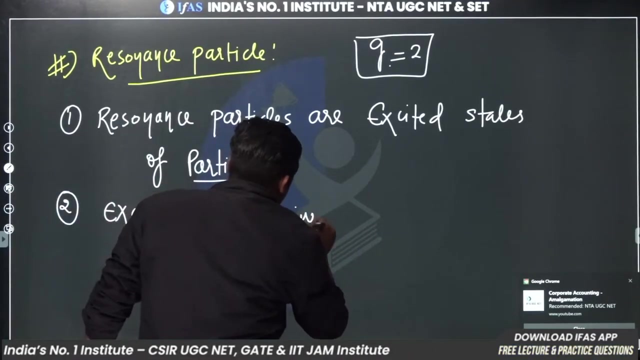 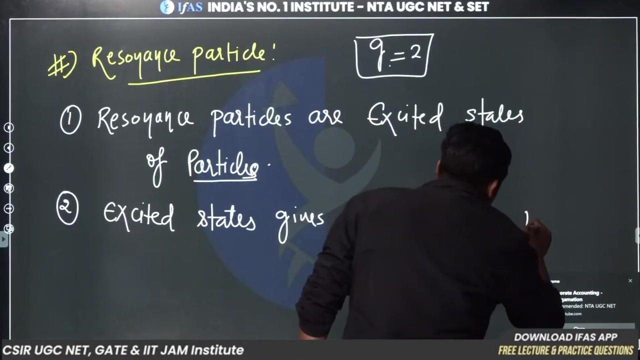 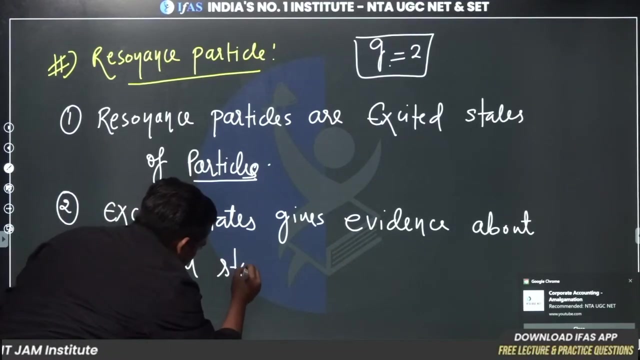 Don't many students know this. I hope you understood it now, So write it here. Write it here. Resonance- excited states- gives evidence about internal structures of nucleons. The internal structure of nucleons is giving evidence about excited states and resonance particles. 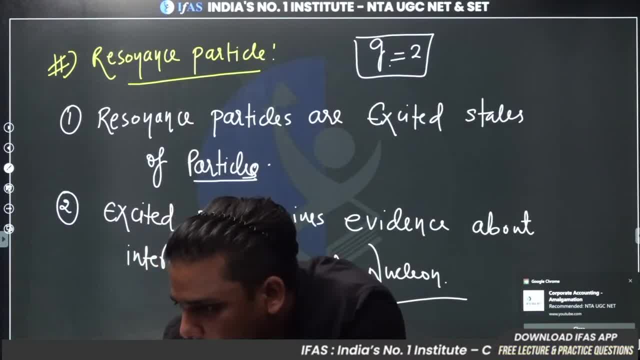 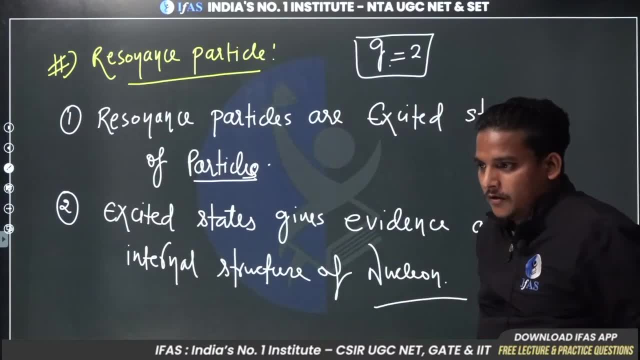 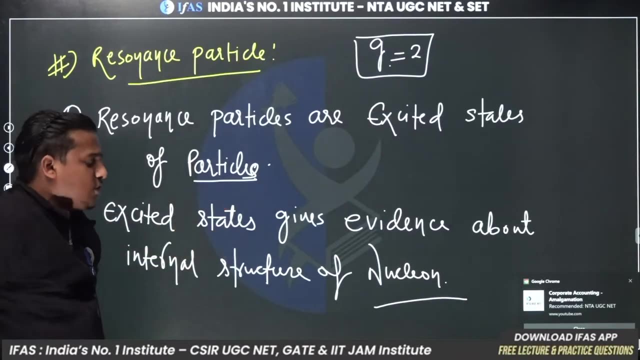 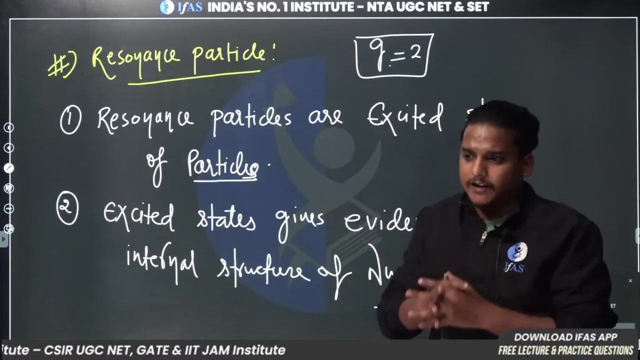 Print this and then we will move forward. If everything is clear, then like and share the session. Thank you very much. Now see how much information we have covered in this one hour session, Sir side, Sorry, Sorry, Forgive me. 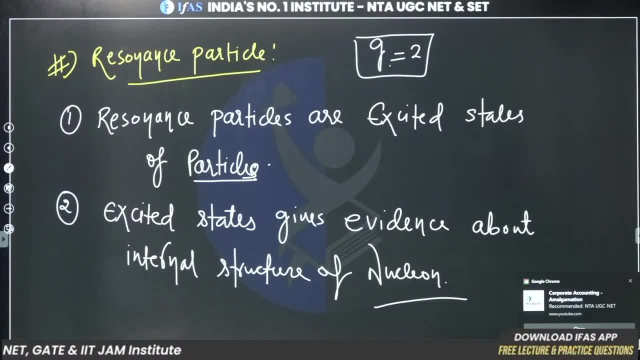 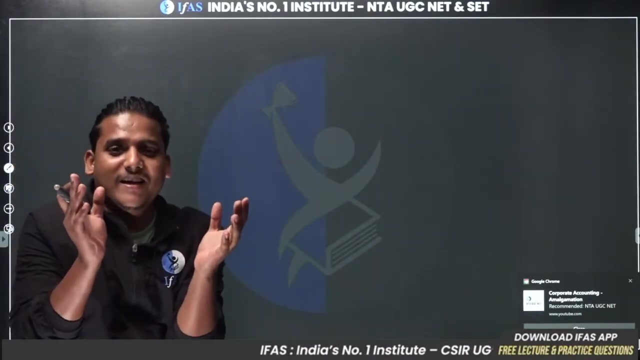 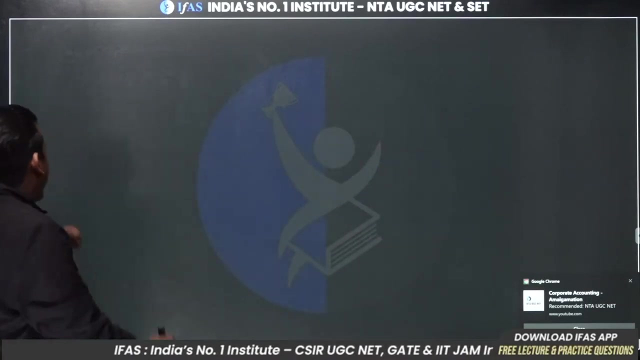 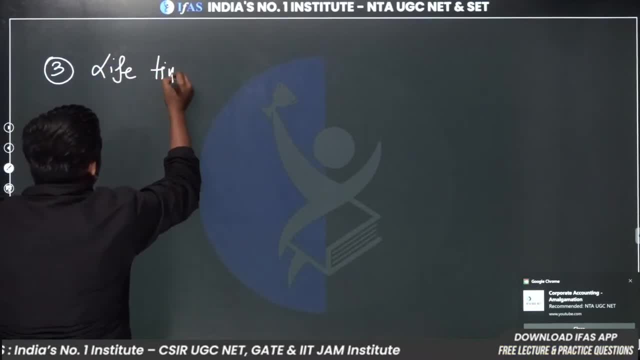 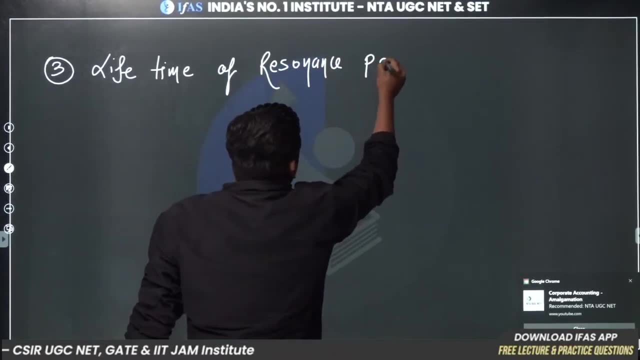 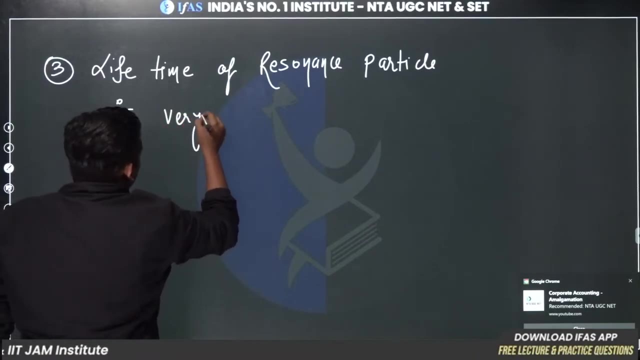 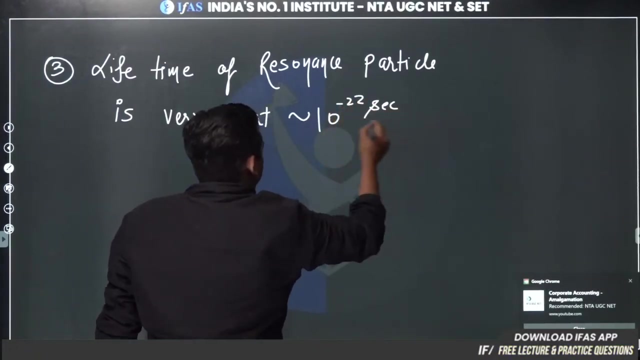 is very short. life time of resonance particle is very short. you can say approx. 10 to power minus 22 seconds. something like this, 23,. something like this, see, means they exist for very less time. their life time is very less. this is the 3rd point. so 3rd point. 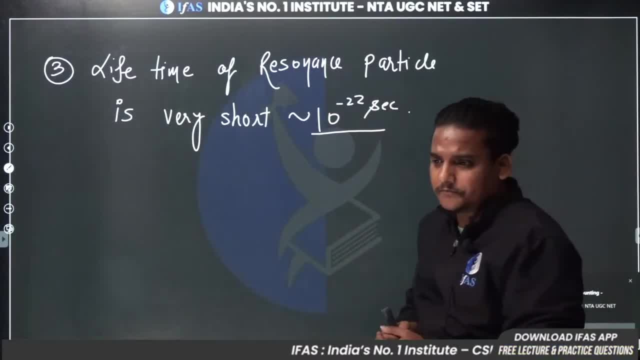 add more 10 to power, 22 or 23,, whatever it is. see they are telling 23,. ok, if it is 23,, then it is 23,. yes, then there is not much difference in it. no problem, come on. 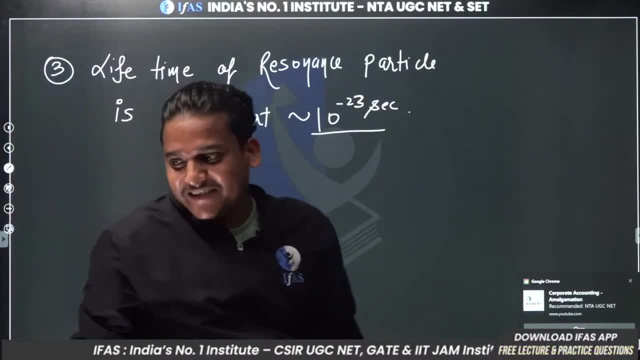 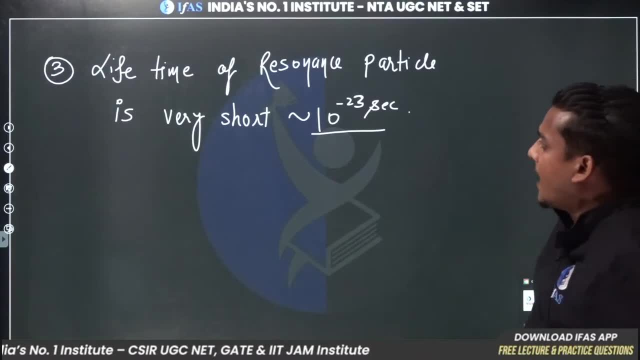 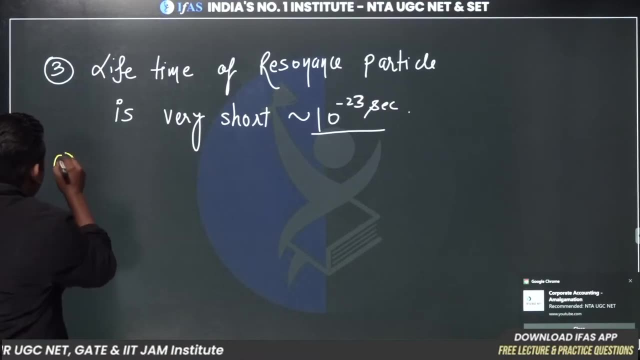 you said as you said, so write clear. now let's discuss which are the resonance particles. which are the resonance particles that exist with us. first is Rho meson. ok, Rho meson, which is Rho meson, whose excited state is Rho meson. I said the excited state of resonance. 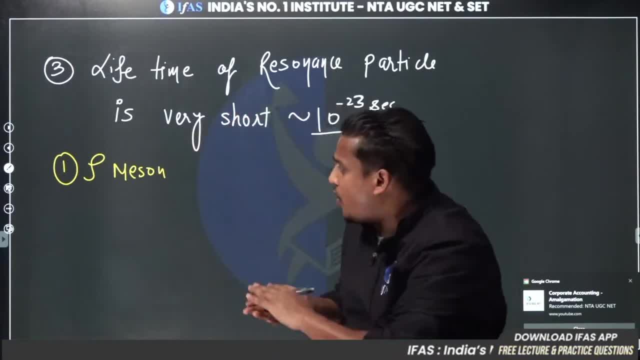 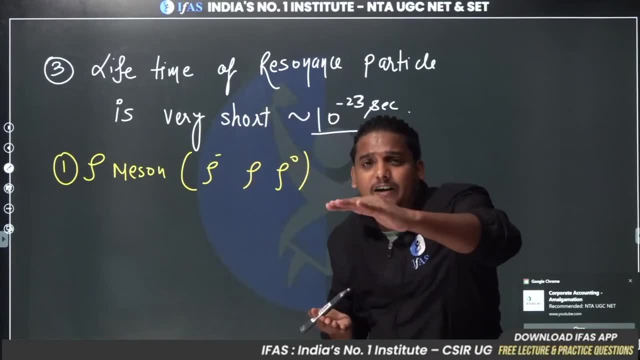 particles, which is the excited state of some known particles. so, Rho meson, which is your 3 particles, Rho minus Rho, Rho, zero, whatever it is. whose excited state is this? it can be asked to you? it is the excited state of pions. very good, very good, perfect Avrupa. 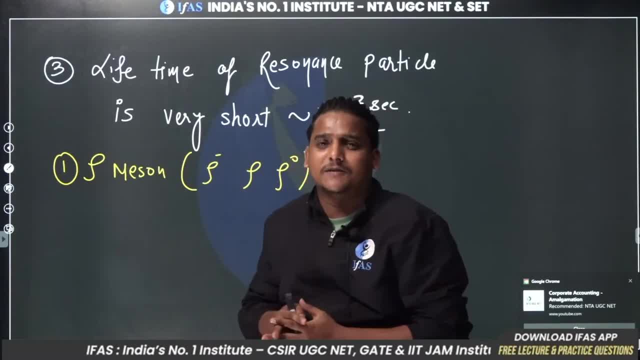 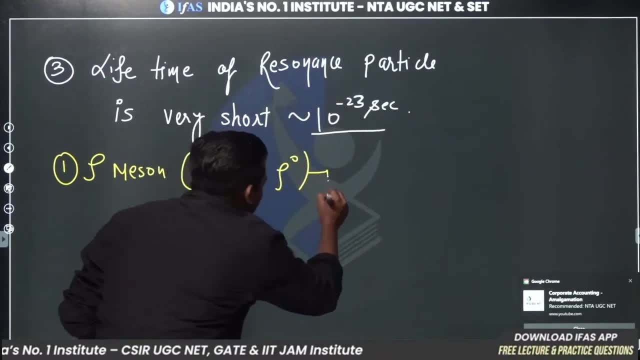 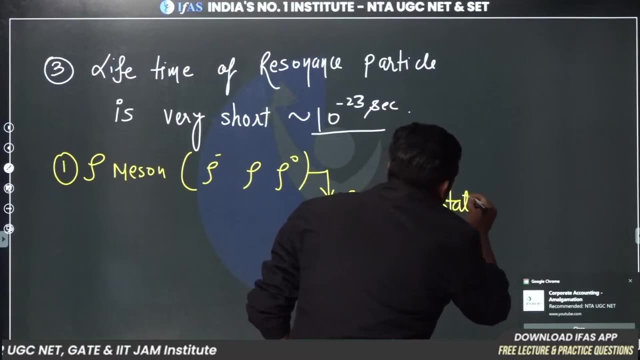 Chaturpad. very good, children, you answer all the questions, I like it. Rho meson, Rho mesons are the excited states of pions. so write here that this is the excited state of pions. perfect, very good, well done, keep printing. one important information, second. 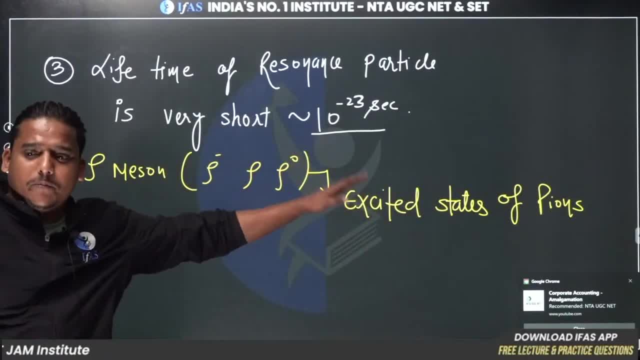 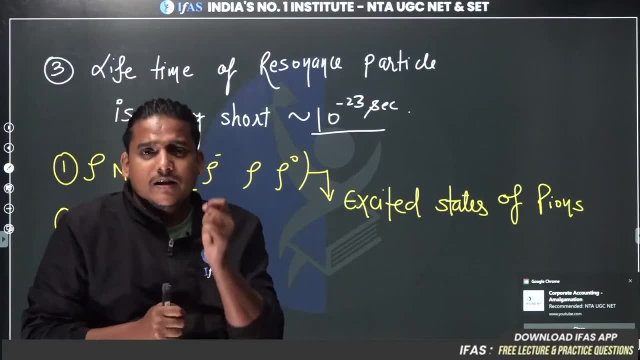 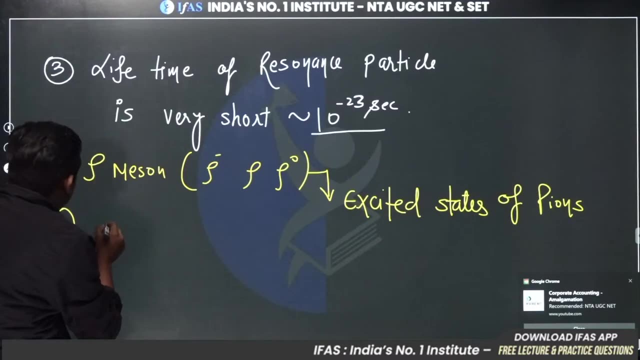 we have delta, delta baryons. ok, the second resonance particle is called delta baryons. here you can write it. you can write it like this. write it like this: in delta baryons you have 4 types of particles: which particles from which particles? delta double plus and. 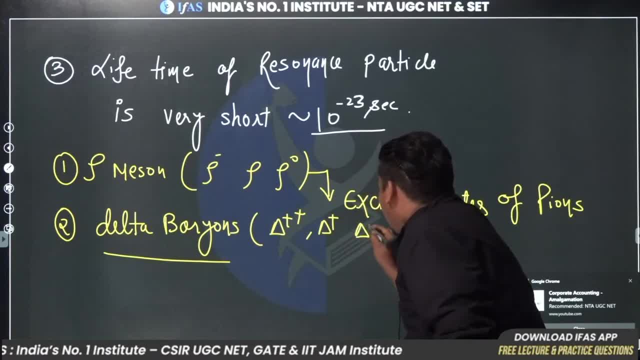 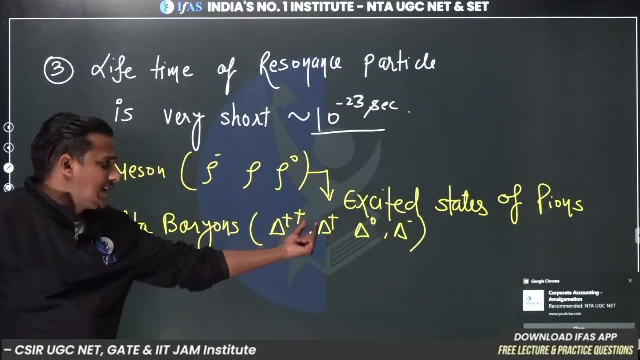 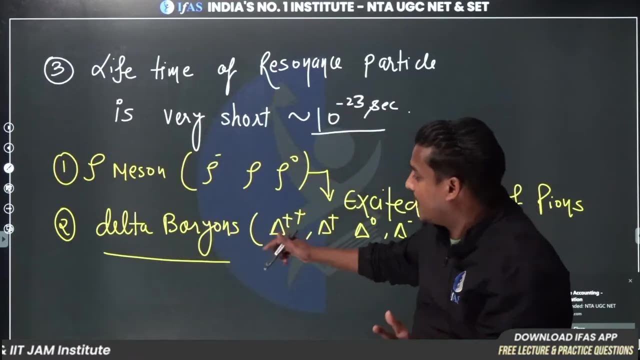 delta plus, delta zero, I think, delta minus. this is the four particles we have: delta baryons, delta plus plus, delta plus delta zero, delta minus, and these are the excited states of what. These are the excited states of in this also, I will. 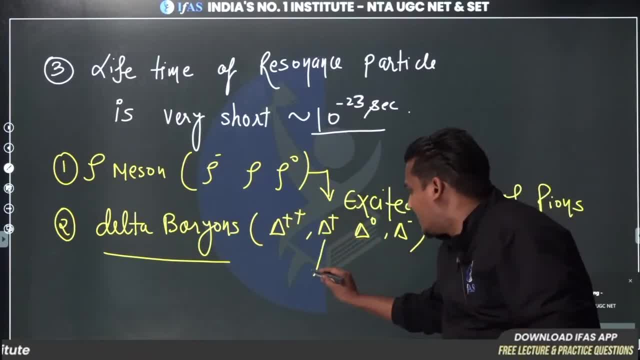 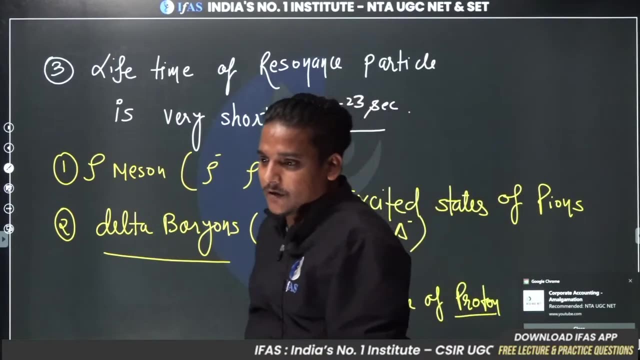 tell you individually: Delta plus. here the excited states are of proton. Okay, Delta plus is the excited state of proton. Write it down: Excited state. Important information. Sir, today we are not able to attend the class because of network issue. No problem, Switch it. 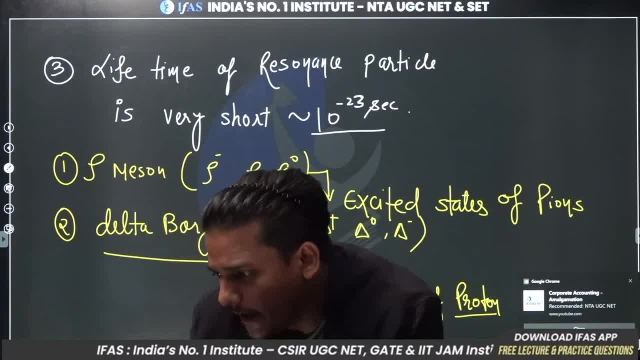 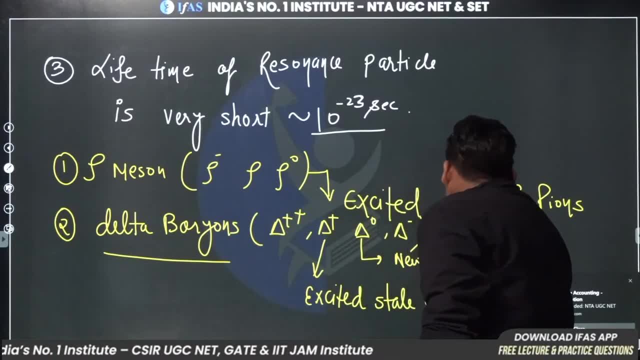 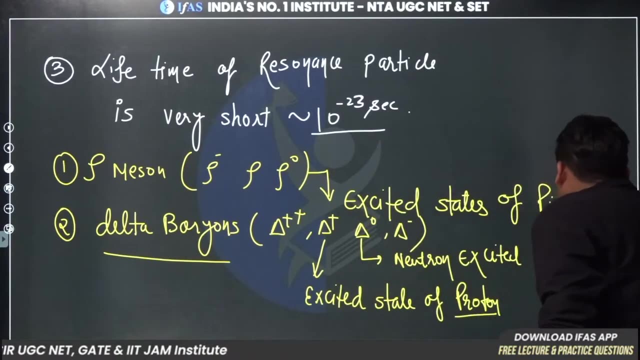 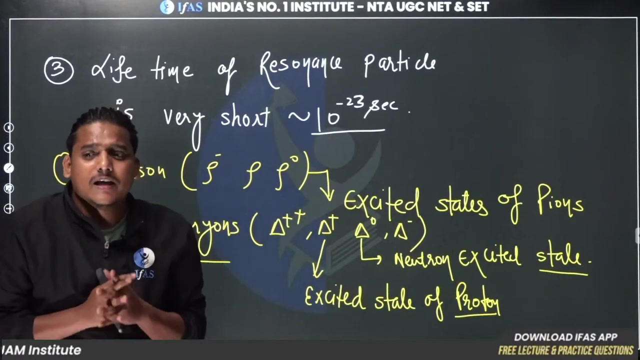 See it later. See it later, No problem. And delta zero is the excited state of neutron. Move aside. So you must have felt the resonance particle. Actually, it must have been clear in your mind that what is the resonance particle? What information? 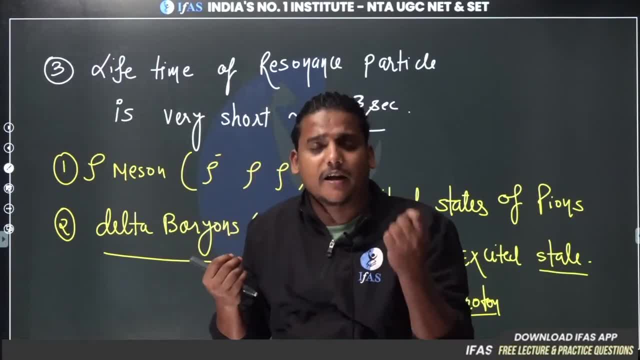 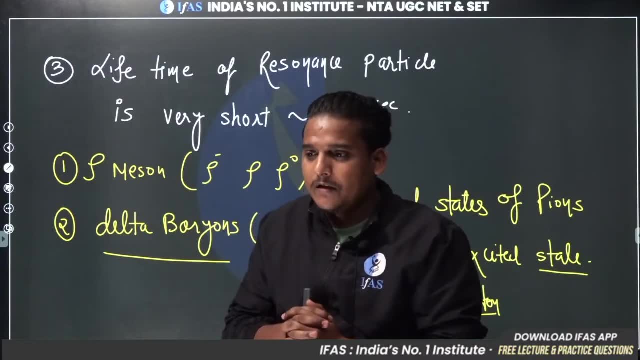 is it giving us, And who are they And whose excited state is it? I hope you must have enjoyed it. Is it clear? Quickly comment on it. Tell me in the comment section: Is the resonance particle's feel clear? Yes, sir, 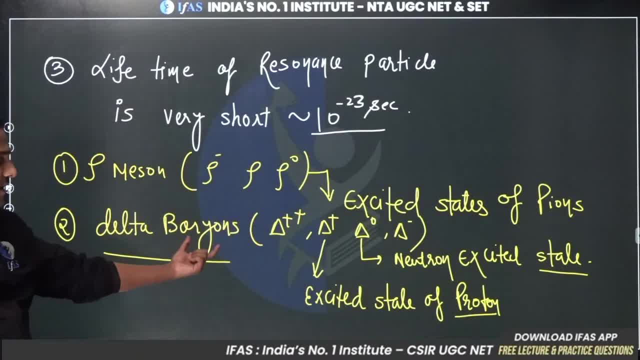 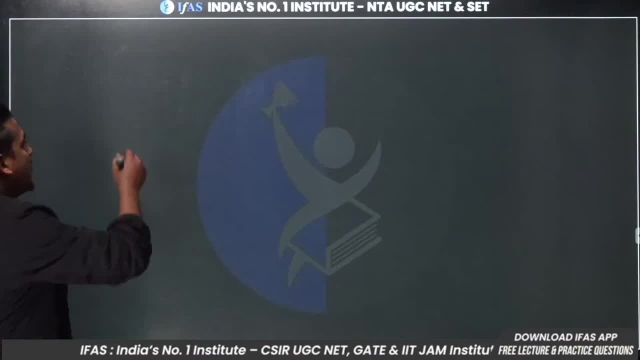 Now let's talk about it. Now let's try to find out its iso spin Delta variance. If you find out the iso spin of delta variance, then what is the multiplicity of delta variance? It is 4.. So 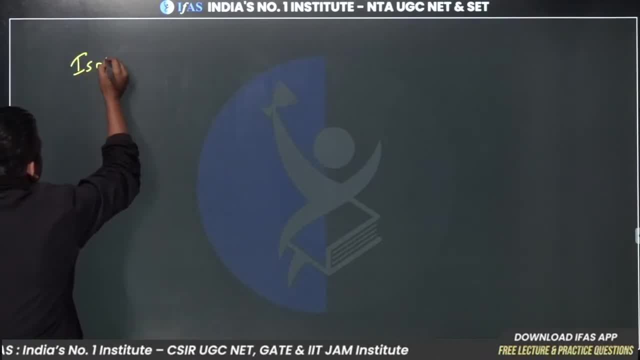 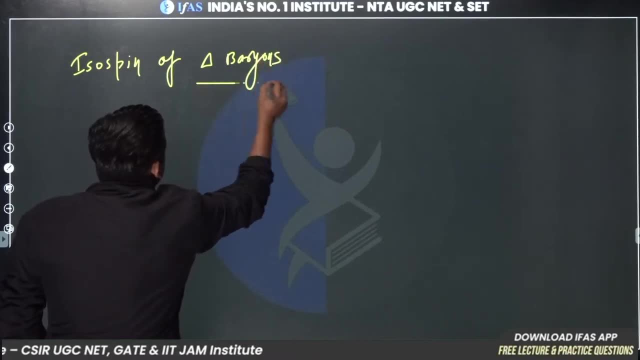 write here Iso spin of delta variance. So if I find out its iso spin, then 2i plus 1. is equal to 4.. 2i plus 1 is equal to 4.. So from here, what will be my i? 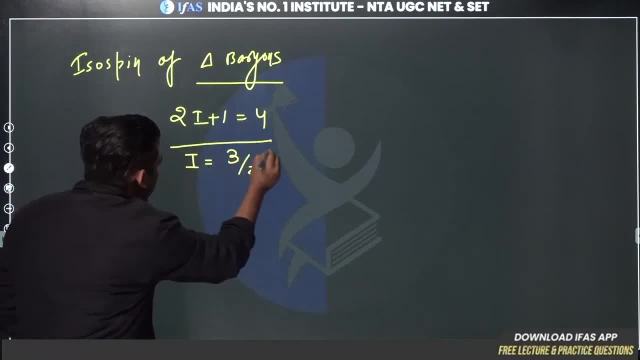 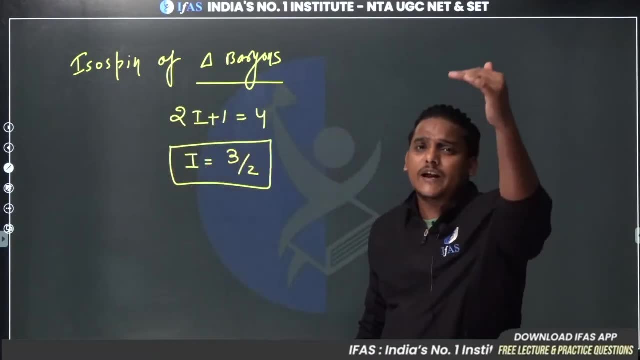 1 out of 4 is 3.. 3 divided by 2.. So its iso spin comes. It comes 3 divided by 2.. So if we find out its third component, then how much will it be Minus 3 by 2 to 3 by 2 in the units of 1.. 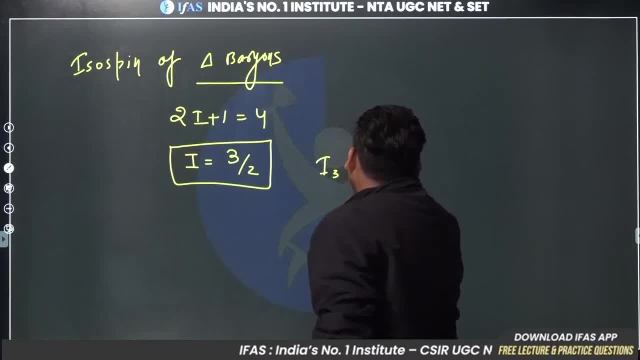 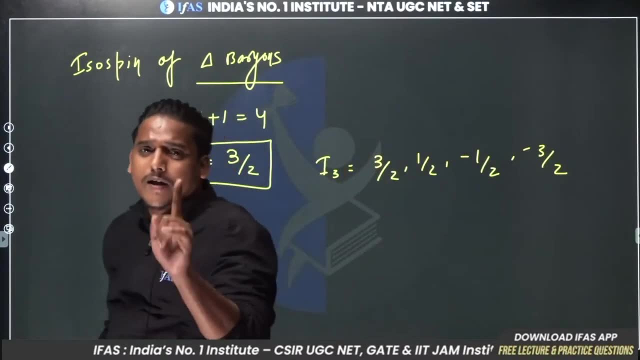 So here, what will be the values of i3?? What will happen here? 3 by 2, 1 by 2, minus 1 by 2, minus 3 by 2.. Is it shining? Is it shining or not? 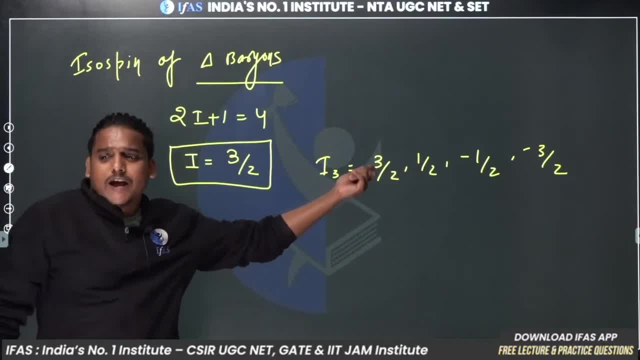 Tell me in the comment section and keep liking the session. The values of i3 will be from 3 by 2 to minus 3 by 2 in units of 1.. 3 by 2, 1 by 2, minus 1 by 2, minus 3 by 2 in the difference of 1.. 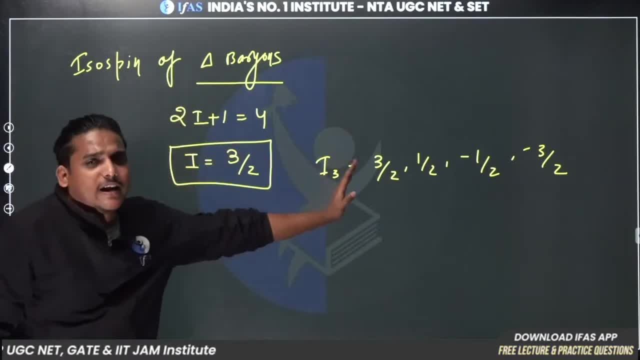 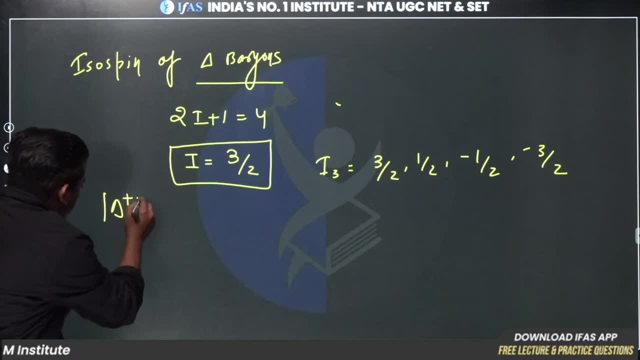 Right, Very good. So now which i3 value will go to which corresponding- This is very important for you- Which i3 will go to which States are written. So delta plus plus. The state of delta plus plus will be 3 by 2 comma, 3 by 2.. 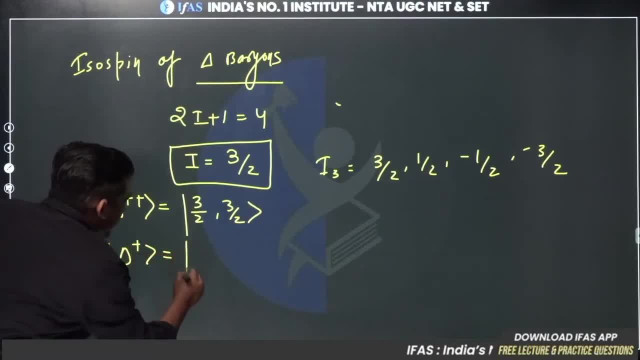 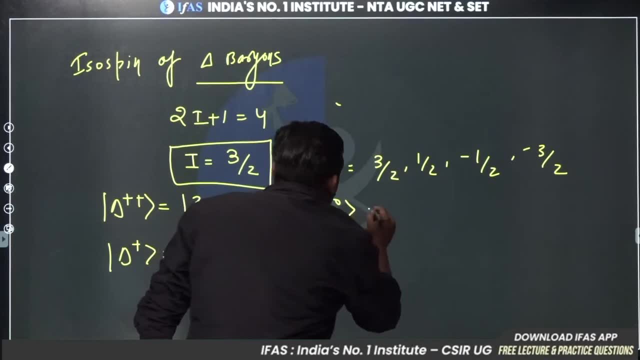 Right, And the state of delta plus will be 3 by 2 comma, 3 by 2.. And write here: the state of delta zero will be 3 by 2 minus 1 by 2.. And the state of delta minus will be 3 by 2 minus 3 by 2.. 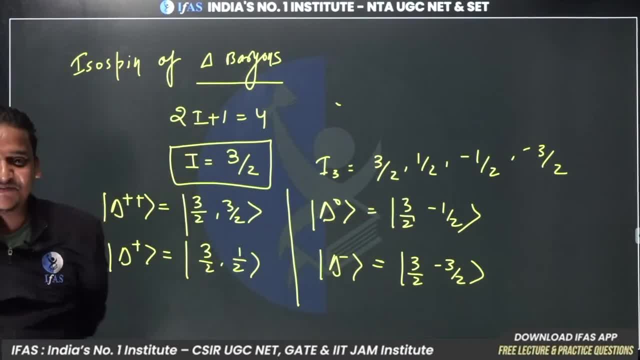 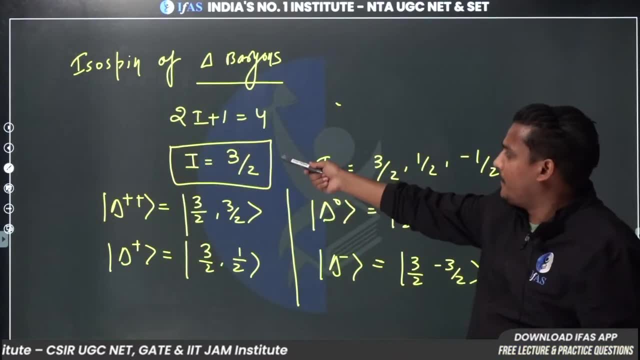 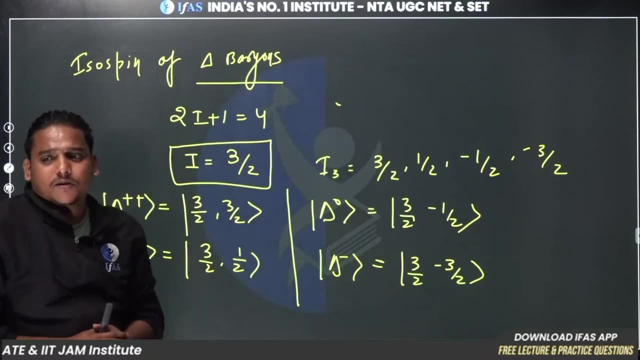 This is the thing, And today's lecture is on here. Is it clear? We took delta's isosceles, delta variance's i3 and defined its states. If any problem arises in this, Any problem, Any doubt, Tell us in the comment section. 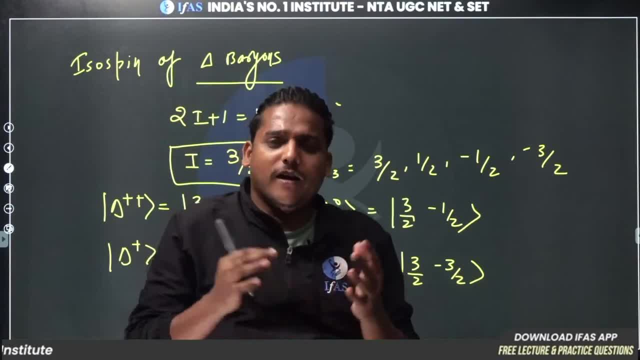 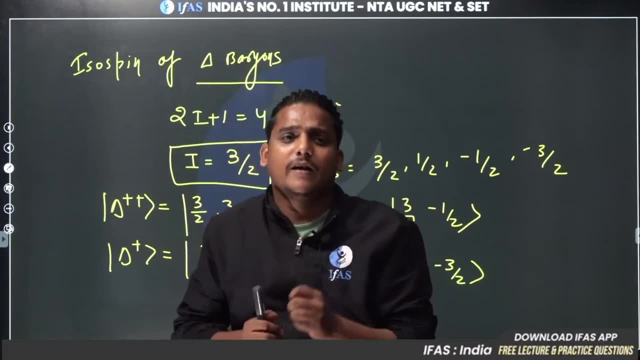 So this was our today's lecture. Today we talked about baryonic number, We talked about the leptonic number. We understood the important points of isospin. What is the need of isospin? How will it play a role in numericals? 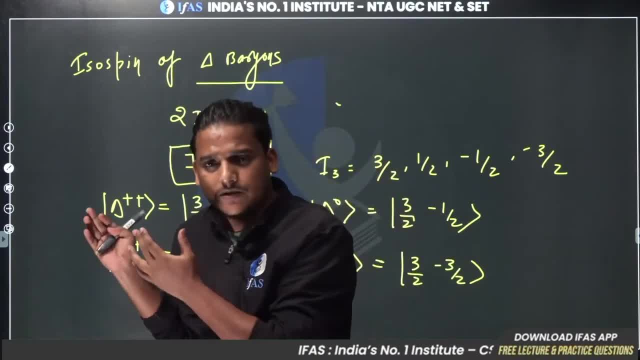 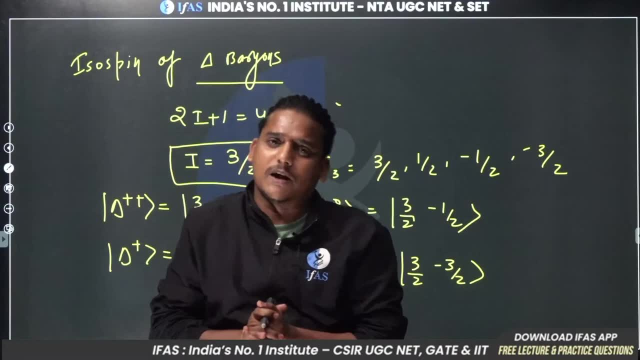 We discussed about that And in the last we understood a very important concept of resonance particle. Is it clear? I hope you have noted all the things. Tell me in the comment section. How did you like the information of today's lecture? 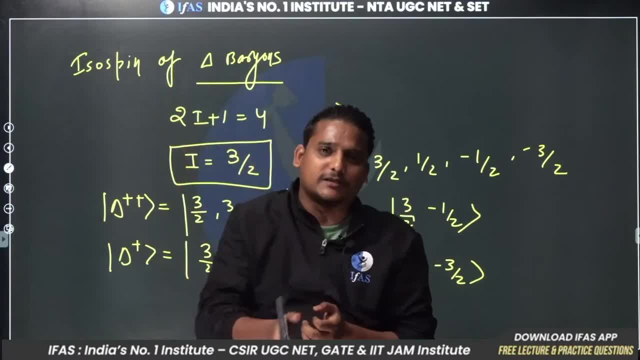 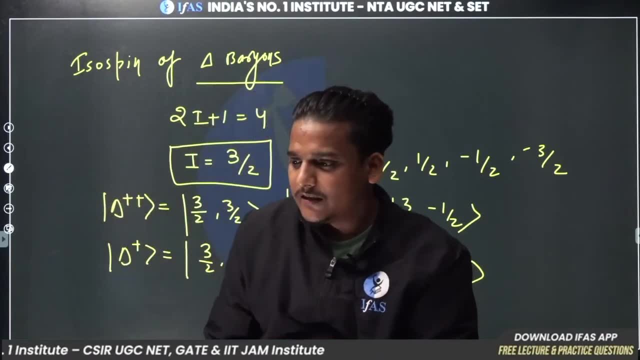 How did you understand? All the things are clear. I want to know in the comment section. I want to know quickly about the comments. Tell me if there is any lack in the lecture And tell me how you felt. I want to know about the comments.